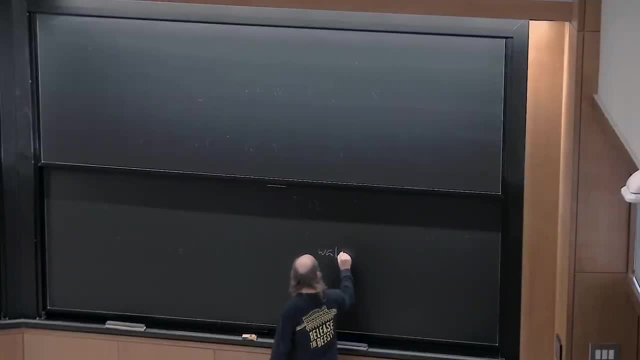 look at a website which I can recommend. It's called WALLS. Oh dear, I was about to write the URL and then I realized- I don't know how, If you Google WALLS, WALLS stands for the World Atlas of Language Structures, and I think it's something done like wallscom or something like. 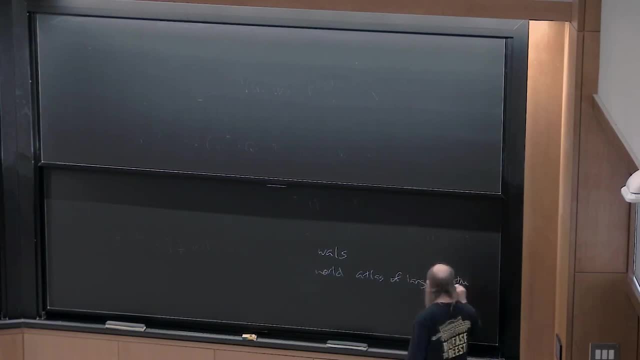 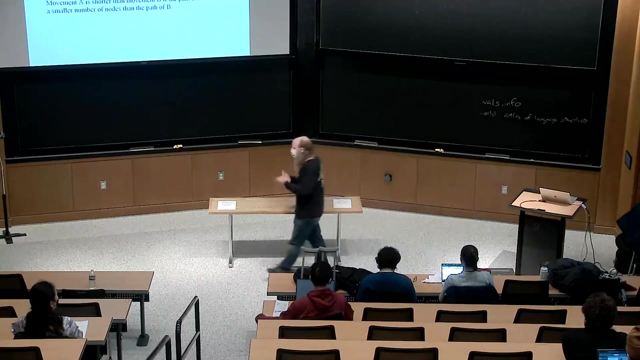 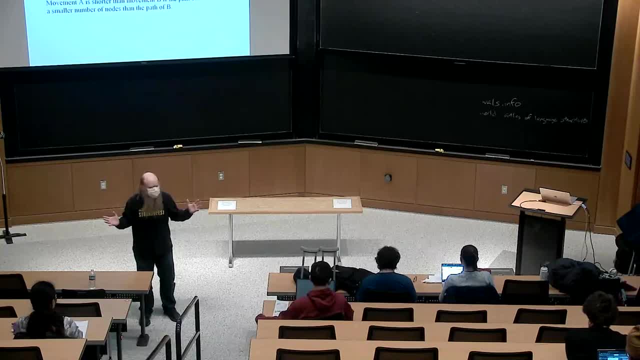 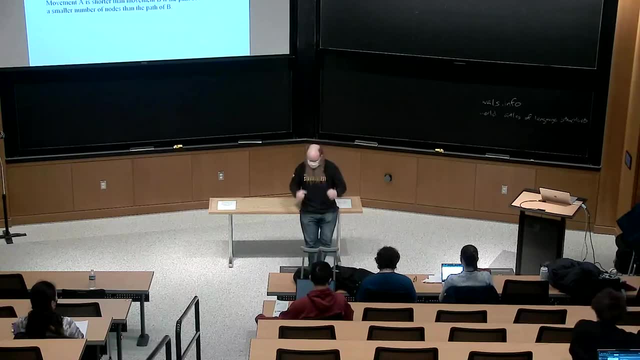 it has, I don't know, thousands of languages, observations by various linguists who work on them, categorized by various phenomena. So there are all these parameters that you can look up. You can, you know, find out how many of these languages have the verb before the object, how. 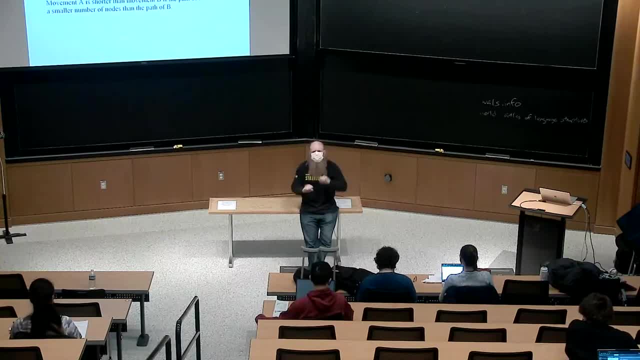 many of them have the object before the verb. You can get it to make you a map of you know where these languages are and all that cute stuff. And they take a stab at having a typologically balanced, genealogically balanced survey, I guess. So the languages are not all Indo-European, They're. 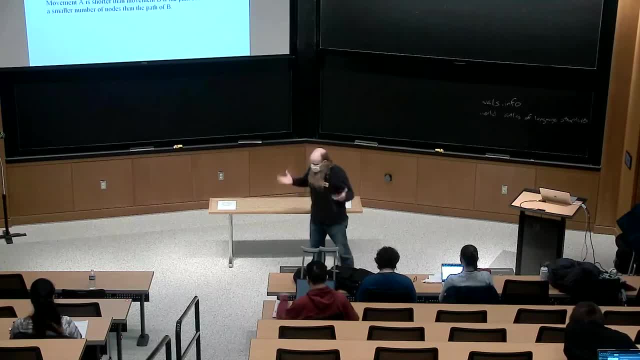 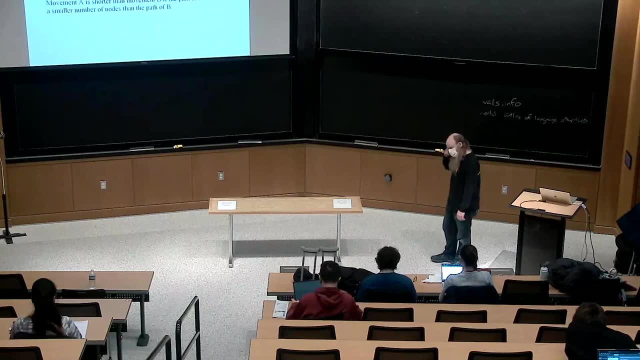 the world. There's all kinds of stuff there, Some of the generalizations that I was showing you. it's trivial to show that they are statistically significant. So for example, there are, according to WALLS, roughly a third of the world's languages have WH movement to the left, That is, they're. 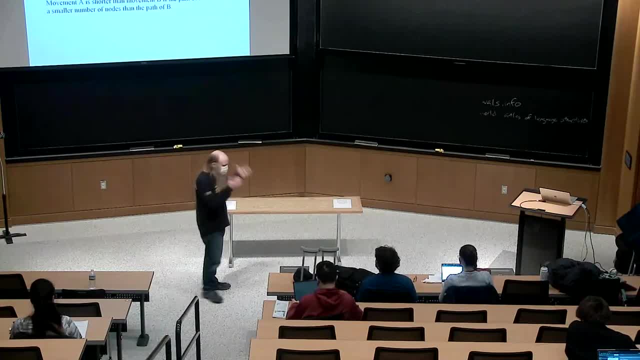 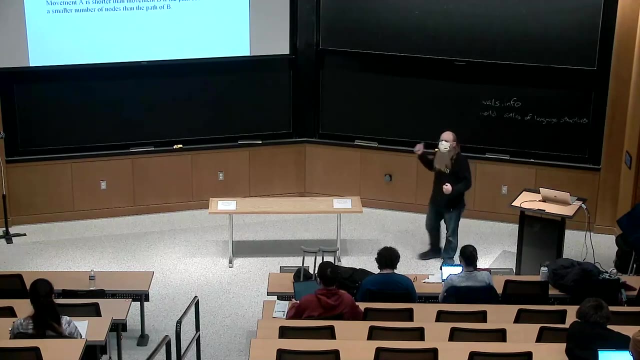 like English, And the other two-thirds have WH in situ. So if that is, WH goes wherever the WH would normally go, it doesn't move. So when I told you that there is WH movement to the left and there isn't WH movement to the right, you know I'm not a mathematician, but that looks statistically. 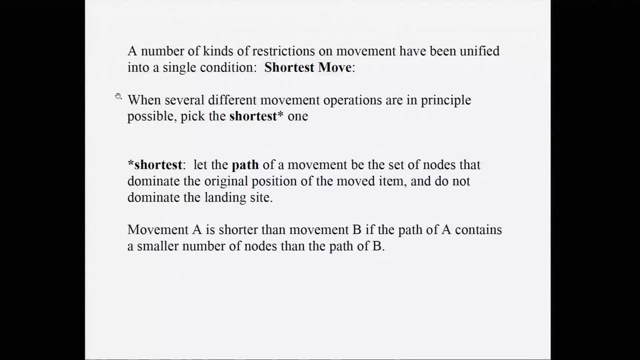 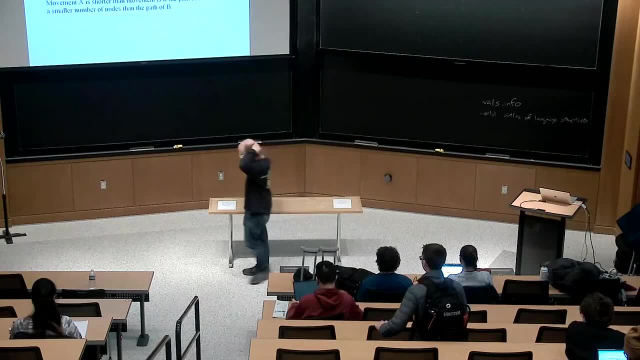 significant, given that they're studying thousands and thousands of languages. It's, it's surprising, you know, if you thought that WH movement to the right was, should be, just as common as WH movement to the left. the absence of that in any of the languages we've studied is is surprising. 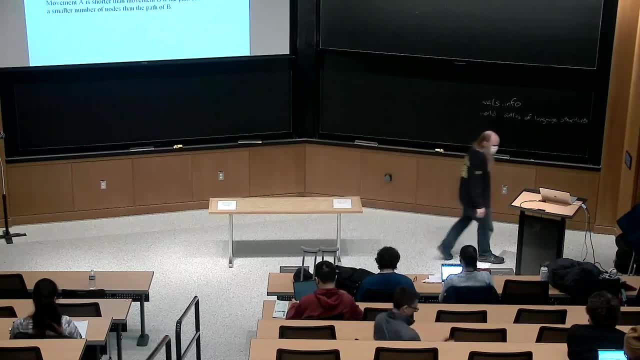 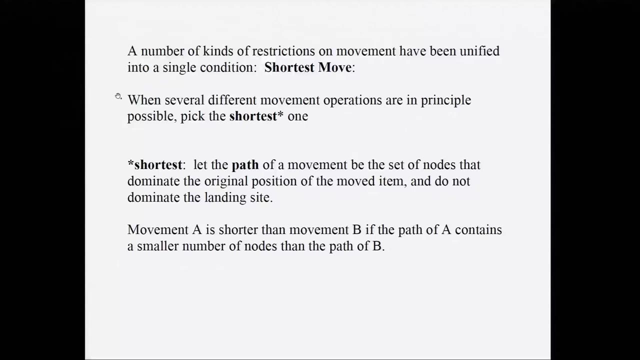 and significant, But, as I say I'll, I'll write up some stats and send them to you. Questions about that or anything else that we did last time? Okay, So this, as I said, we had gotten started on this and I'll just back up and go through this again. We were talking last time about 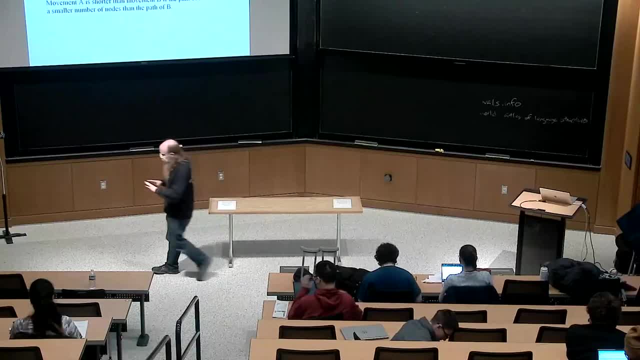 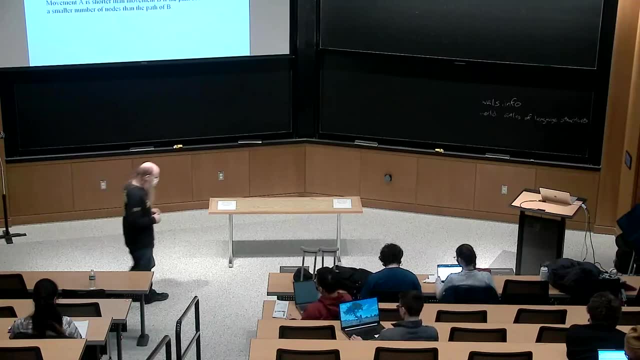 restrictions on movement. So I've given you the beginnings of some reasons to believe that there are cases where forming a tree for a sentence, forming a syntactic structure, isn't just a matter of merging things to each other, but that sometimes you take something which has already been merged. 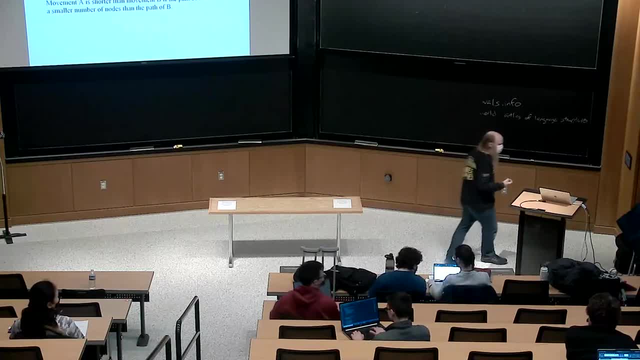 and you move it someplace else. And we've talked about different kinds of movement And last time, towards the end of last time, I was starting to show you examples of kinds of movement that you couldn't do. So you know. 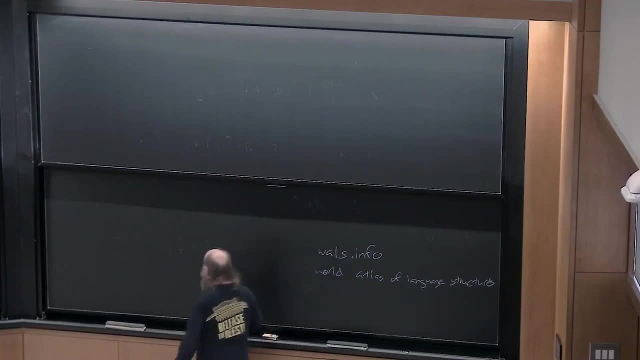 I think one of the examples we talked about. you know you can say things like she ordered a hamburger and fries, but that if you were to take fries, replace it with a WH phrase and try to WH move it, giving you what did she order? 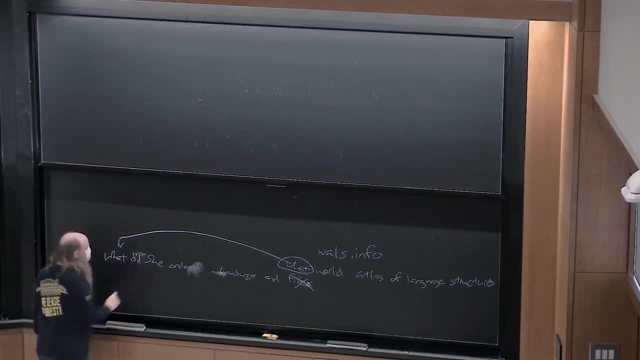 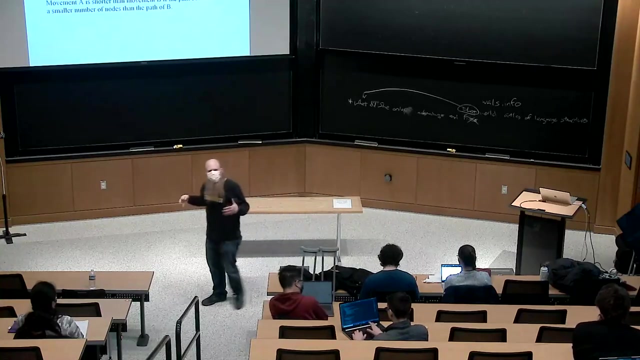 a hamburger. and even if you spell did correctly- which is surprisingly challenging- the result is very bad. So I showed you some examples like that, where if you arrange to put a WH phrase in a certain kind of structure, it somehow can't escape. We're calling those structures islands. 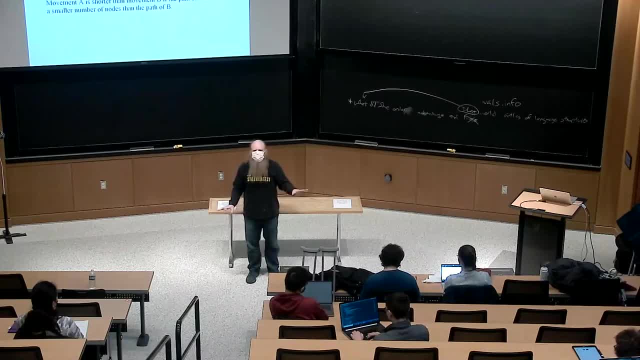 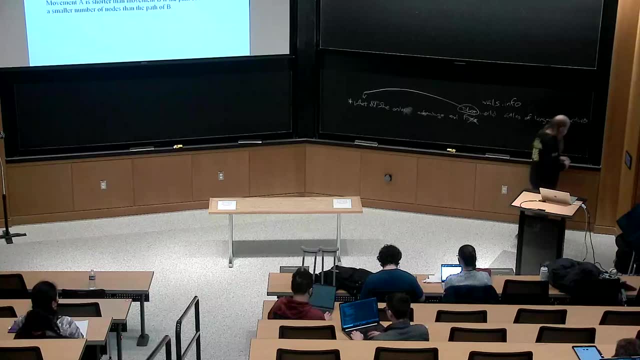 There's some kinds of WH movement that you just can't do. Does this sound familiar at all? We were doing this last time And then I said: you know so? there's big literature on syntax, sort of identifying these islands, and 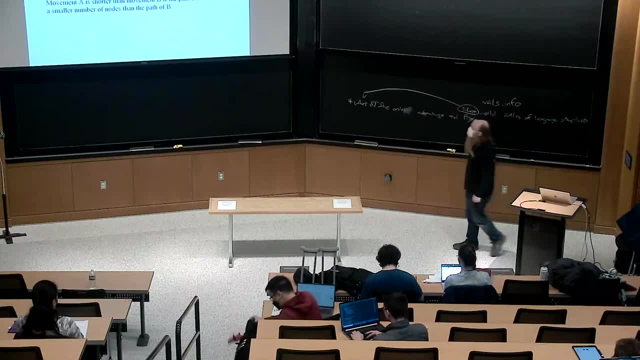 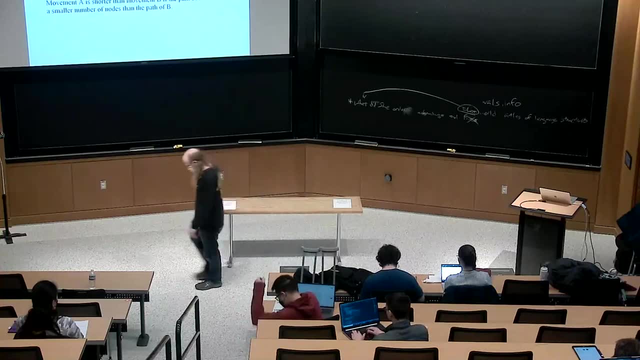 trying to figure out what are the structures that you can't move out of There's actually, and then attempts to develop theories of why certain things are islands, why are certain kinds of things opaque to extraction, And I wanted to show you one theory of one particular set of examples like this: 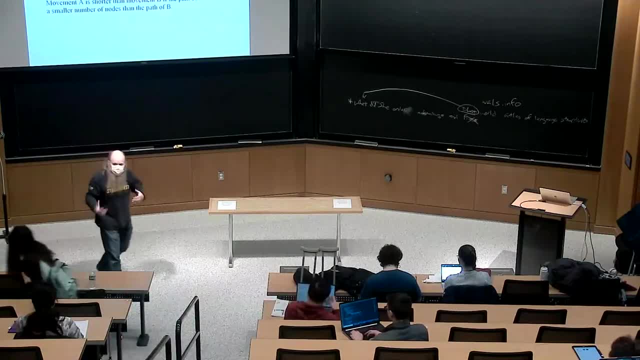 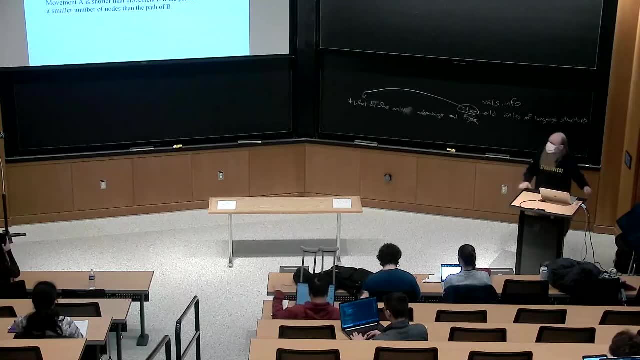 examples of places that you cannot move out of, because, well, the explanation for why these particular things are opaque is, you know, particularly straightforward. So old observation actually, that a number of the restrictions on movement that people have found can be unified into a single. 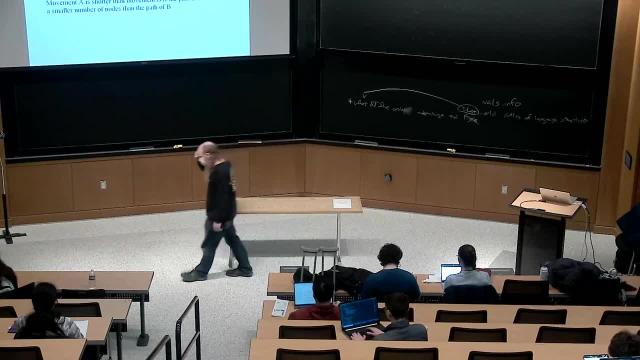 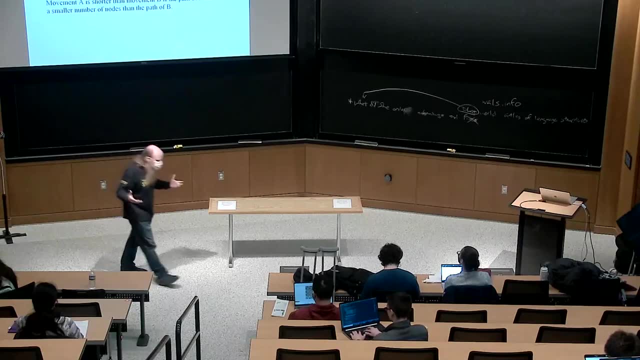 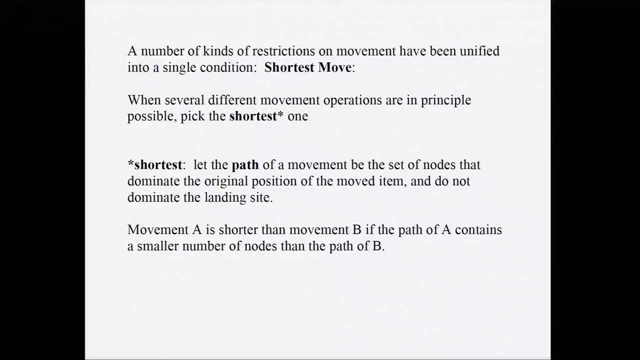 condition that has been called various things and formalized various ways, but today I'll call it shortest move. It says basically, if you have a choice between two movement operations, you should pick the shorter one. So pick short moves over long moves. And I gave you this definition of short. 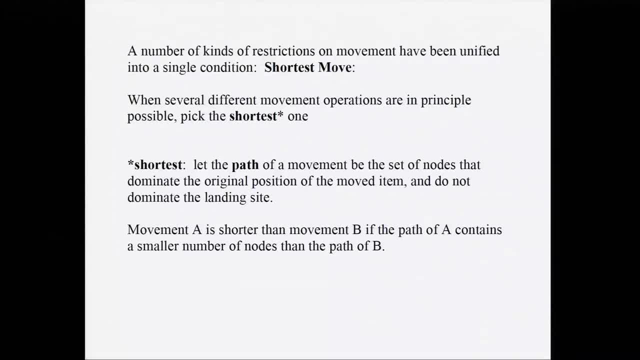 So one of the things people do in this literature is try to figure out exactly how we ought to define short. So one way to define it would be to say one movement is shorter than another movement if it crosses a smaller number of nodes. So you start off dominated by a certain number of nodes, move. 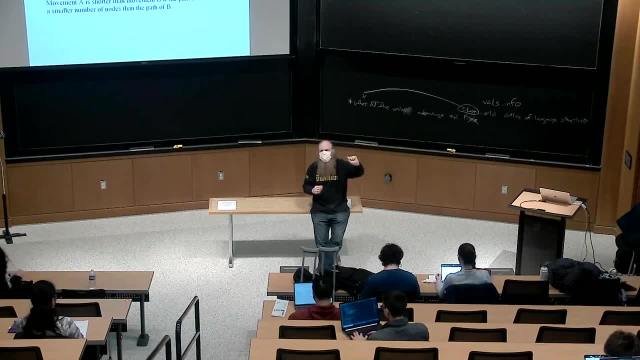 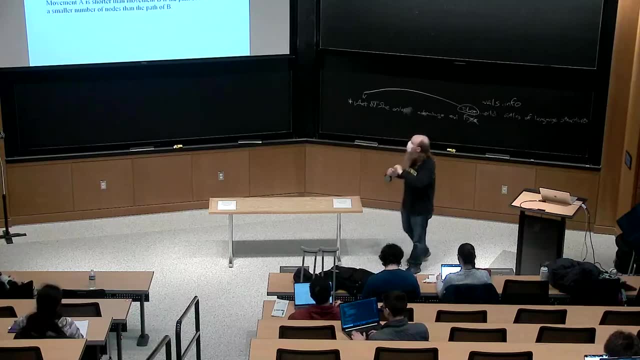 to a position where you are not dominated by some of the nodes. All that means is that if we're saying anakabunga, the path is linked to one given node and you don't Scr museums on which nodes went to and together with other nodes, and they all go together. 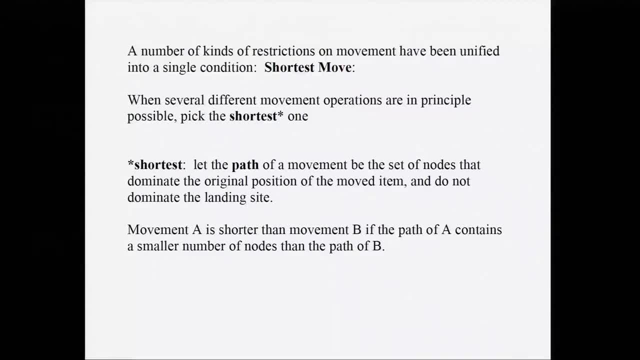 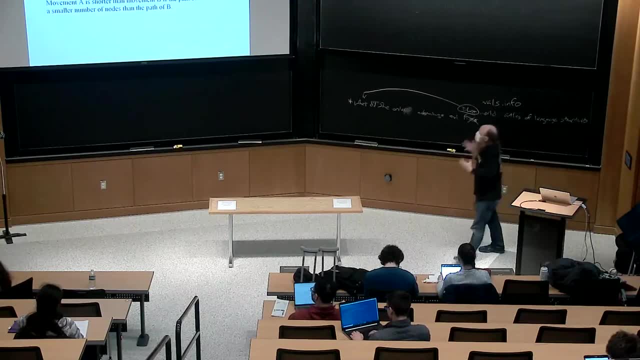 But you say that one move takes one plus one and you say that one move directly. Graci, read the normal way and your path is exactly that same way. What we're saying when you say pluck you Servus. So let's take a look at that. first cue Twomates is identical in extension. you still 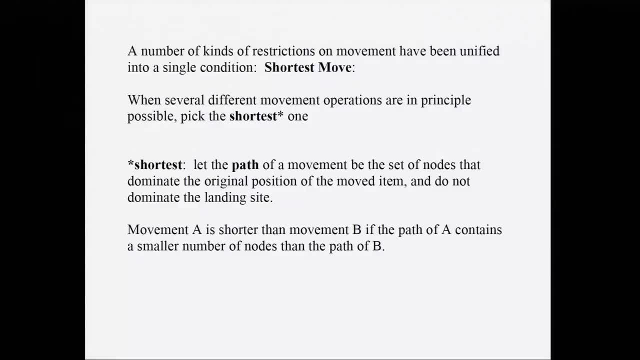 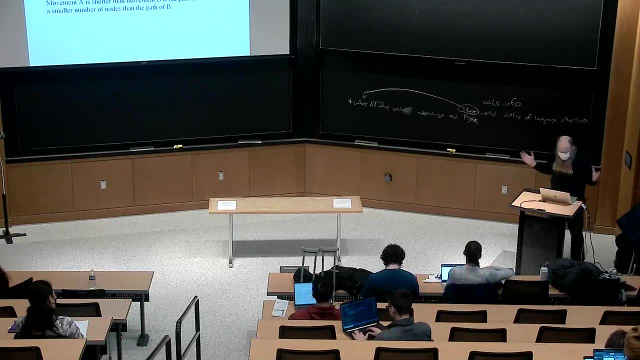 have to Milli of, and then you put in province where the most commonDE님이her- this is point a- then slice in point a, then you put it next one, And then my property limit becomes two. The difference is that have overlapping paths and you are supposed to pick the one that is a. 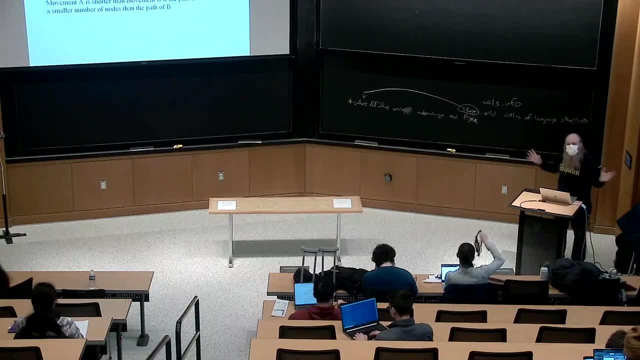 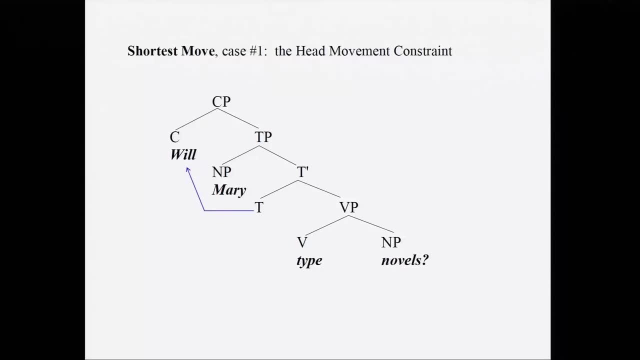 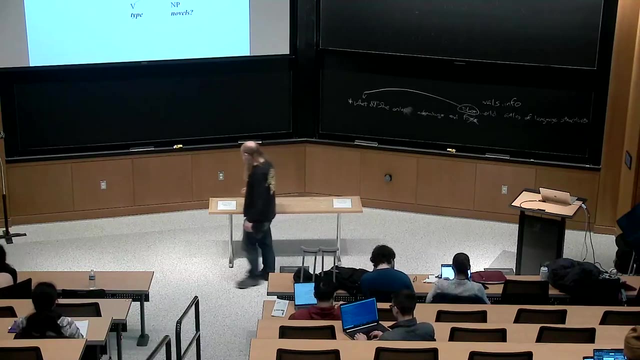 subset path. that's a subset, yeah. so story to tell here, I'll show you some examples. the first example which I showed you last time was the head movement constraint, so you can move heads, but only over very short distances. so English forms: yes-no questions by moving T into C so you can say ask. 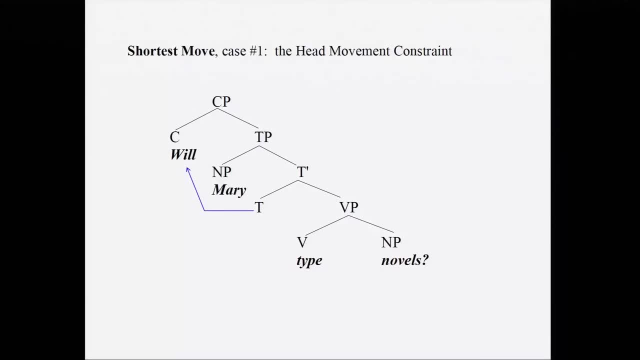 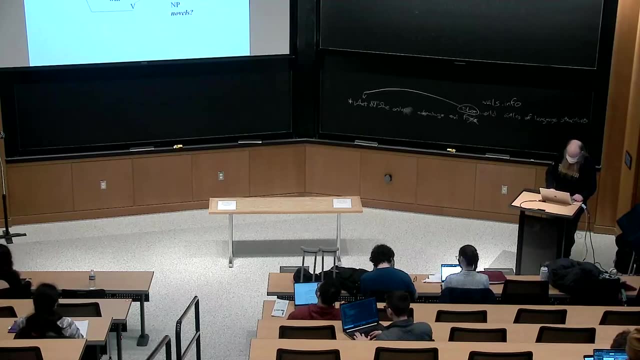 questions like will Mary type novels, where you take what's in T, which is will, and move it into C. that's a way to form that kind of yes-no question. but I said you do not in English or in any language form yes-no questions by moving the verb. 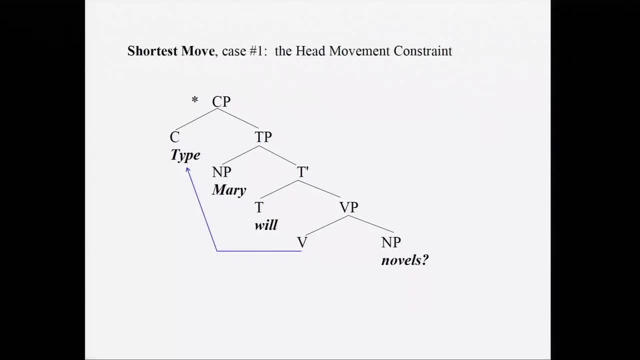 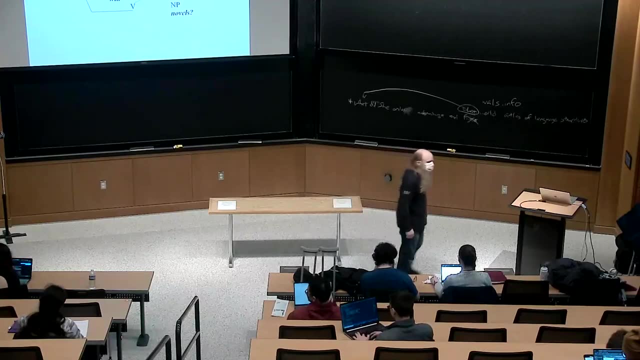 in to see past the auxiliaries, so English can't ask questions like type Mary will novels. this is out. I'm showing you this with yes-no questions in English. I could have shown it to you with v2, so the same thing holds in v2. verb second German phenomenon and many other. 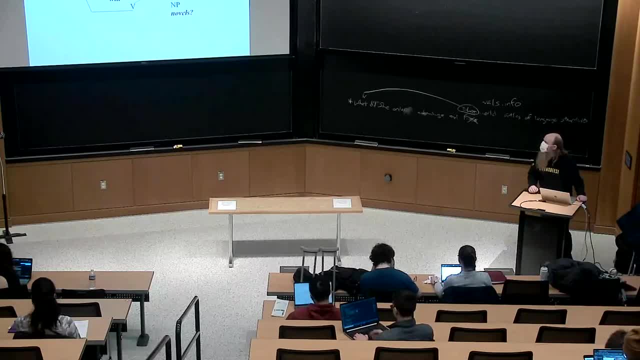 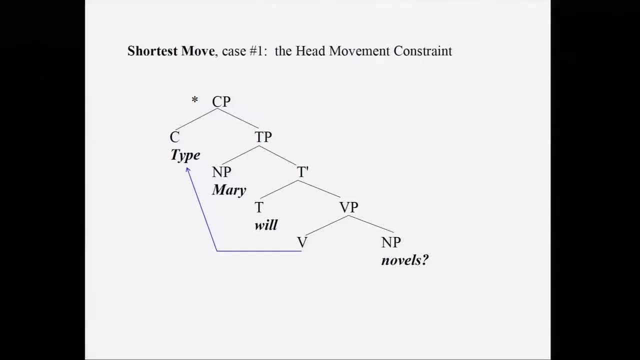 languages in which something has to be in C and what happens is, whatever head is highest moves into C, you do the shortest move. in German, you move the auxiliary, and if there is no auxiliary, you move the main verb. if there are multiple auxiliaries, you move the highest one. okay, so this is one example. 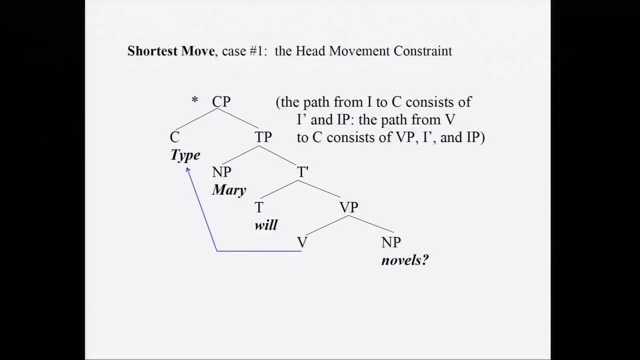 of shortest, shortest move. oh, I did it again, sorry, I haven't fixed this yet. the path from I to C, which is really the path from T to C, sorry, the path from where will is to where C is, consists of T, bar and TP, that is, those are the nodes that dominate T and don't dominate C, but the 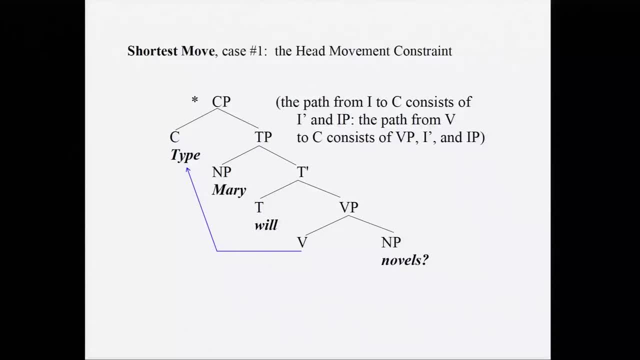 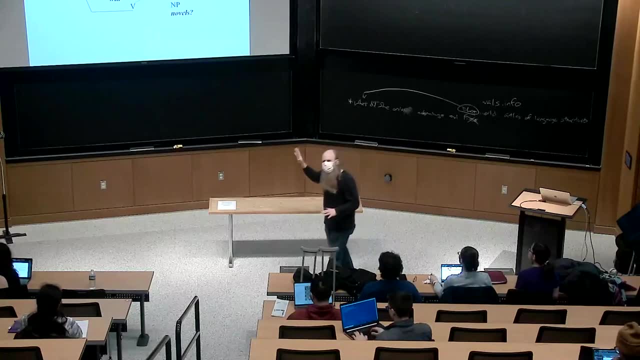 path from V to C consists of VP as well as T, bar and TP. do people see that? even though I wrote the wrong things on the slide, so please mentally search. replace I with T on this slide. I'm using an old term for IP which I'm not familiar with. 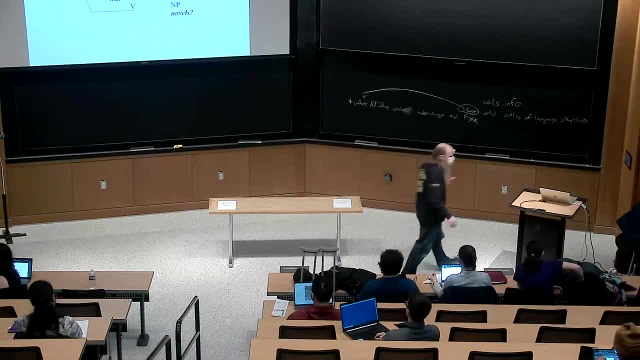 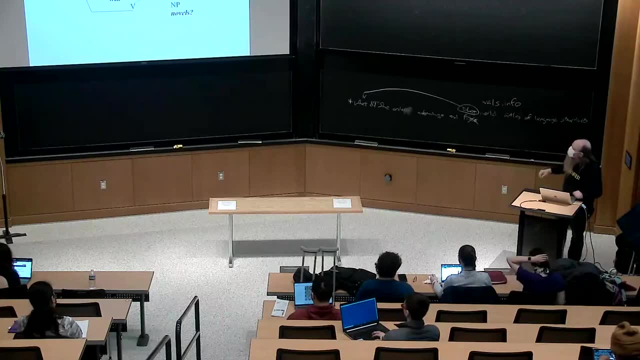 which I meant to go back and fix. there are no IPS anymore. yeah, so this is an example of how you use paths to sort of explain to yourself what you mean when you say that one move is shorter than another. as you can see, this is also a. 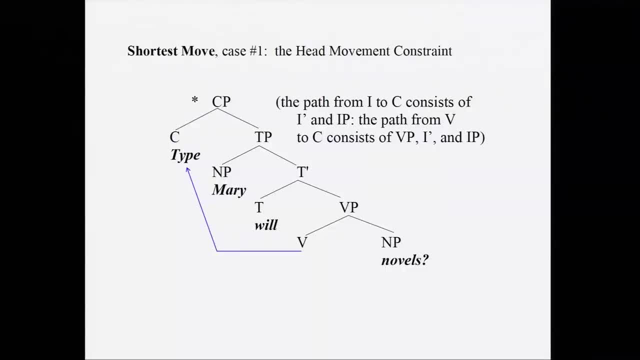 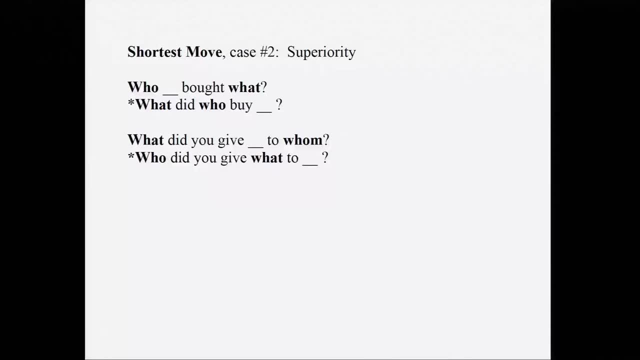 case in which one of the paths is a subset of the other, and then the second kind of case which we talked about last time, and this is one of the reasons that this is only as far as we got, because this case is a little shakier than the. 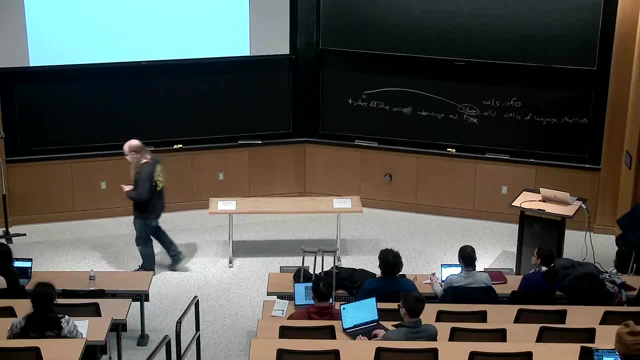 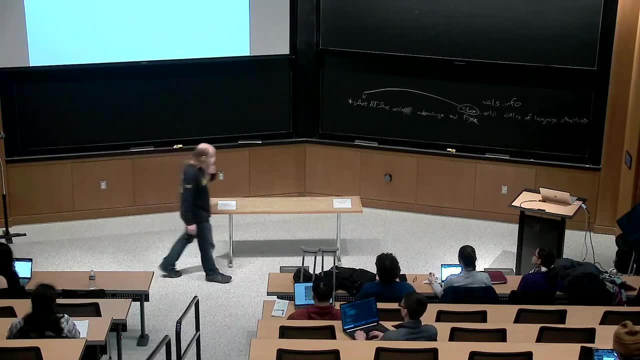 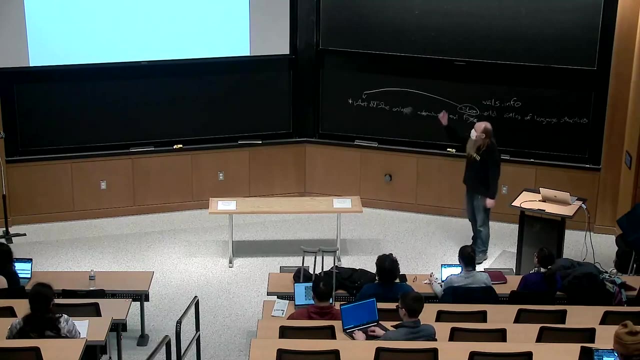 first one, the head movement constraint is extremely strong. if you violate the head movement constraint then your sentences are almost uninterpretable. superiority: there are all kinds of complicated semantic things going on that allow you to sometimes violate superiority, but at least in some cases, out of the blue, if I ask you who bought what? that's better. 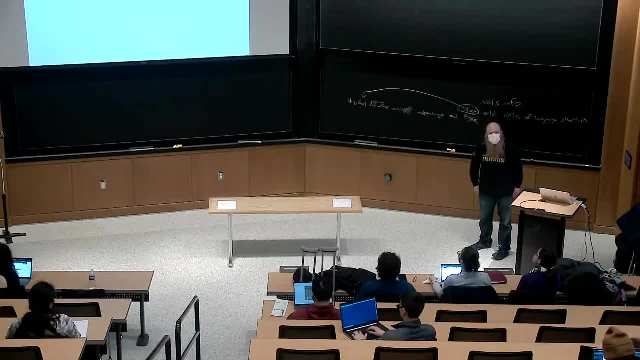 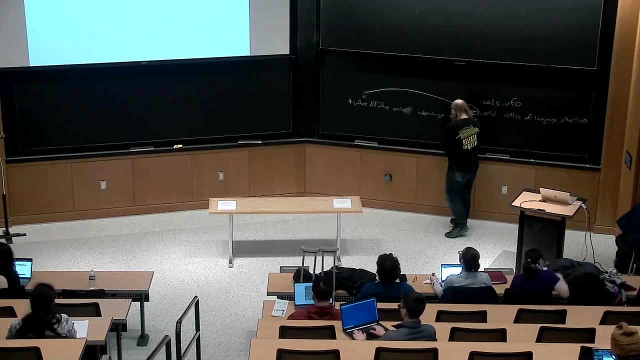 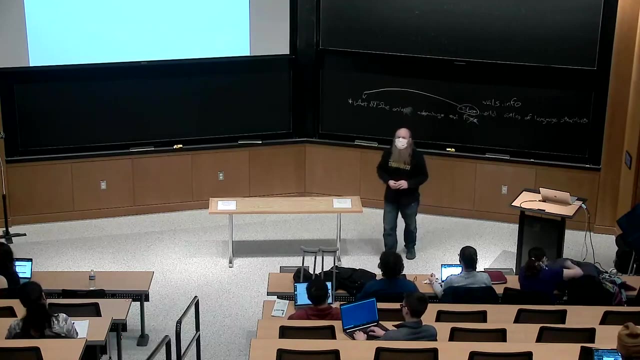 than asking: what did who buy? I was getting a general agreement with that last time. one of the things I said last time- and I think I think this is true- is that superiority judgments are particularly strong if you are talking about if there, if there are only two answers, so WH questions, multiple WH questions, what? 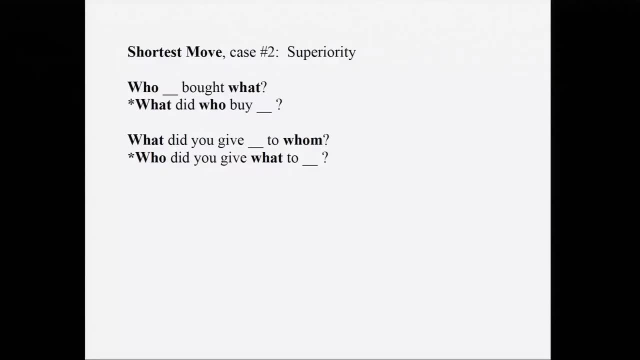 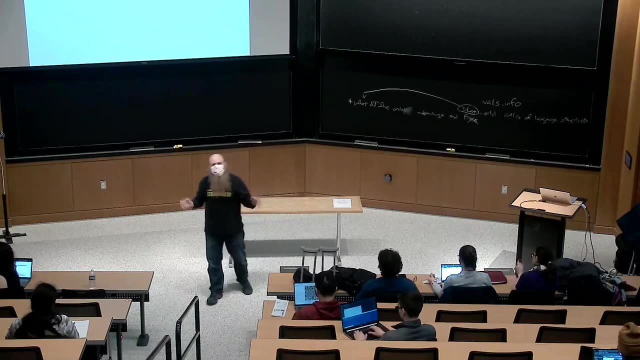 you're asking for are is a is a list of pairs, usually. so if I ask you who bought what, the answer is going to be: well, you know Sally bought chocolate and Bill bought novels, and you know Mary bought a computer, right. so it'll be a list of people and things such 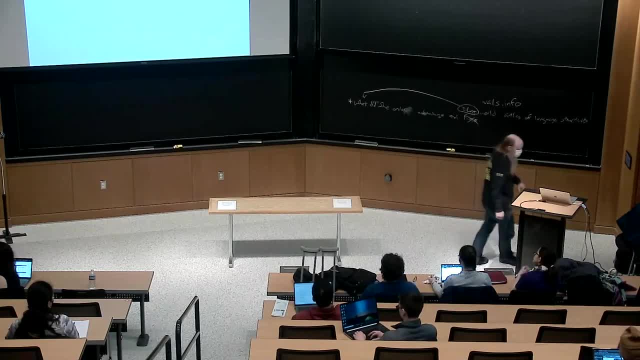 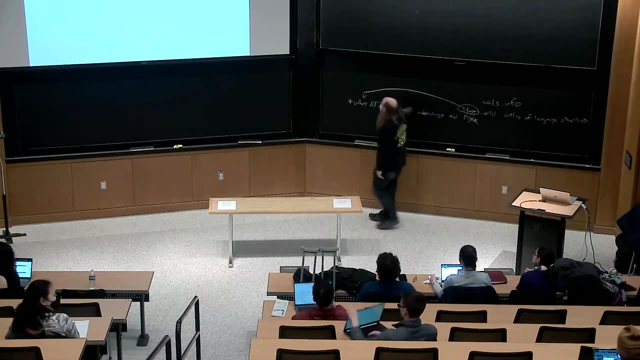 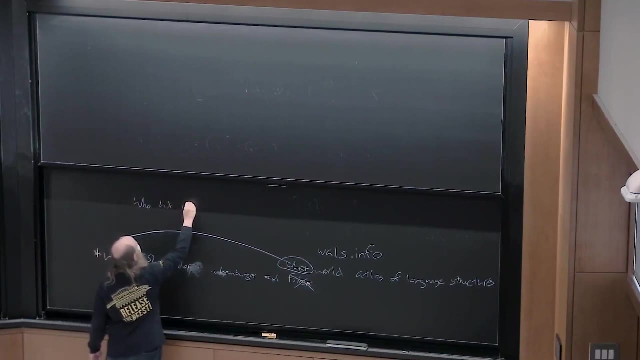 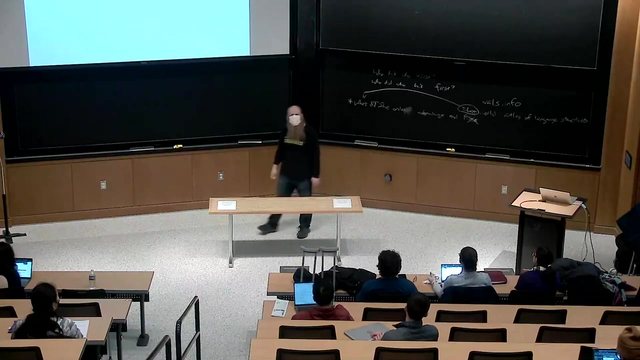 that the people bought the things. superiority- we talked about this last time, but superiority judgments are strongest when there's only one pair. so if you see two people fighting, you might ask who hit who first. compare that with who did who hit first? for me at least, that's a particularly strong judgments. are there people who prefer? 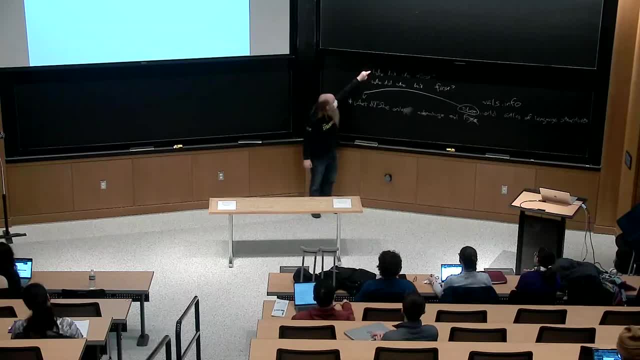 one I didn't see. let's see you show hands. who prefers the first of these to the second, who prefers the second to the first, who finds them both fine and is not sure why some of you raised your hands the first time. okay, so there are a. 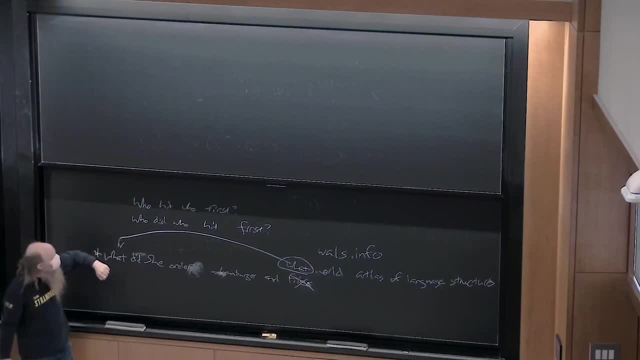 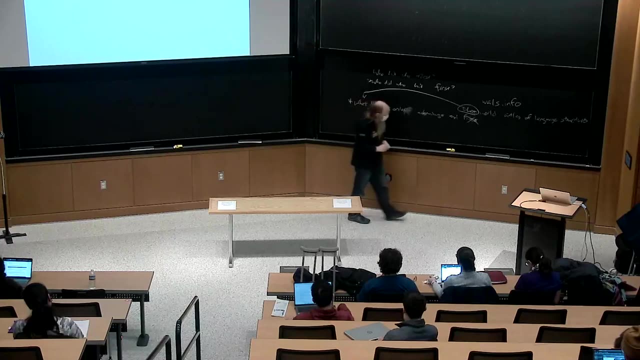 few of you who don't care whether there's only a single pair, but for many of you, this one is better than this one. so, okay, this is a phenomenon which is not as strong as the head movement constraint, but resembles the head movement constraint in that there's a preference when you've got a choice between two things, which 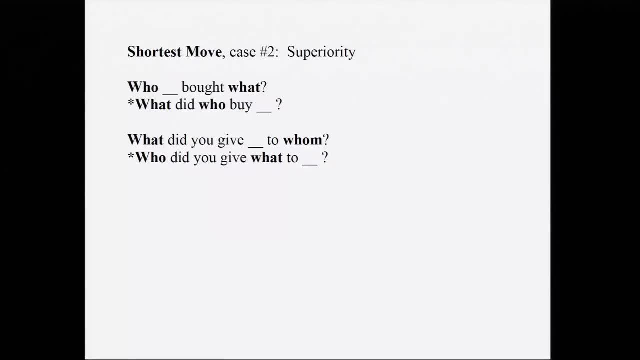 of them to move. there's a preference for moving: the higher one, the first one, And then here's case number three, which we didn't get to last time. This is what are called WH islands. Island, again, is a name syntacticians use for these positions. 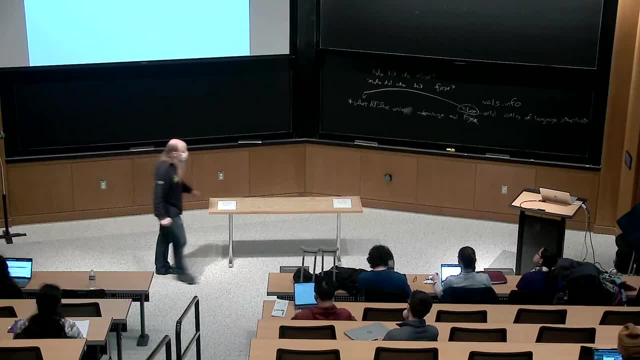 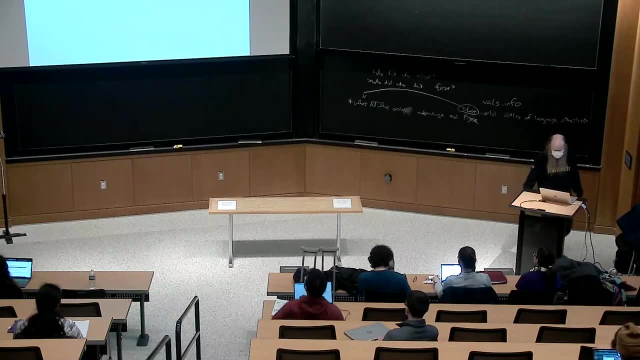 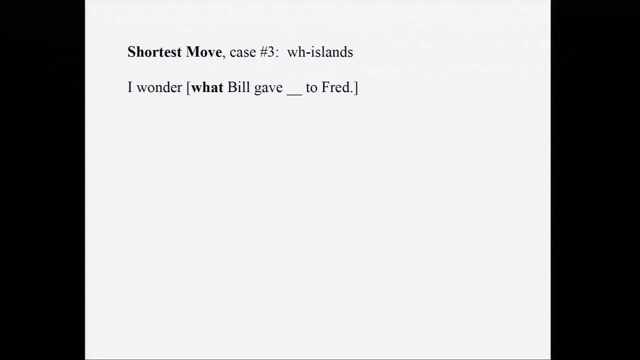 that you can't move out of. It's this metaphor. I guess that involves WH phrases not being able to swim. If they're stuck on an island, then they're stuck. So here's a sentence with an embedded WH question. I wonder what Bill gave to Fred. So this whole sentence is not a question. 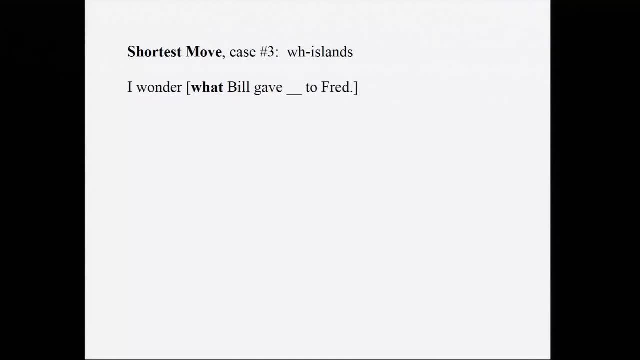 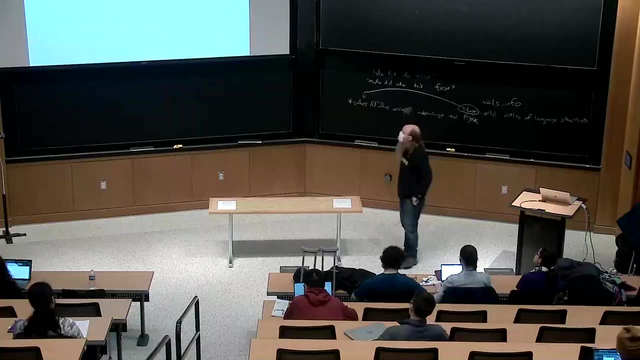 really It's a statement. I'm telling you something about my mental state. My mental state is one in which I don't know the answer to a particular question. That question is: what did Bill give to Fred? So there's WH movement happening in the embedded clause. 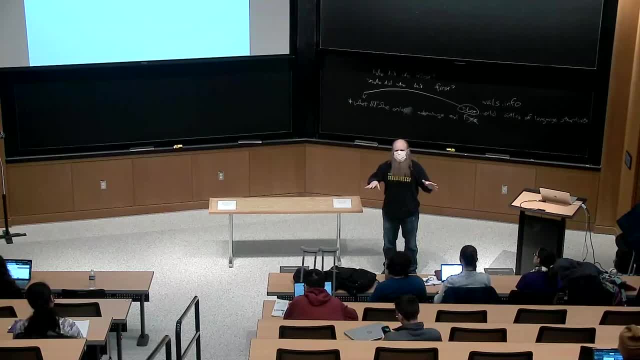 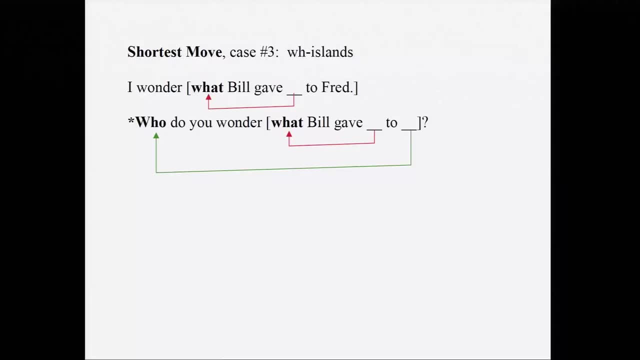 What has moved to the edge of the embedded clause? Is that clearer? Does that make sense? That's what's going on in this sentence. Now observation about embedded questions. If I ask you, who do you wonder what Bill gave to? 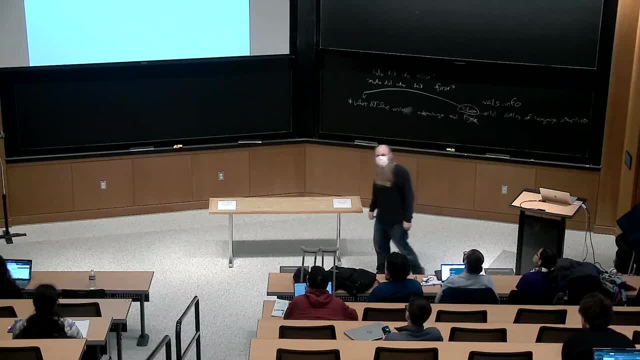 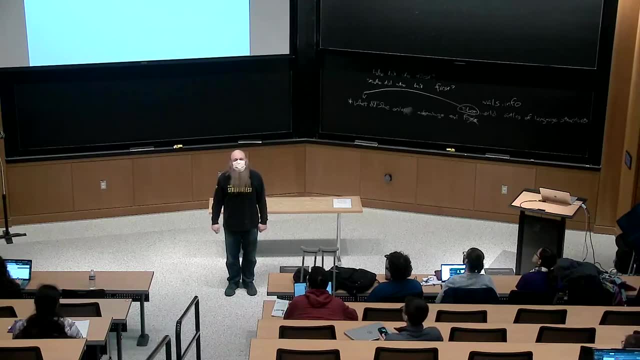 you're upset. So what did I do? Well, I turned Fred into a WH question, a WH word zzing. Now Fred is who? and I moved who out of the embedded clause into the matrix clause. Who do you wonder what Bill gave to? 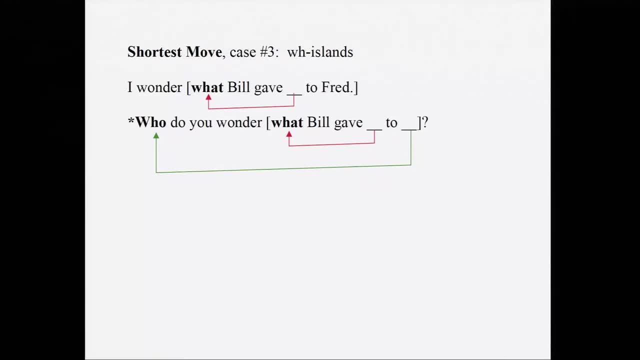 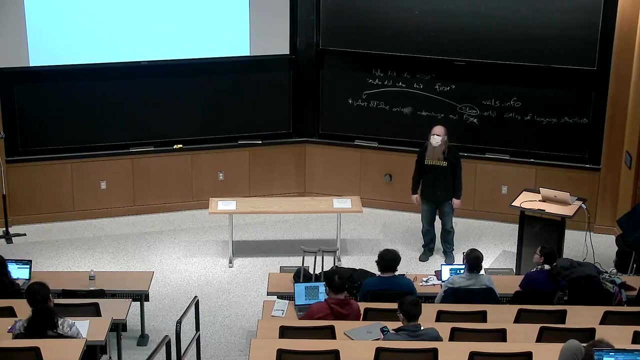 Where the answer is. well, I'm wondering what Bill gave to Fred. This ought to be able to mean that, but it really really can't. There's something badly wrong with this sentence. So this is called the WH island, A WH question. like what Bill gave to Fred in this sentence means single piece. So I mean, this is, it's just here now. it's not perfect, but at this point I'm not sure the impetus matters. So I'm going to talk a little bit about Tube. then. this is where I wanted to be here. I mean 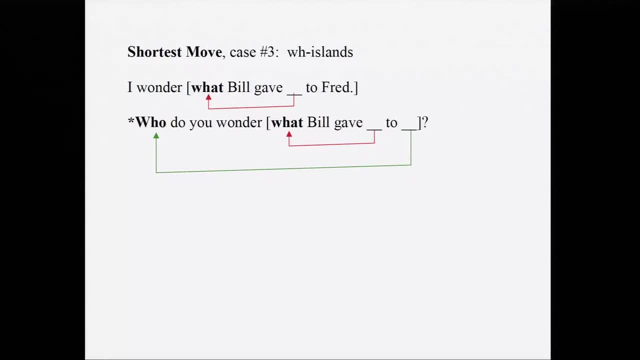 I think I have two on my list of questions. that, okay. Well, my second question this week was a question Bill gave to Fred is an island You can form that. That's what the first sentence says. I wonder what Bill gave to Fred. 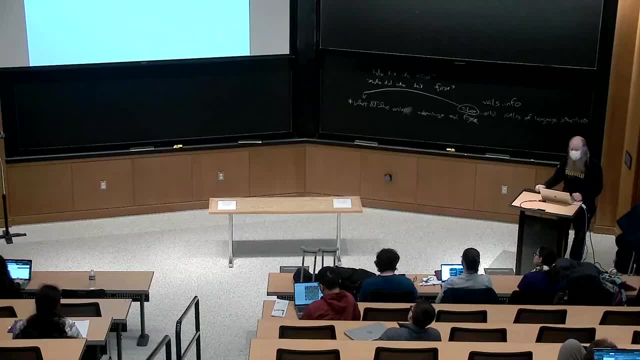 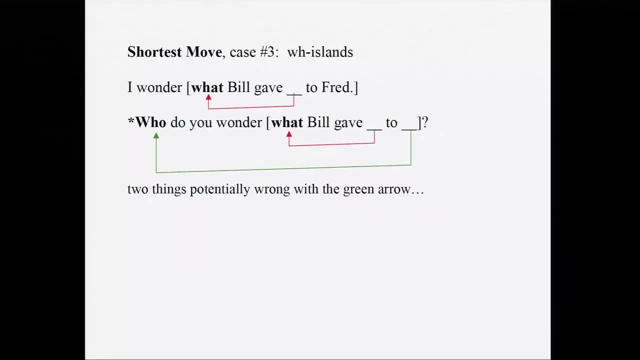 But you can't wh-extract out of it Proposal people have made. Well, look, there are at least two possible things that could be wrong with the green arrow there, the one that's going from the embedded clause into the matrix clause. One is: 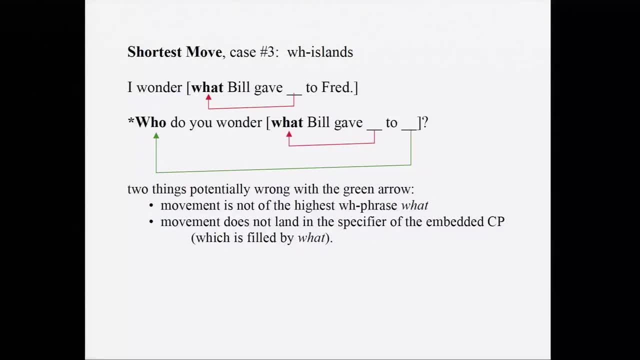 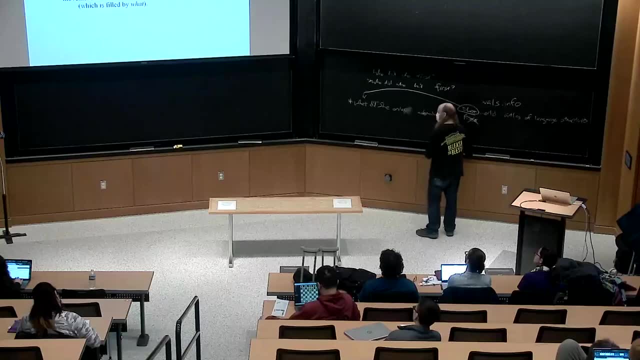 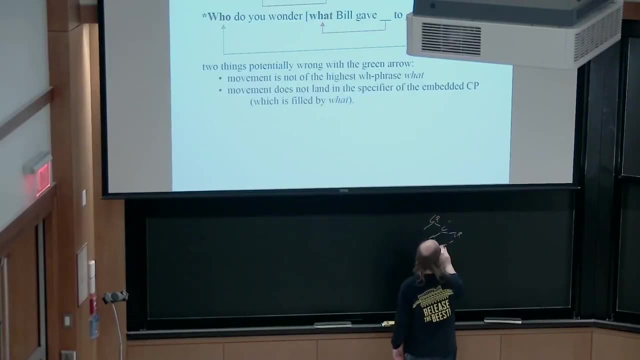 here I am in the matrix CP and I'm trying to decide what to move and there are two wh-phrases: There's what and there's who. I should really have a tree here. Let me draw a quasi-tree. Is it wonder? 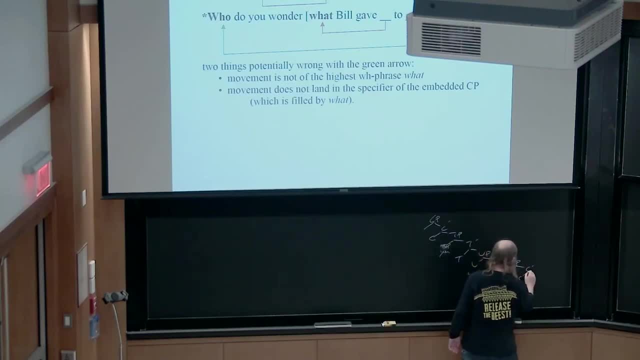 Okay, and then down here we have what, and then I'm out of board, so I'll just use a triangle here to who? Okay, so this is. you wonder what John gave to who? I know my handwriting is terrible, but can people see that that's. 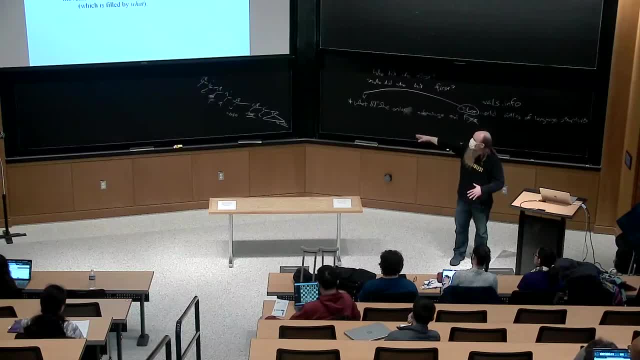 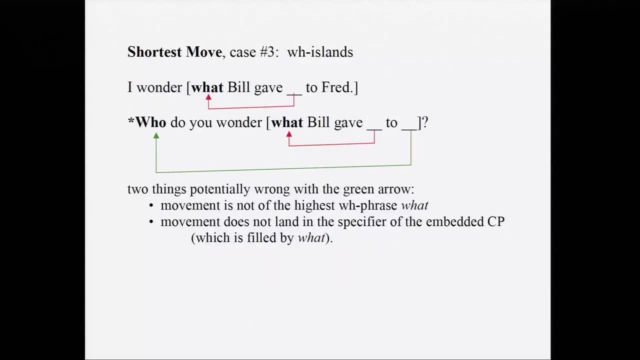 what that tree is meant to be. So this is the tree for the second sentence. This is going to be my attempt to draw the second sentence. So who do you wonder what Bill gave to? So we've got. we can fill in some of the gaps here. 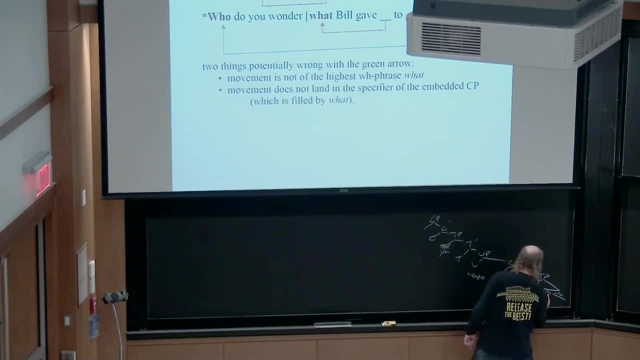 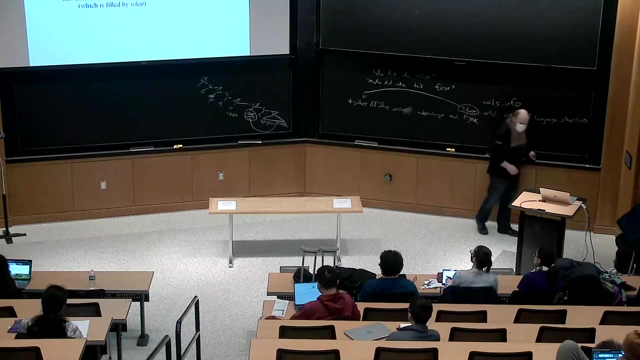 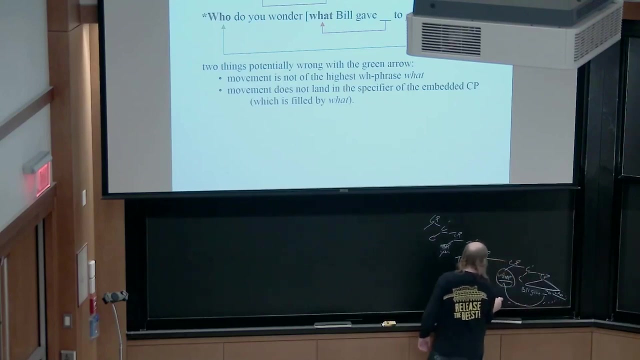 Bill gave blank to who. So we first moved what into the specifier of the embedded CP. and now- this is one of the few times in my life I wish I had colored chalk. Now we're going to take who and we're going to move it. 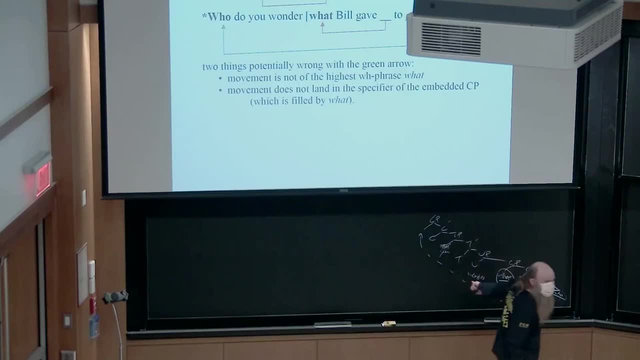 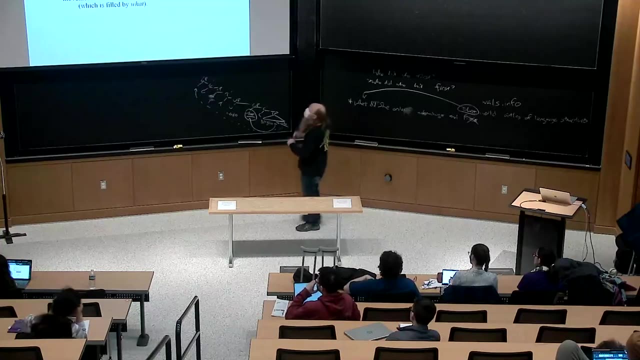 up to here and there's something wrong with this. Try to figure out what's wrong with it. The shortest move story about what's wrong with it goes like this: Well, actually there are two things that you could blame this on. One is when we're. 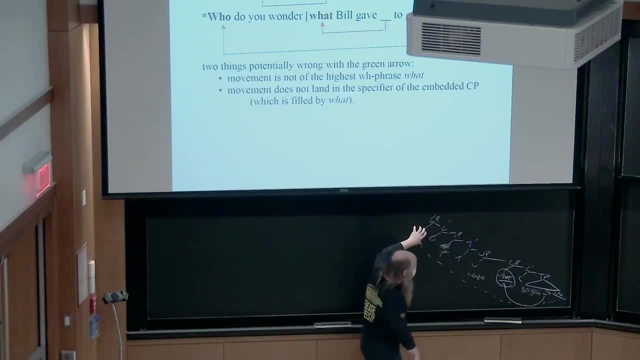 here and we're trying to decide what to move into this position. well, at this point there are two wh-phrases: what and who, and what is higher. So maybe one thing that's wrong with it is basically superiority. over again, You've got two wh-phrases. you have to pick. 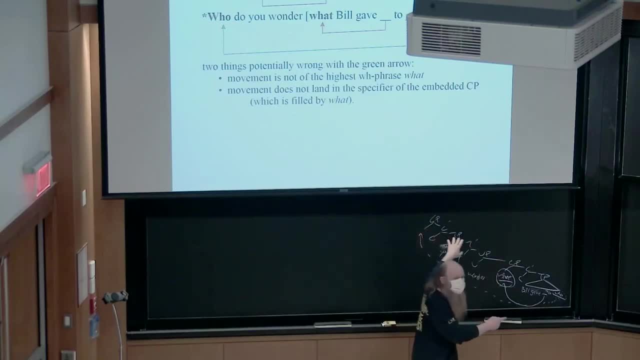 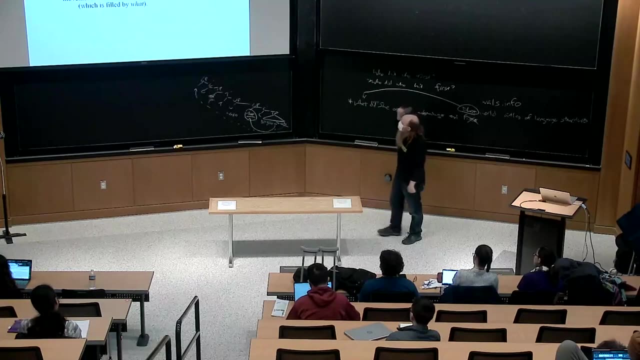 which one to move. you should move the higher one. You didn't, So you didn't pick the shorter move. And the other objection you might have to this green arrow goes like: this Wh-movement is to the spec of CP. Here's who sitting here. If you're going to, 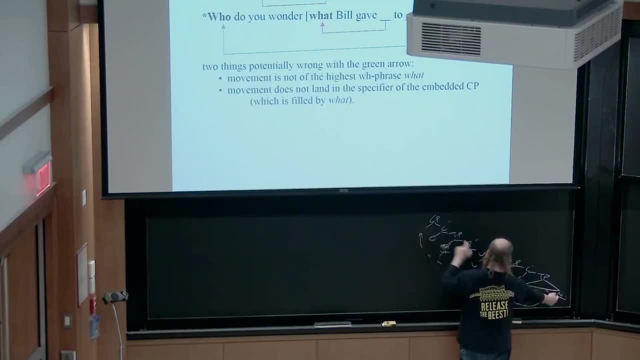 move who? well, you shouldn't move it here. you should move it here. Sorry, I'm gonna do that without putting my body in the way. You shouldn't move it here. Here's the spec of CP, yeah, to which it's gonna land. but really, what you should do is: 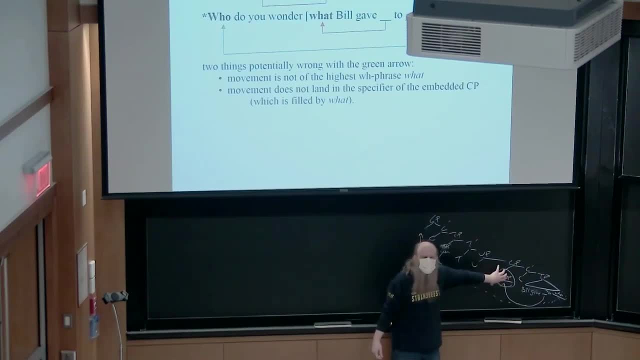 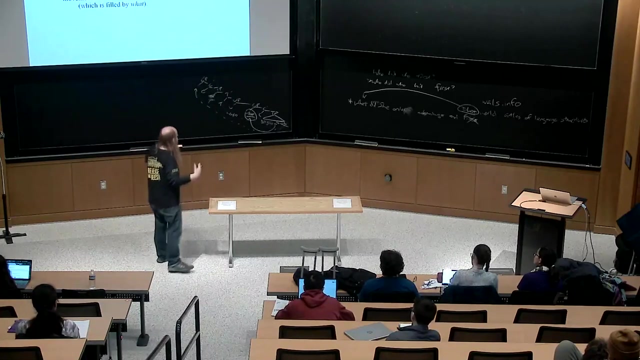 move it here, and you can't because there's a wh-phrase here. This place is stuck, And so the ill-formedness of this sentence. the star is. you know this feeling you're having trying to satisfy multiple conflicting requirements. 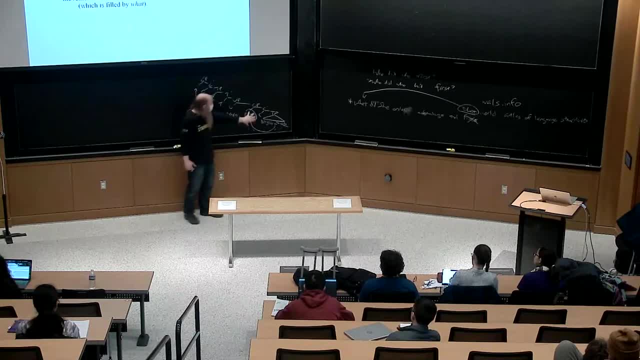 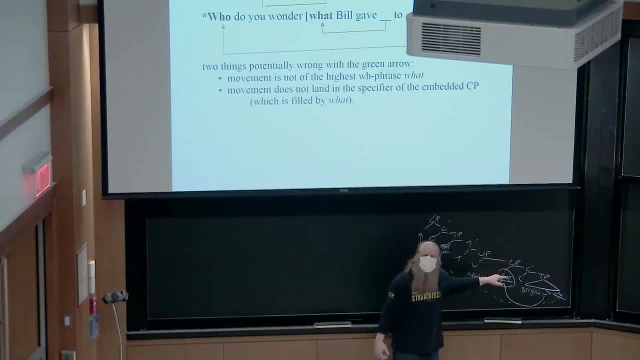 There's a Greek tragedy going on here, Who Absolutely needs to land here, but there's what in the way, And so you know who wants to kill its father and marry its mother, and then bad things happen. Yeah, you can't do everything that you want to do. 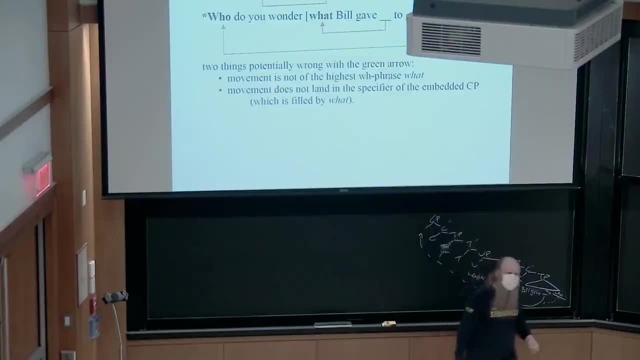 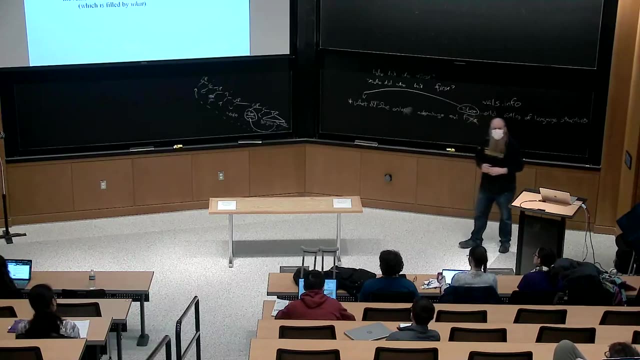 So this wants to make the shortest possible move and it can't and it's unhappy and it pouts and that's got the shape of a star. That's a story, anyway, about why wh-islands are islands. Do people see the problem? Yeah, that sentence is bad and it's not like it's unclear. 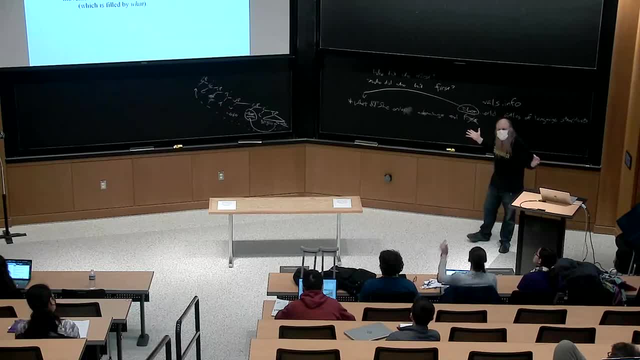 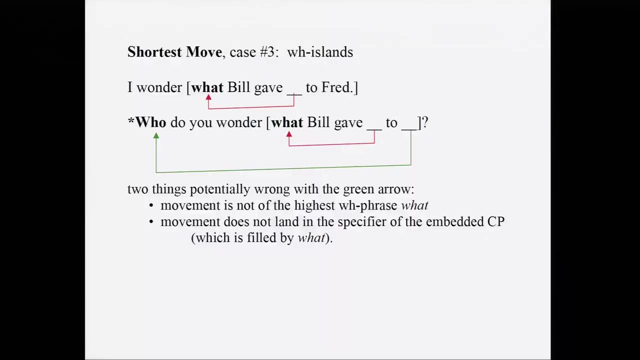 what it means, but you just can't say that, Yeah, you can't. who do you wonder what Bill gave to? the closest you can come to saying it in English is to say things like: who is it that you're wondering what Bill gave to him or her? 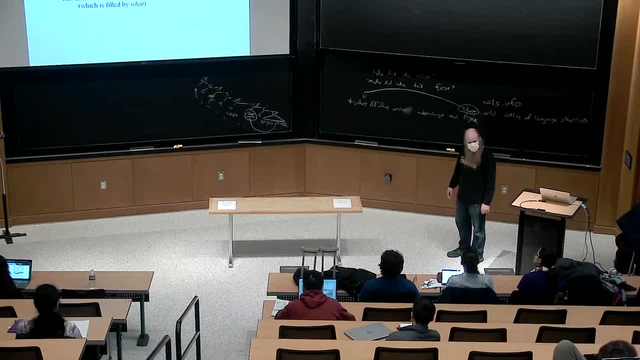 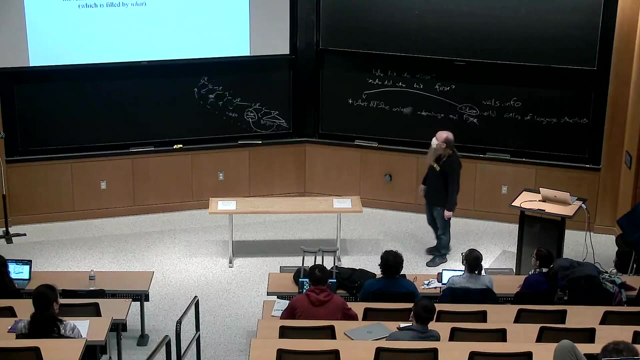 So sometimes for some people, putting in a pronoun improves these sentences. for me, The effect is not so strong. There isn't a very good way to say this. There are languages in which this is okay, which is an interesting thing. You know they're interesting questions about why, but in 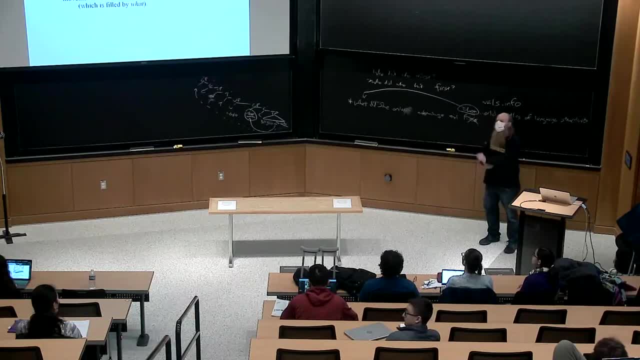 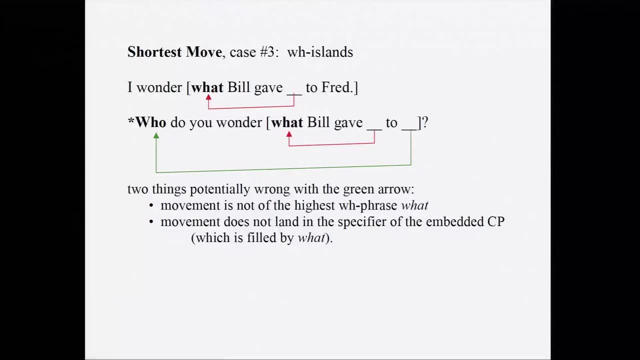 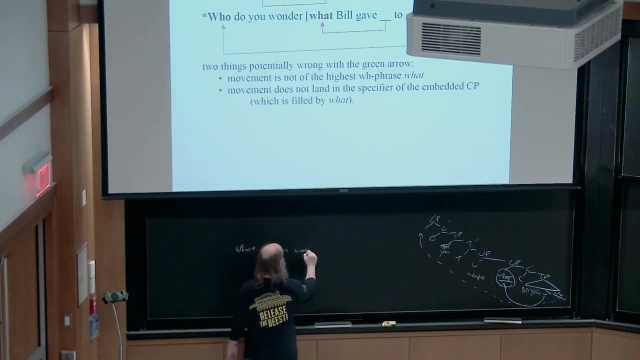 English not so much. Yes, what do you wonder Bill gave to who? So one of the things I just said was: you know, when we're asking what went wrong with the, I've got up there, Who do you wonder what Bill gave to? one thing that you could. 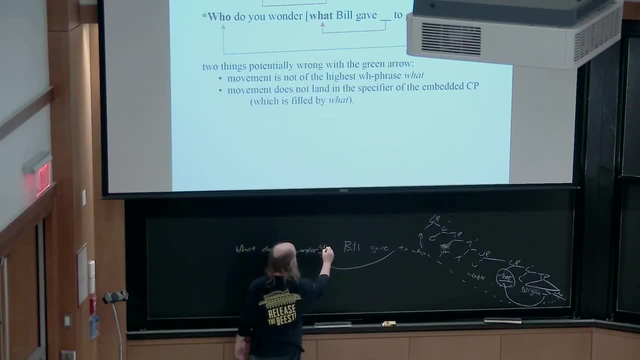 blame it on. is you moved who and what is closer? what you should really have done is move what. I don't know about you guys, But for me what do you wonder Bill gave to who? I can't say. So this is another one of these sort of Greek tragedy things. 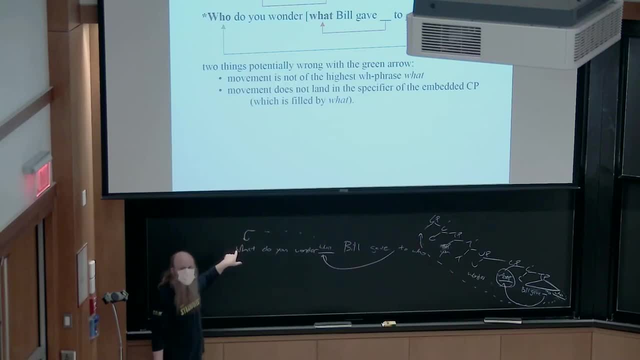 shortest move, really wants that, this to be the thing that moves. but the result is that Let's think about what wh movement does. it makes questions right, So you know when you move what. here you're making this into a question. you know, you wonder what Bill gave to Bill, to Fred or? 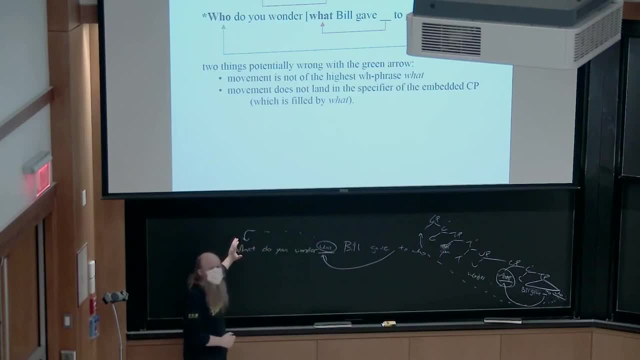 whatever. If you move it up here, you're making this into a question, and maybe what we're seeing is that you can't do both. We could demonstrate that without without doing nwh Island, So it's also bad, at least for me. 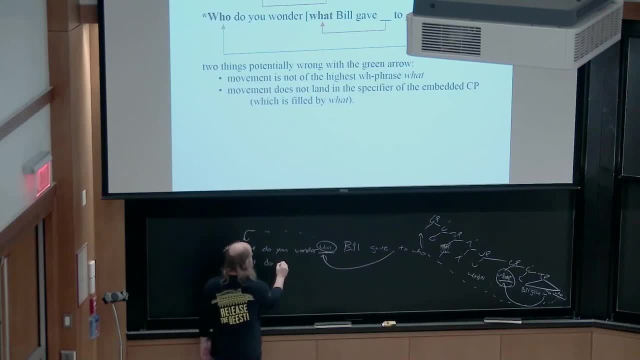 I'm going to star this. It's also bad, at least, for me to say things like: what do you wonder Bill gave to Fred right, This is also out. So it's just independently impossible for what to start here, move here and then move here. 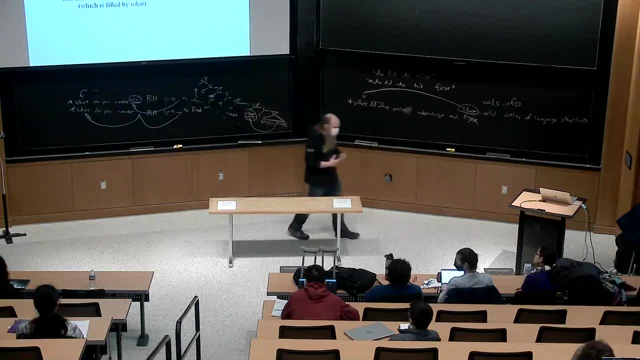 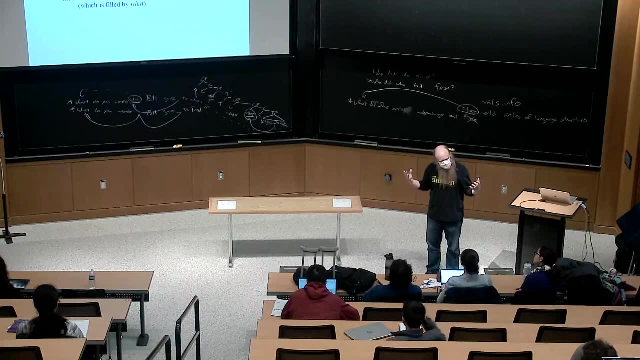 It's as though what can't be the you're attempting to form two questions with a single wh word and you can't. Your last one is okay. What do you wonder Bill gave to Fred? You could say: what do you wonder whether Bill gave to Fred? 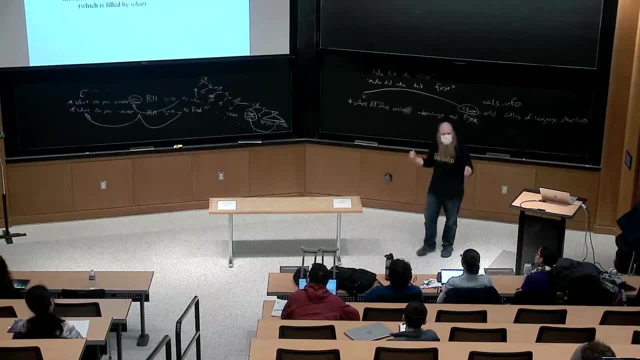 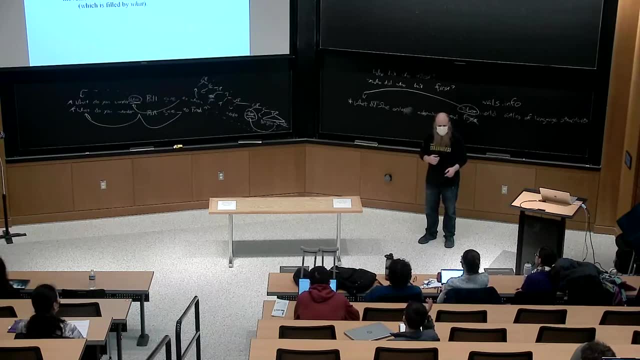 Yeah, for me at least, I can't say this, But I agree with you that if I were to make it, what do you wonder if Bill gave to Fred? That's still bad, but it's better than this, My feeling about it. 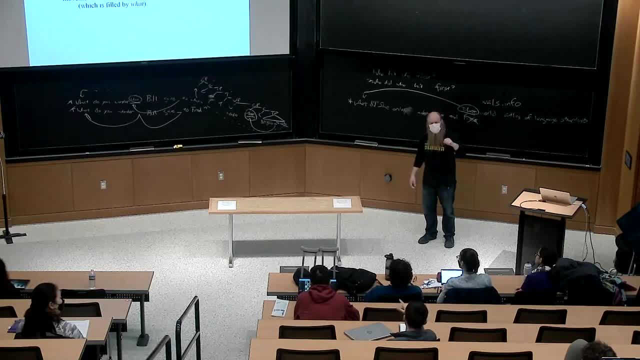 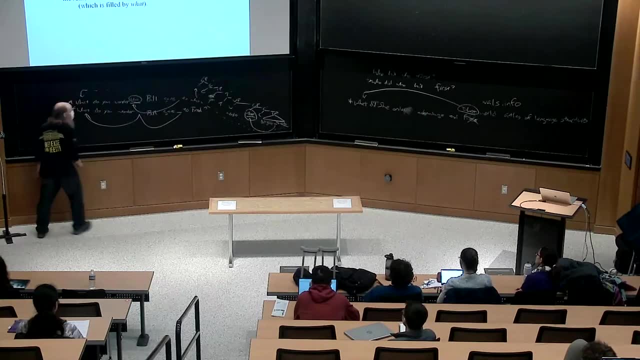 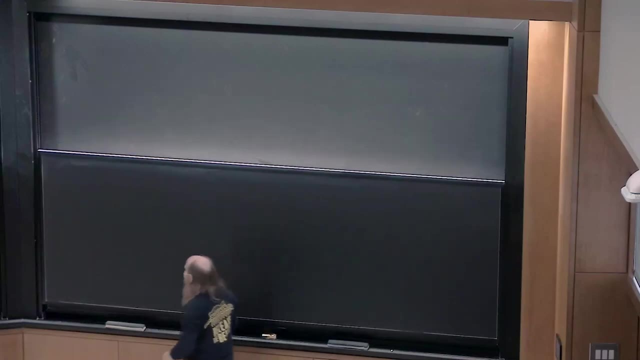 Just it Wonder replacement. Thank you, Yeah, so notice. good point, Right, that's it. So wonder. selects for an interrogative CP. You can say: I wonder who left, why they left where they went, But not, or you know whether they left their various things. you can say: 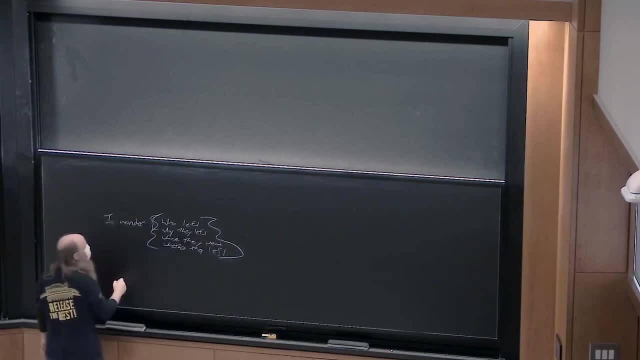 but they're all questions. Yeah, So wonder, Wonder selects for a question and that she left is no good. Think is the opposite. You can say: I think that she left, But not I think whether she left, or I think we left, things like that. 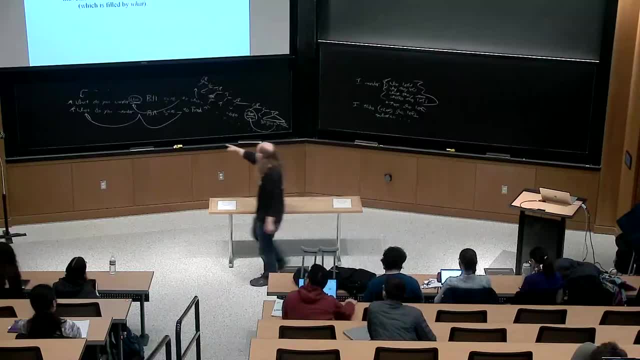 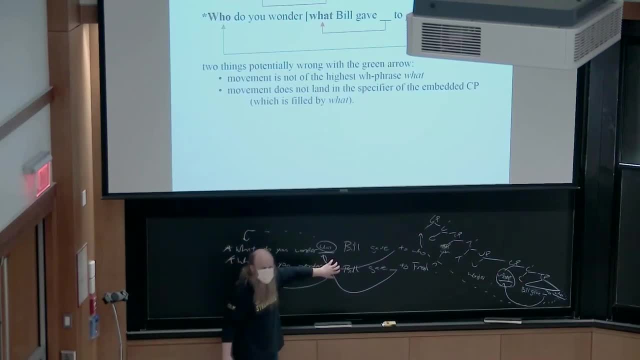 Yeah, so you're absolutely right. If I make that think, what do you think Bill gave to Fred? Then what is going to be able to move up here, Because think doesn't care, In fact doesn't want this to be a question. 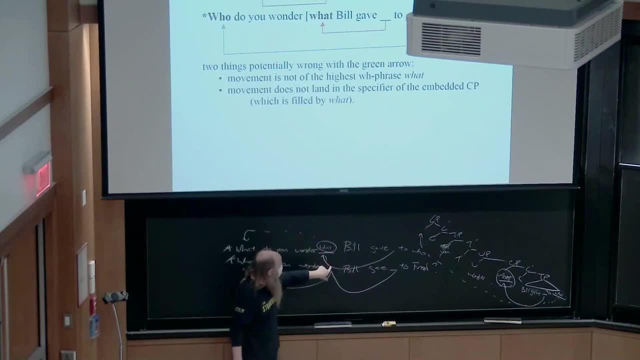 But wonder, does want this to be a question, with the consequence that if what goes here it's as though it's stuck right, It's got a job, It needs to make this a question. If it moves, then you know it isn't a question anymore. 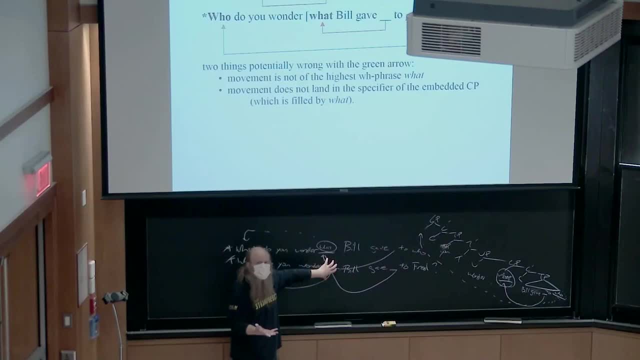 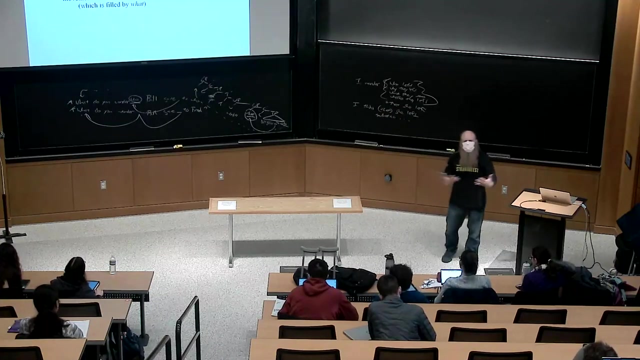 Something has gone wrong. So we have two sort of conflicting things there: shortest move, that says in this example, what should move up to here should really be what? and then you have wonder which says no, what, you stay here, You have a job, And these two things can't be reconciled. 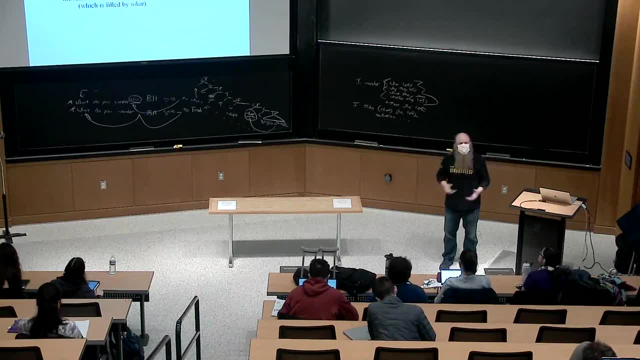 Notice that we are out of the domain of optimality theory here, right? So if you remember optimality theory back when we were doing phonology, we were talking as though sometimes you know, when you have two things and they're fighting you just. 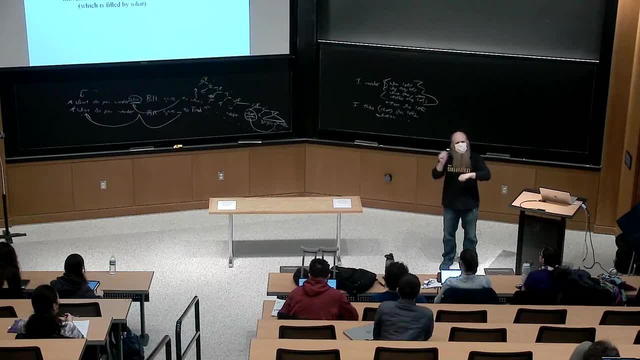 you know, try to find some middle ground. You find the thing that's best, or you decide who's more important. That's not the way I usually settle fights between people, But apparently in optimality theory that's what you do. You decide which of these requirements is the most important one. 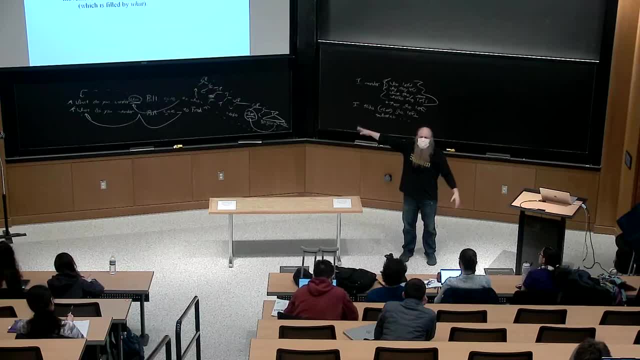 The way I'm talking here is not that. this is more Like here. you have two conflicting constraints And so you die, You can't do anything. There's no way to make everybody happy. Yeah, Okay, So this has been an exercise in well. 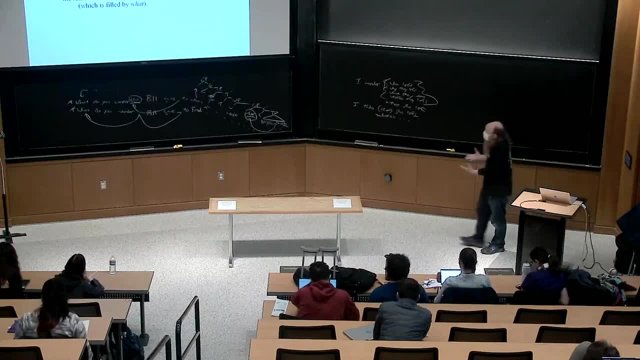 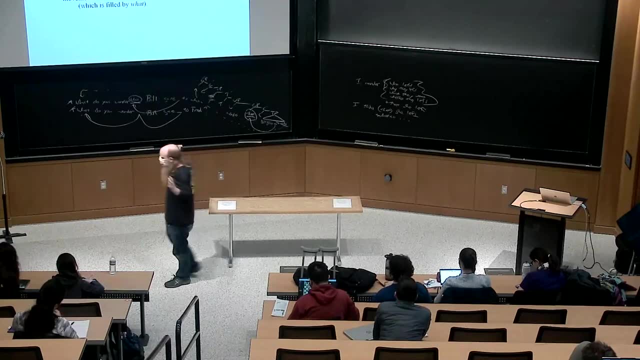 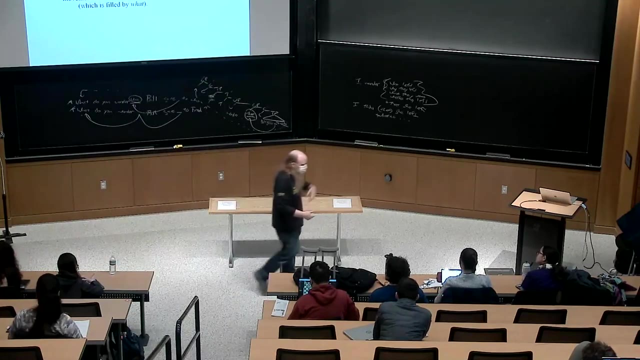 first showing you some other places where movement is barred and then also sort of giving you just a hint of a very large and interesting literature in which syntacticians look at a variety of phenomena and try to unify them. So you know, head movement, constraint and superiority in WH islands are all things that were discovered independently at different times by different people. 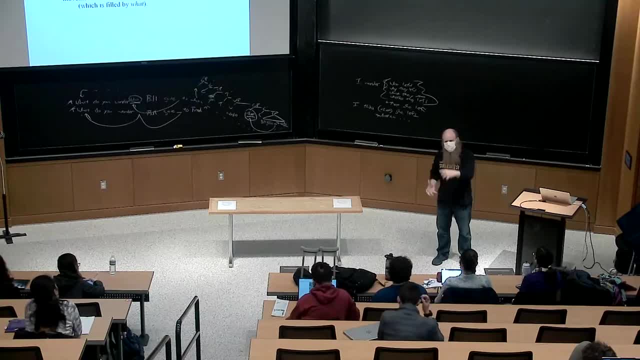 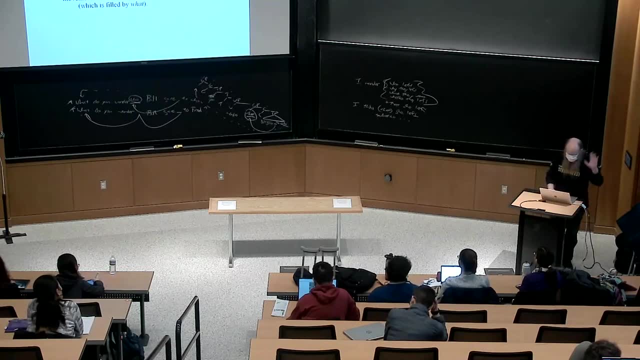 And then another generation of syntacticians came along and said: don't these all belong in the same box? You know that's where we are at this point. Yeah, Okay, Lots more work like this to talk about, But this is 24 900. 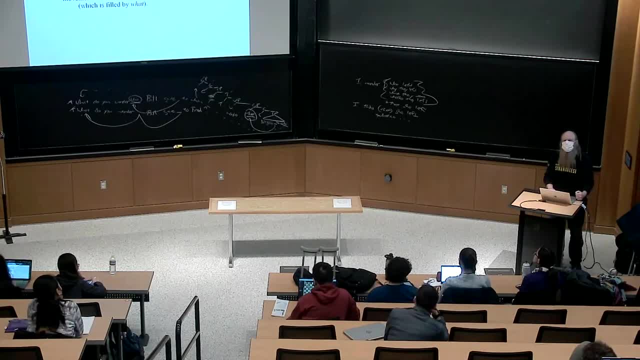 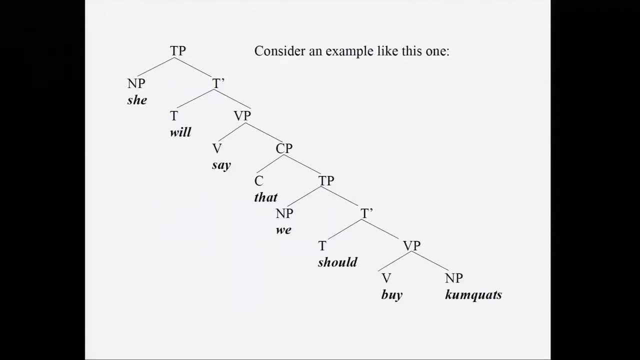 And although I am a syntactician- I looked at the syllabus, by the way, and we're actually more or less on track- I was astonished We're supposed to stop talking about syntax today, And so we will. Okay, One more thing for me to show you about syntax. 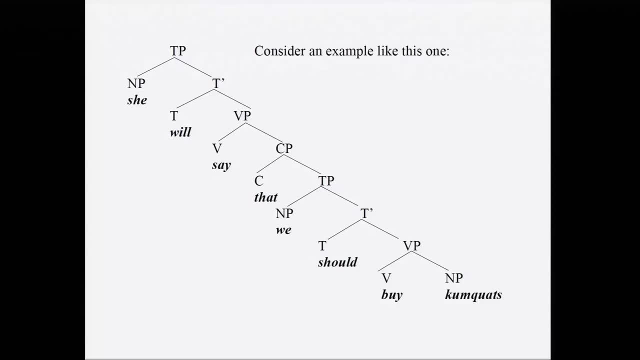 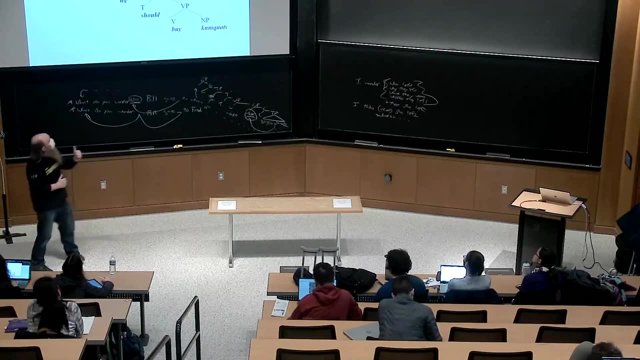 It's actually kind of connected to this, to Joseph's point. Here's the sentence: She will say that we should buy kumquats. Questions about this sentence. Does this make sense? Did I put anything in here that's surprising or disturbing? 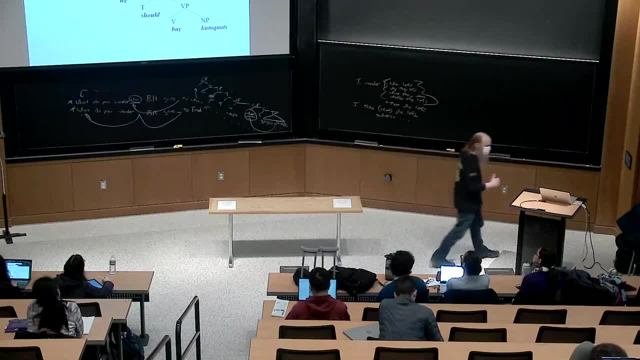 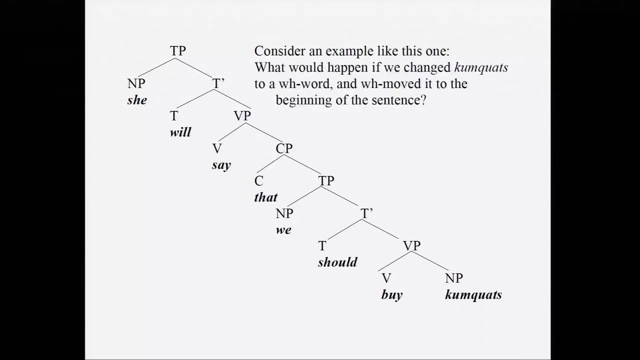 Yeah, I think I have a new thing in T, which is: should that? maybe that's not so alarming. Okay, And now what happens if we change kumquats into a WH word zap, And we WH move it to the beginning of the sentence? 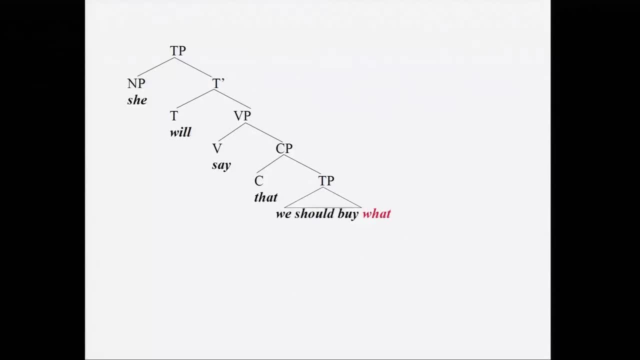 Well, you know. so that's me turning kumquats into what and also turning the TP into a triangle because I was running out of room, and then we're going to move what into the matrix clause, So we'll get what. will she say that we should buy? 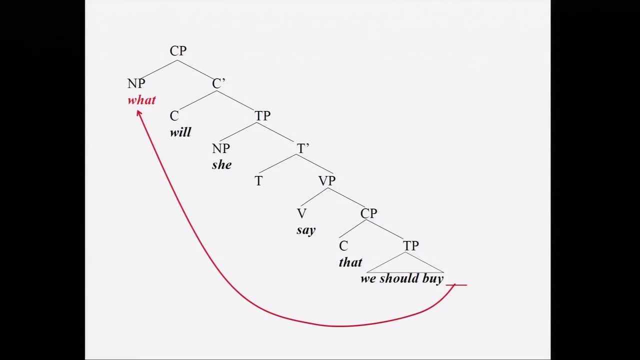 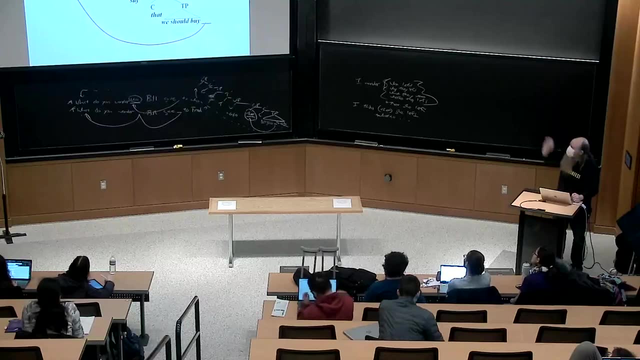 So we've done WH- movement of what- and we've also done head movement of will from T into C. I haven't drawn an arrow for that. Okay, and that's how we form that WH question, But given everything I just said about short, 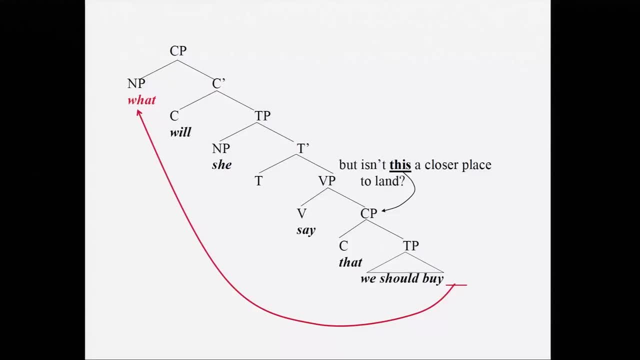 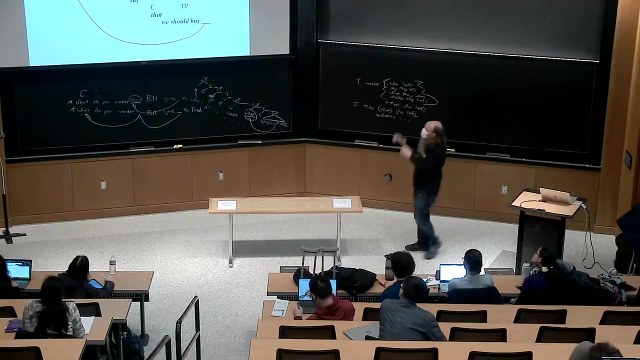 just move. You might worry, might say to yourself, but wait, isn't CP a closer place to let that lower CP that we should buy? Isn't that a closer place to land after all? WH words move to the specifier of CP. Here is an example where there are two CPs. 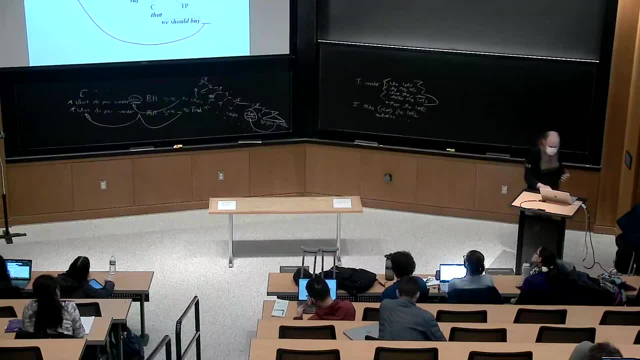 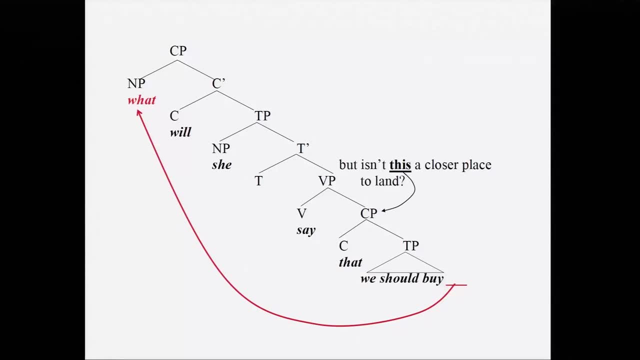 right. So what should we? what should we do? And there are various theories you can have about that. one would be to say, yeah, WH phrases move to specifier of CP, but it's specifically negative CP. They form questions, So not that kind of CP. 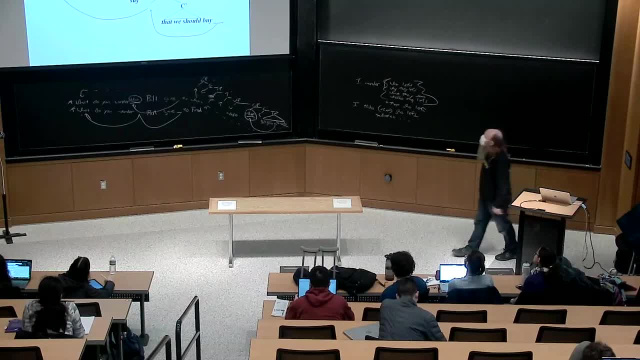 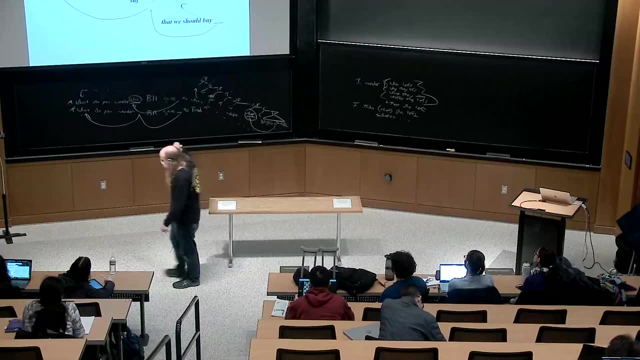 But you know, another kind of theory we could have would be to say: no shortest move is correct. The fact that what can in principle land in the specifier of CP means that it must. So it's not possible to do the arrow. that bless you. 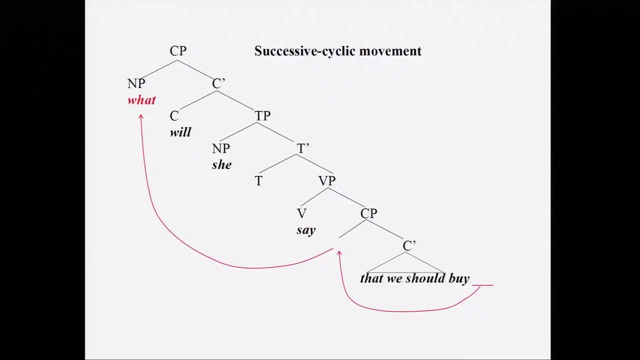 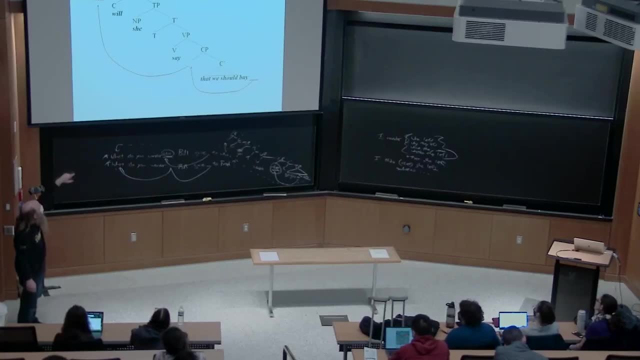 The longer arrow that I showed you on the previous slide, where what just starts down there and moves in one hop up to their movement is always the name for this Is successive cyclic. It's always in little hops. You can't move from one CP, out of that CP into another CP without stopping at the edge of the CP that you started out in. 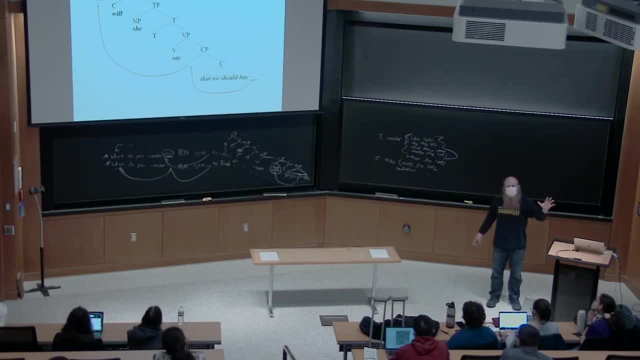 This is something that was proposed by Noam Chomsky decades ago, And when he first proposed it, it was met with widespread derision. People were like, just because of the shortest move constraint, You're going to say that we're doing all these little hops. and then there was immediately a flood of 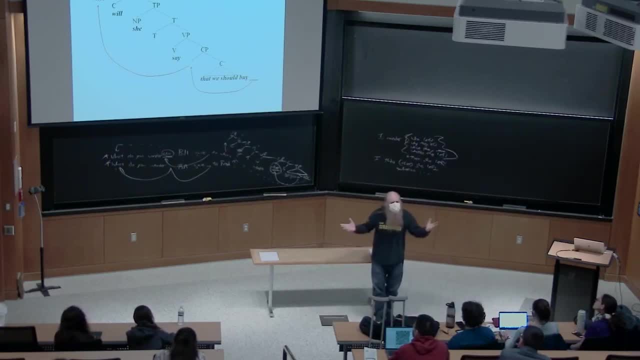 Really good evidence that this is true. It really does work this way. I'm going to show you one piece of evidence that this is how WH movement works. It's going to be kind of involved, So I'll try to go through it slowly. 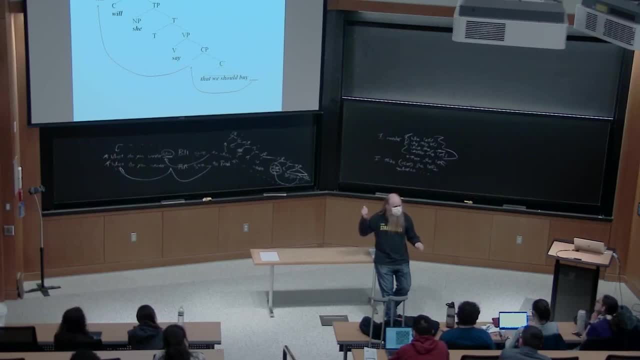 Did you have a question? Yeah, So if we move it up to where the CP is, then it would be like she will say what that we should buy. But like I feel like that sounds weird, Like I would say like she will say what we should buy, or something. 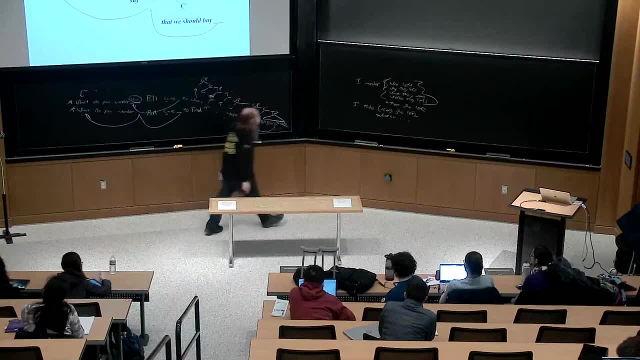 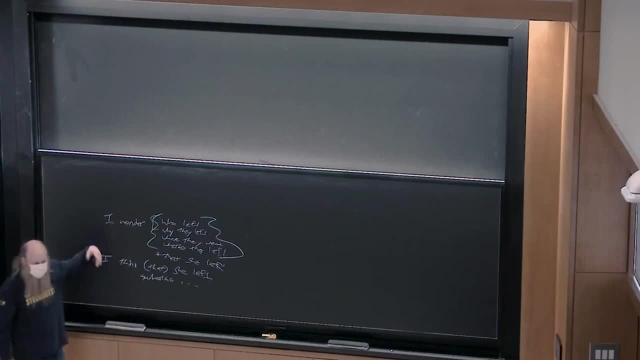 I don't know. No, Yep, No, You're right. So say we talked about. there are verbs like wonder that need to question. There are verbs like think that need to not have a question. say can have either one right So she can say she will say that it is raining or she will say who left. 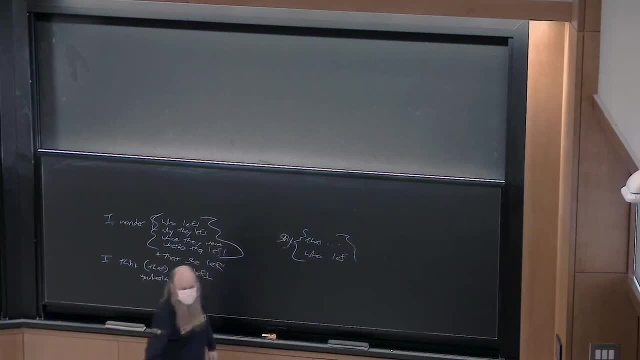 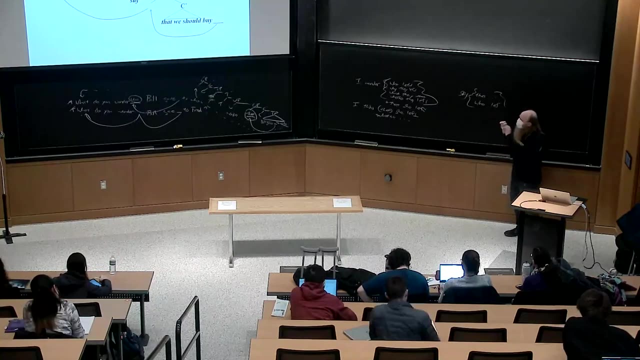 So say, has both options. It can have either a question or a statement. but actually the evidence that I'm going to show you about successive cyclic movement Shows that it actually doesn't matter whether the higher verb Can select for a question or not. 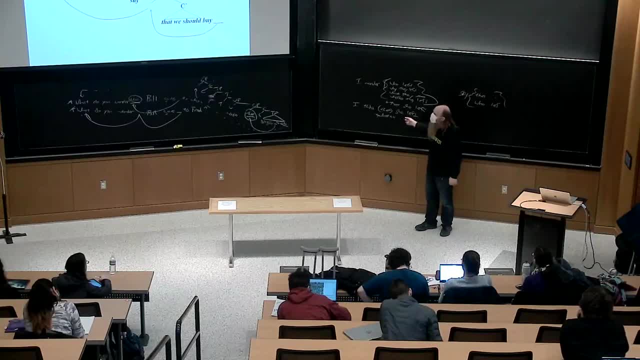 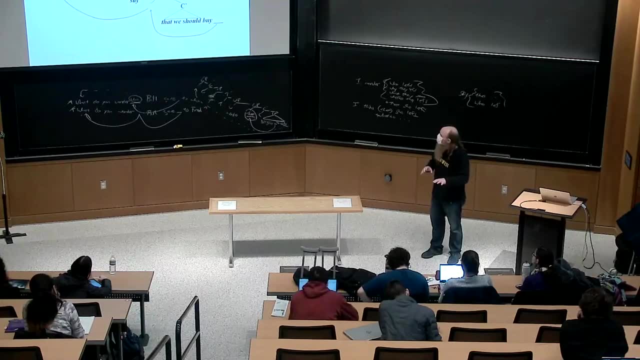 But even for verbs like think, that have to select, for statements, you get successive cyclic movement. So you're raising a very good point, which is- I'm sorry I'm going to hijack your point- this movement, this first movement, It's not driven by the need to form a question. 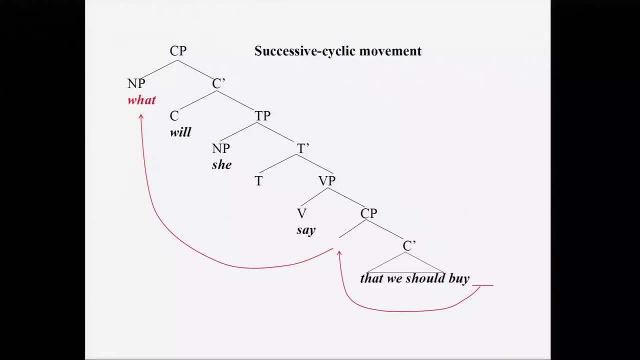 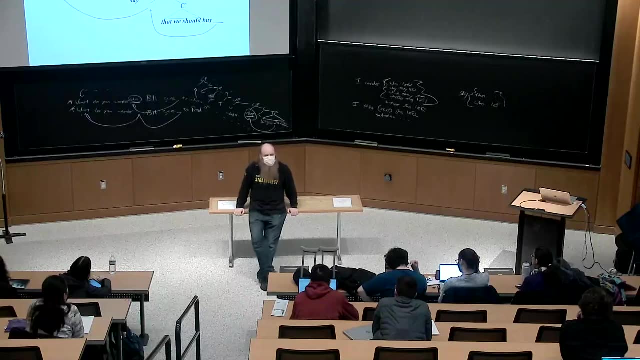 right. It's not that this WH phrase is moving here to make that embedded clause The question. it's just moving there. And then there's this question about why, like why does successive cyclic movement happen? But what I'll try to show you now is that it does happen. 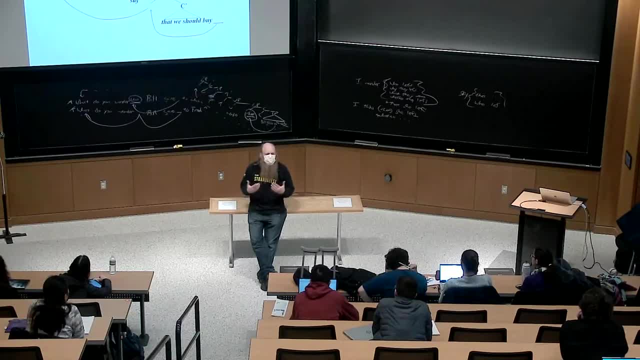 And so we need to get used to it and try to understand why. but, but you know, we need a theory of why, because, it's true, does happen. Okay, I haven't yet shown you any evidence that this is true. so far, All I'm doing is asserting, through the force of my personality, that this is how WH movement works. 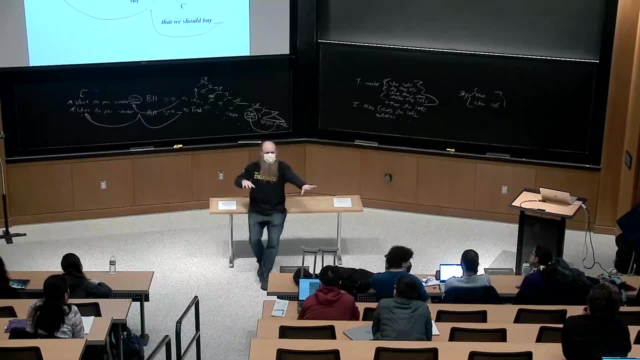 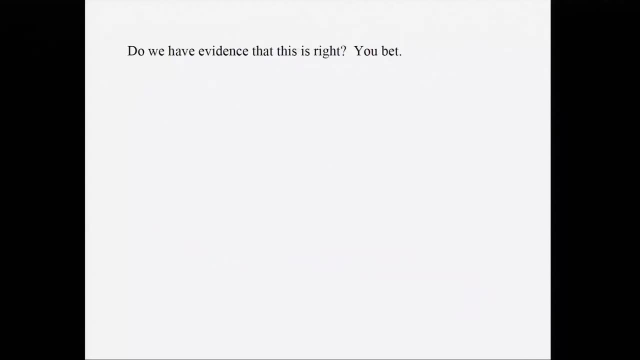 Let me now show you some evidence. Okay, Right, The evidence involves: do we have evidence? This is right. Yes, Evidence comes. There's lots of evidence for this, but I want to show you one of my favorite pieces of evidence. 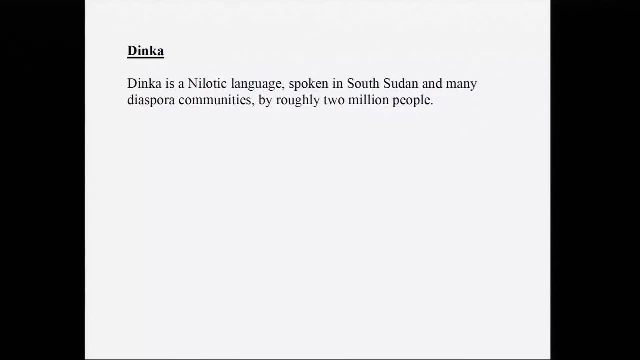 It comes from a language called Dinka, which is a nilotic language. It's spoken in South Sudan and in lots of diaspora communities, including a big community here in Boston by about 2 million people. It's phonology is lots of fun. 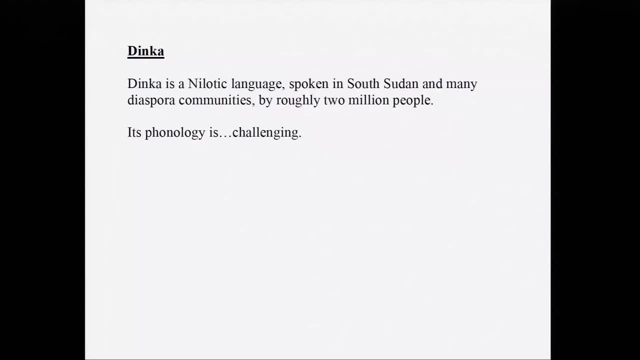 We did a field methods class on Dinka a few years ago. It has all kinds of shenanigans It gets up to with vowels. Actually, let me see I can play you these shenanigans in a way that you can hear. 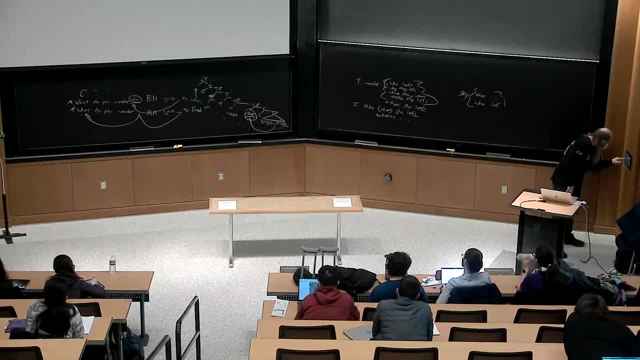 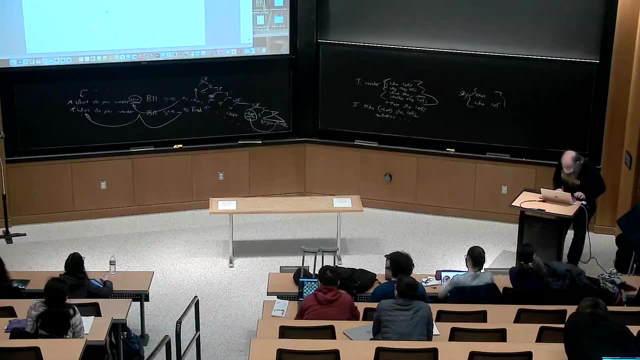 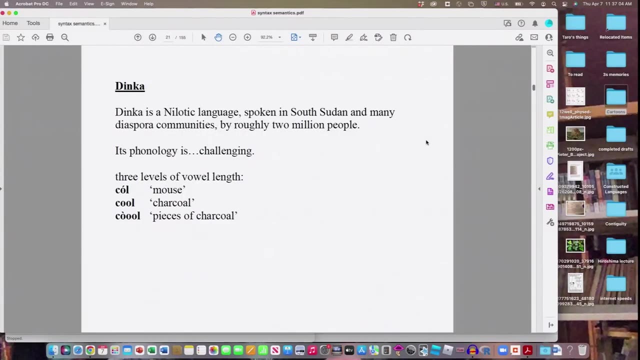 We'll see whether this works or not. So it has long and short vowels, which itself is not all that unusual, but it has three different levels of vowel length. So there are short vowels and long vowels and really really long vowels. So here are three minimal triple. 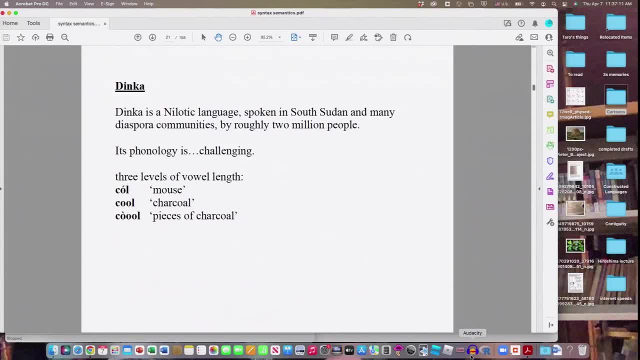 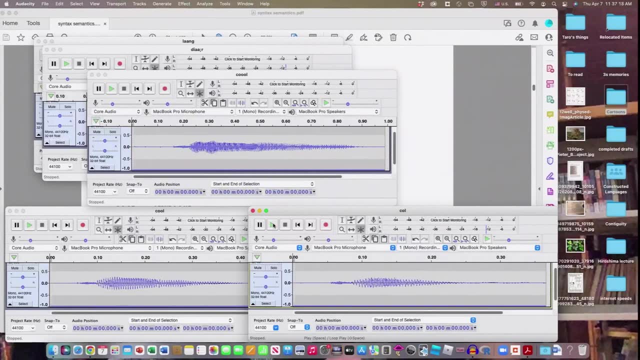 You've got mouse and charcoal and pieces of charcoal, the singular and plural. So here's the word for mouse. Let's see if I can play it so you can hear it. No, I can't. Oh, I think I know what happened. 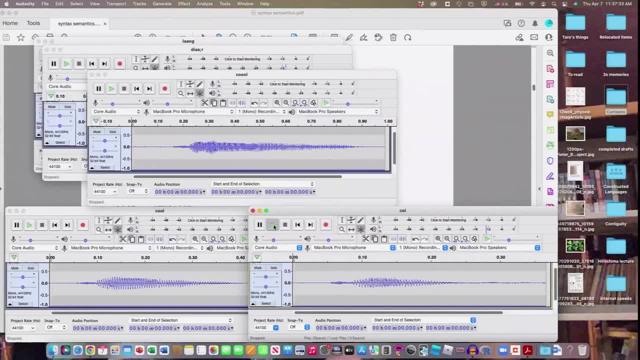 Okay, I will put these here. Okay, if people will be quiet, they may be able to hear this. All right, And here is the longer version. That's a longer vowel, And then we also, somewhere around here, have a really long. 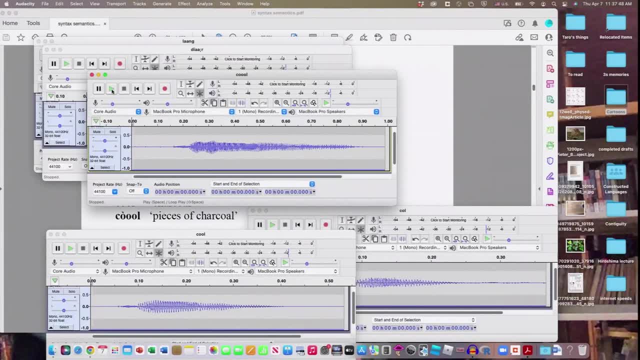 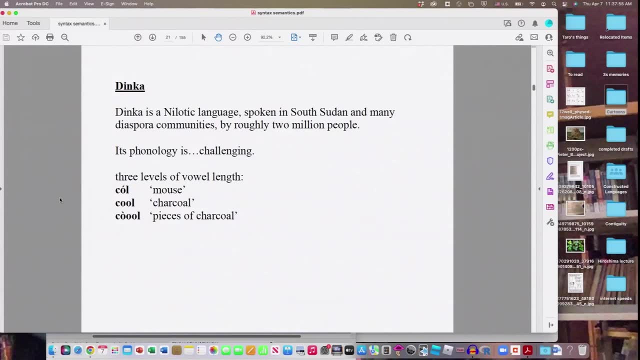 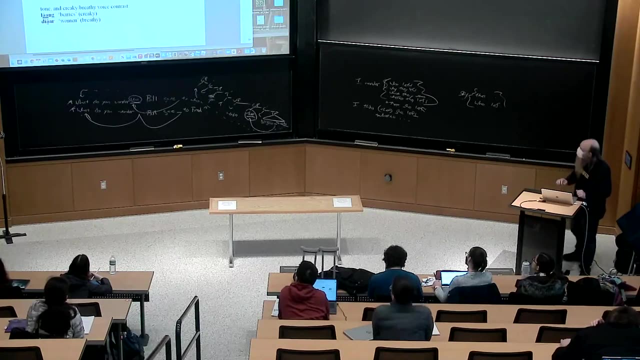 vowel: Yeah, there, I'll put those sound files on the website so that you can hear them. Basically, the word for mouse is Joel, The word for charcoal is Joel and the word for pieces of charcoal is Joel. It also has tone and it has a contrast. 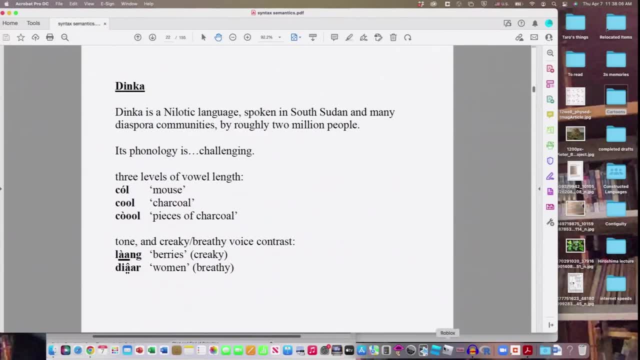 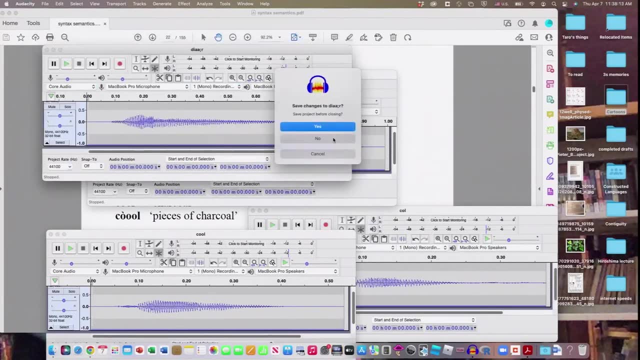 Between what are called creaky and breathy voice, And I'll play those sound clips for you as well. Actually, here, Let's see if I can get this to work. No, no, no, no, no, no. 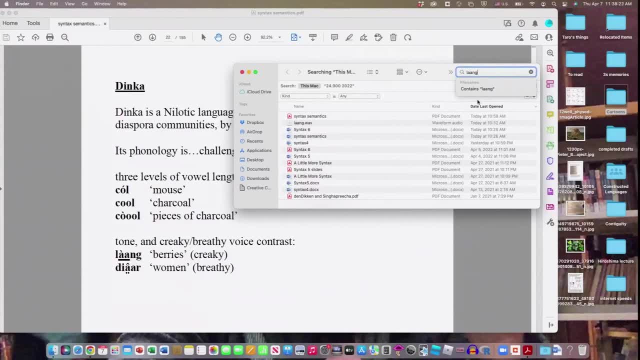 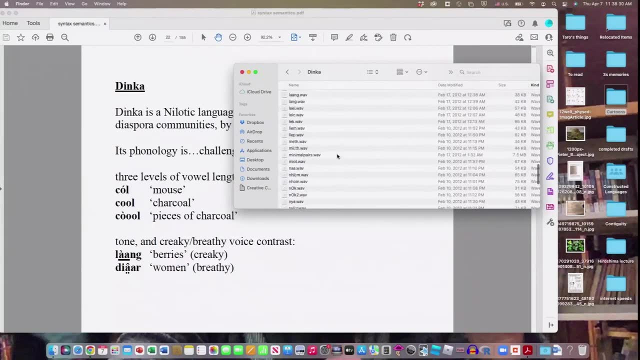 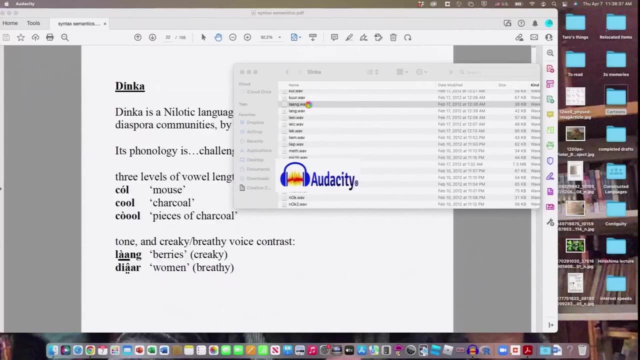 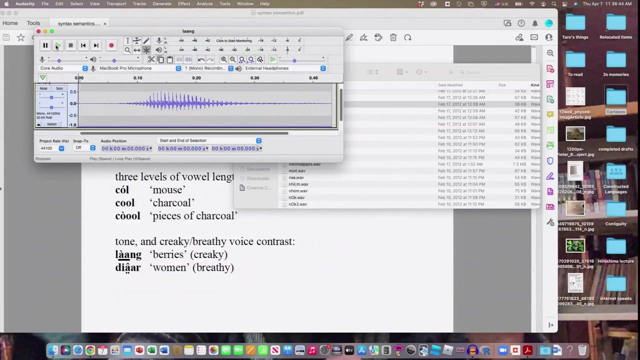 Sorry, Yeah. Theory is this was not working because I didn't have it plugged in when I opened the program. Let's see whether that's true. Okay, so that's creaky voice. That's the word for berries. Here's the word for women. 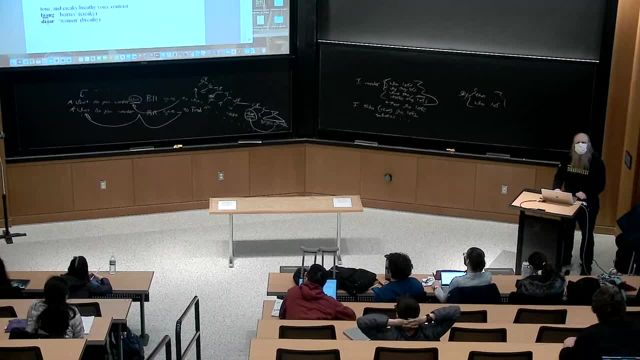 Yeah, okay, Yeah. so you do fancy things with your vocal cords When you speak this language. you either have to have. it has. Different dialects of Dinka have different numbers of voice qualities, But in this dialect there are two. there's creaky voice, where 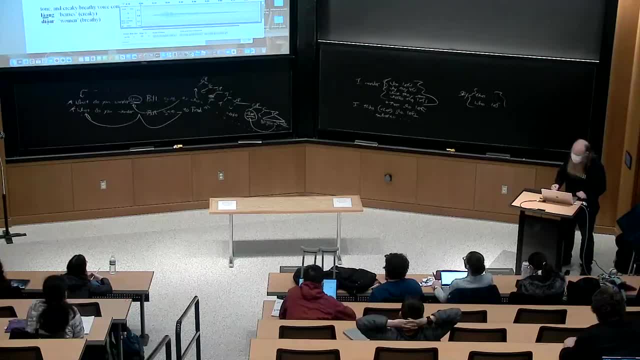 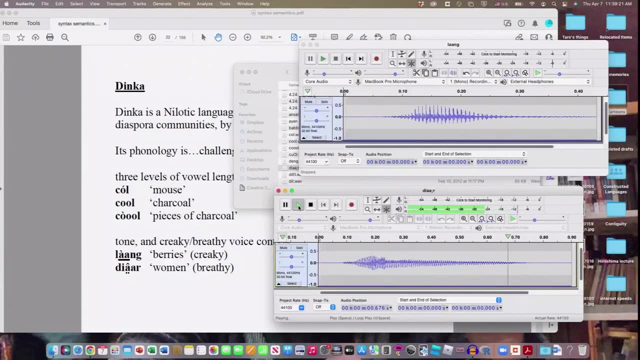 your vocal cords are under a lot of tension, I guess, as you're as you're speaking. So that's the word for berries. Here's the woman. word for women, Yeah, where the voice is breathy. There's actually a more minimal pair in here somewhere. 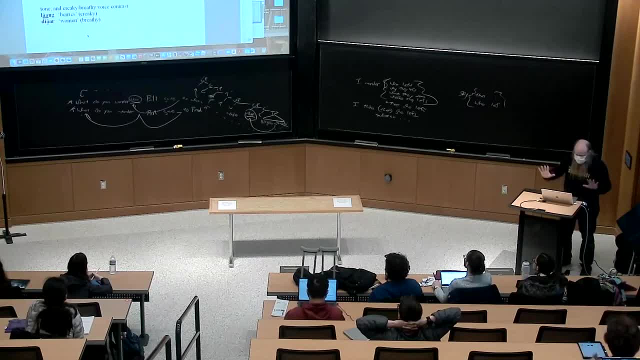 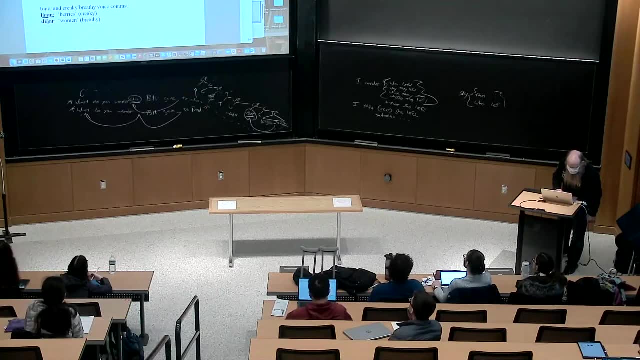 But I'm not finding it. Okay, nevermind. Okay, So that's what Dinka sounds like. It is lots of fun to try to study, partly because a lot of its morphology is tonal, involves changes to tone or to creaky or 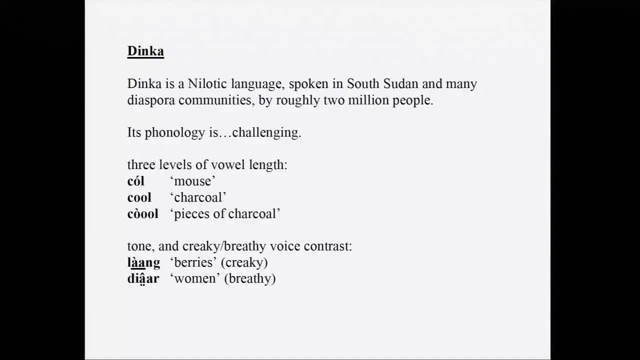 breathy voice or develop length. So you can see, for example, that the word for charcoal forms its plural by lengthening the vowel, which is already long, and also making it low tone, So it changes from total to Joel. We were. we lived in fear that we were missing half of the morphemes. 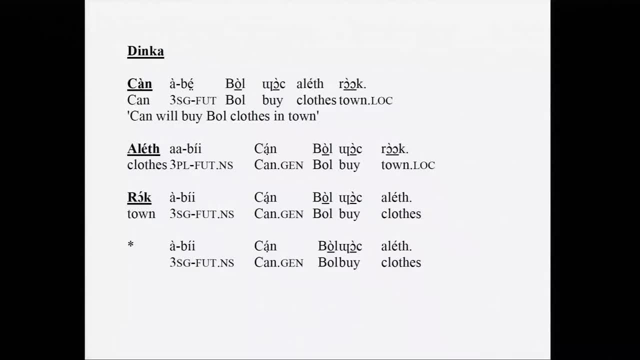 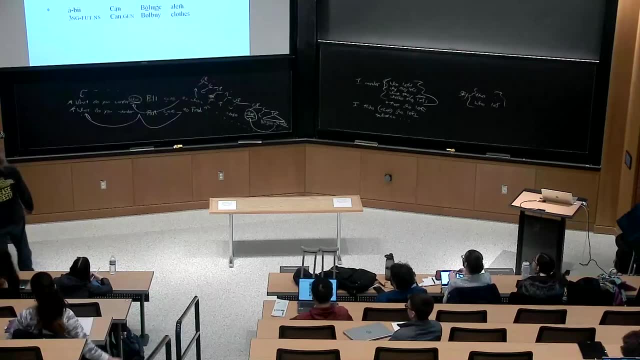 Okay, so that's enough about Dinka phonology. Let me tell you some things about Dinka syntax. Dinka is a v2 language, So see some examples here. If you want to say things like: Chan will buy ball some clothes in the 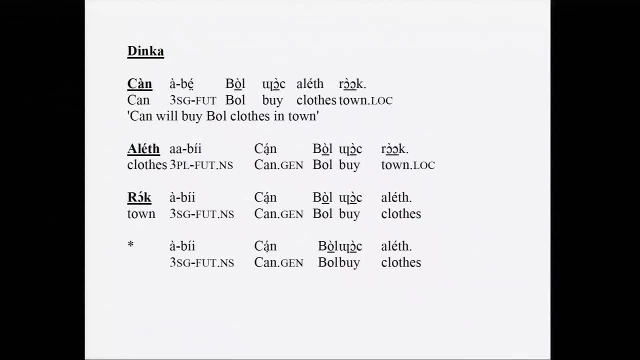 town. There's a position at the beginning of the sentence that has to get filled by some phrase. that can be filled by John, or by town, or by clothes. right, You can pick any of these things and move them into the first position. That phrase is then followed by an auxiliary, and all of these. 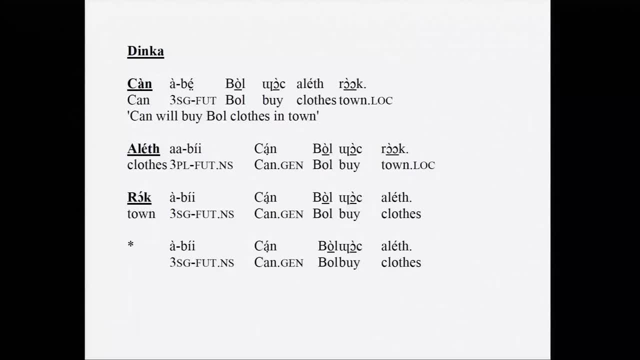 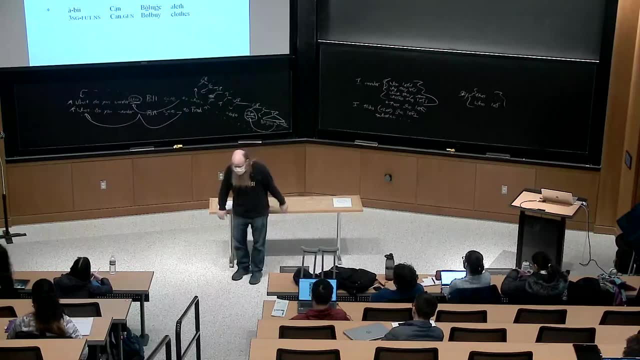 examples: If there isn't an auxiliary, then you get the verb in that position and then you have the rest of the sentence. Dinka is unlike German in one or two ways. German doesn't have creaky and breathy voice for one thing, but also the verb in German. 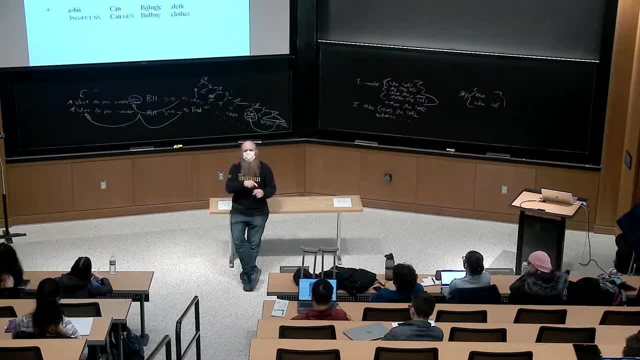 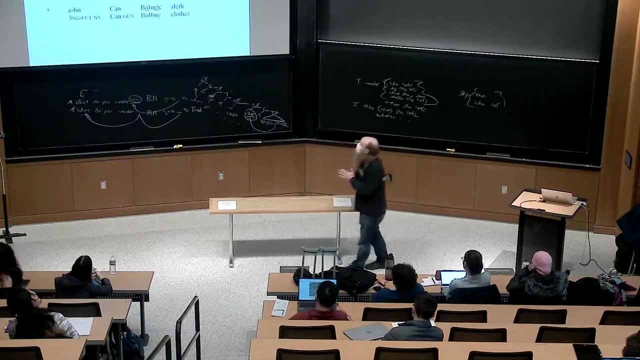 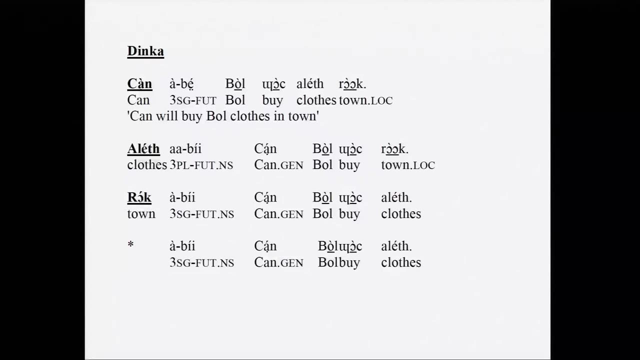 We saw, goes at the end of the verb phrase. The verb in Dinka goes earlier in the verb phrases. It's head initial. It's followed by its compliment, with some complications as we'll see. so you can say John Will bowl by clothes in the town. or you can say clothes will John bowl. 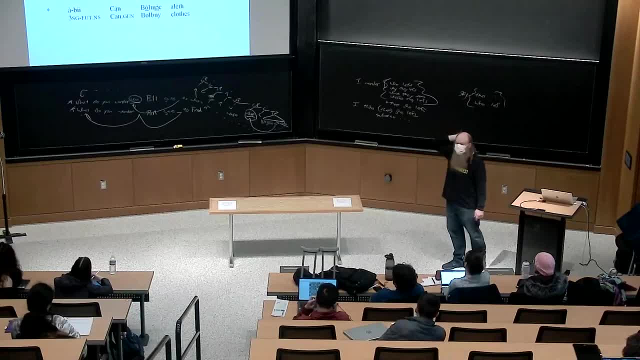 by in the town, or you can say town. You can take any of these phrases and move them into first position. Dinka is also different from German in that there's a morpheme in Dinka that tells you the number of the thing you've put in first position. 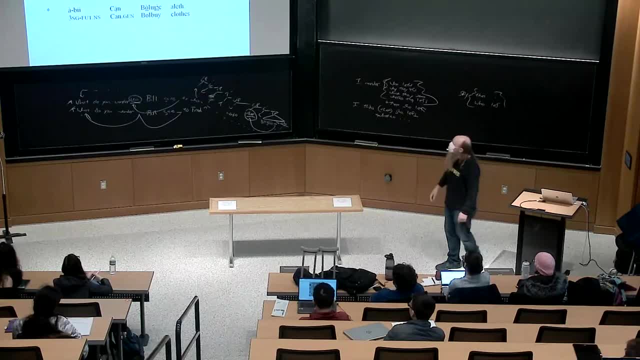 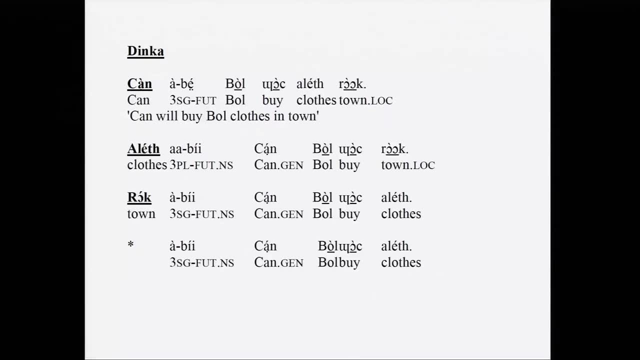 So you can see that the auxiliary in the first and the third examples starts with a, and in the second An example starts with a. so the a in the second example is indicating that the clothes are plural. the thing in first position is plural, So German doesn't have that. there are other alternations that you can. 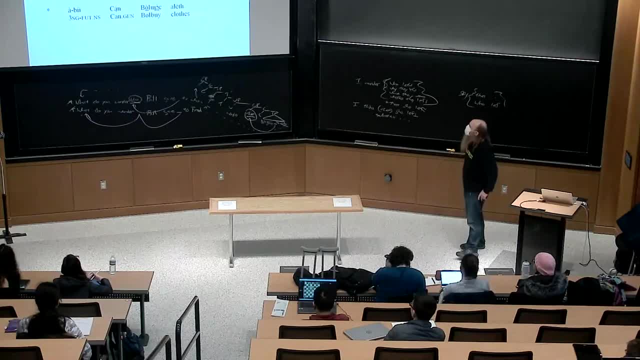 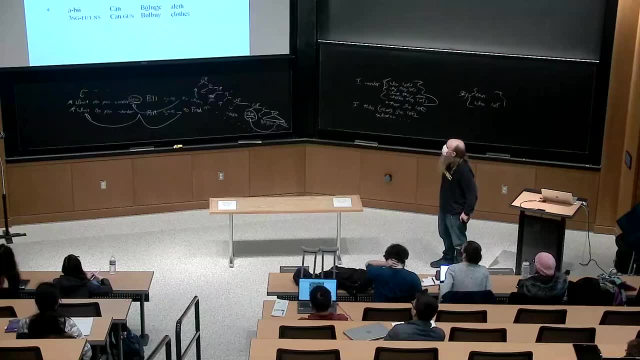 see there, which I won't, I won't try to talk about. Oh well there, so you can also see there's a difference between the auxiliary in the first example, which is that tells you that the thing in first position is the subject, whereas the auxiliary in the second. 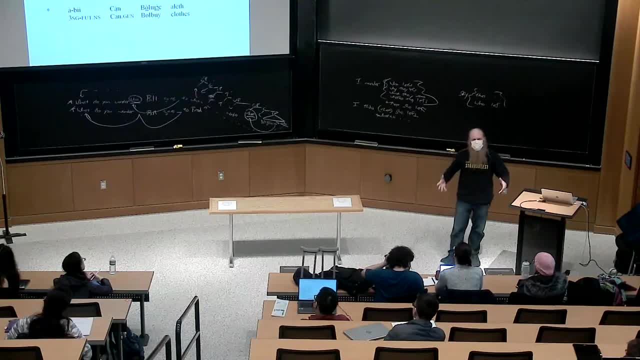 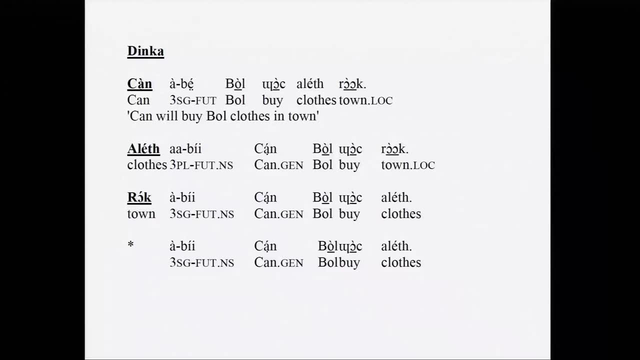 and third examples be is telling you that the thing in First position is not the subject. So there's all this morphology and you can see it's tricky to tricky to keep track of. Okay, So it's V2. the last example sort of demonstrates this. so it's ungrammatical. 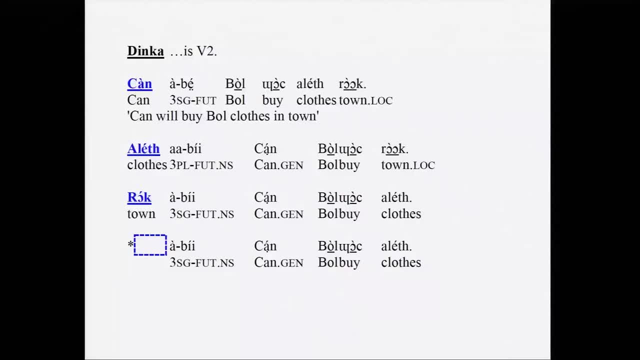 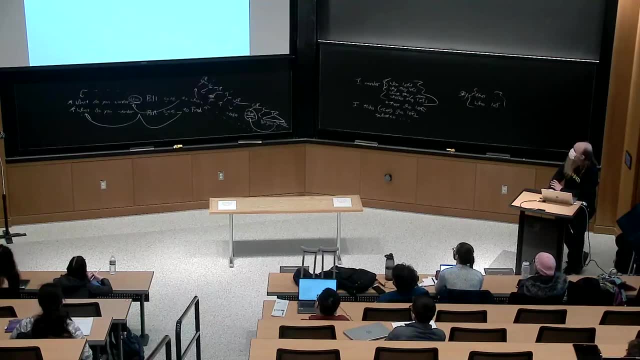 to just have nothing in first position. You have to put something in first position. Okay, V2 language. Now there is another position in the Dinka clause that has to get occupied. So if you want to say: in Dinka, I saw a giraffe. 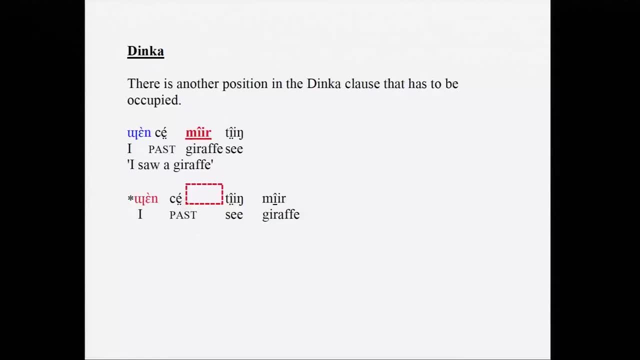 You can say: and to me a team, No, sorry me a team, So see is breathy, You've got I. the word for I, in first position here is satisfying the V2 requirement and throughout I'm going to make things in the V2 requirement. 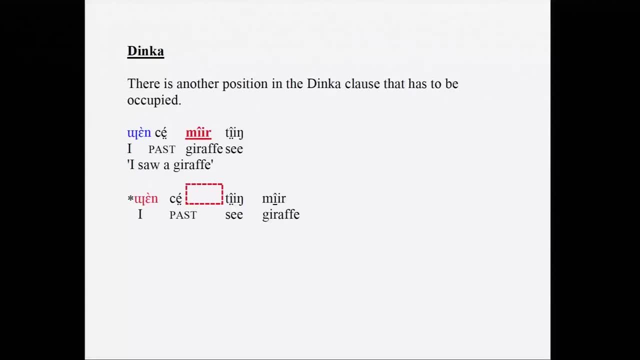 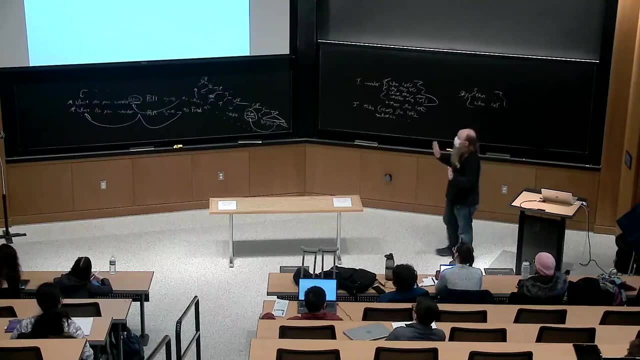 things in the specifier of CP, things satisfying that need for there to be something in first position. I'll make those things blue. There is another position that has to get occupied though. So you can say I Auxiliary giraffe saw. that's how you say I saw a giraffe. 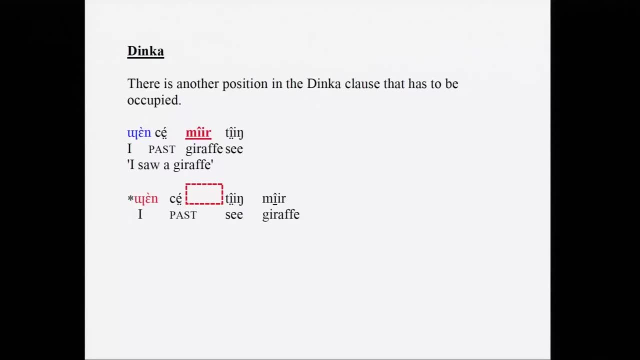 You can't leave giraffe after the verb If you. basically, the generalization is that if there is a deep, an NP object, the NP object has to go before the verb. everything else goes after the verb, but the NP object goes before the verb. 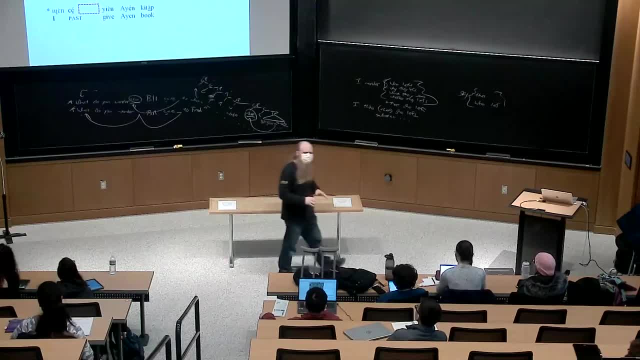 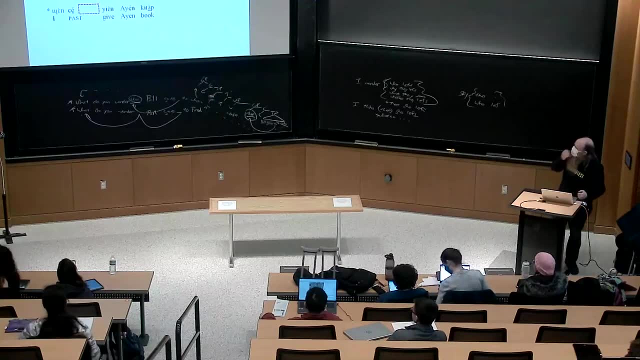 So there's another position down there. I won't try to talk about how we figure out where that is in the tree. That won't matter for what I'm about to show you, but I want you to know about it, Partly because it'll make things slightly less confusing. 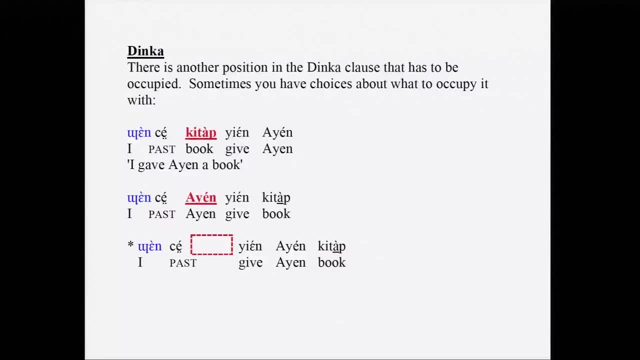 I hope if you have two objects you say things like I gave I in a book. You can choose either of them to go in first position. So you can say either I have a book, given I n, or I have a yen, given the book. 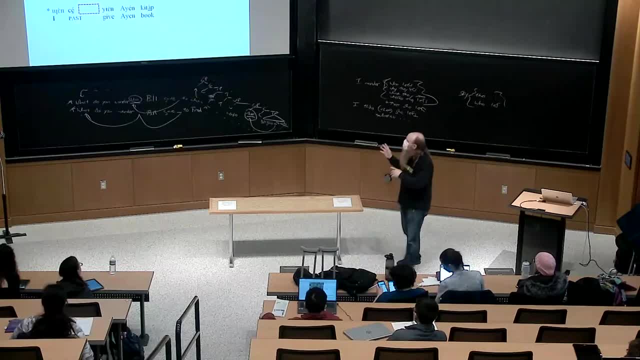 One of those two objects has to go before give. you can't leave them both after give. I don't think I have this anywhere on the slides, but you also can't put them both before give. Okay, so it's a V2 language. 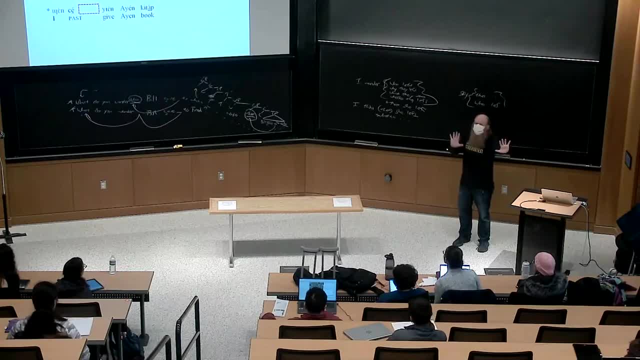 Something has to be in first Position and there's another position right before the verb. that also has to get occupied if there is a noun phrase object. if there is no noun phrase object and nothing goes in that second position, Okay, that lower position, the red position, 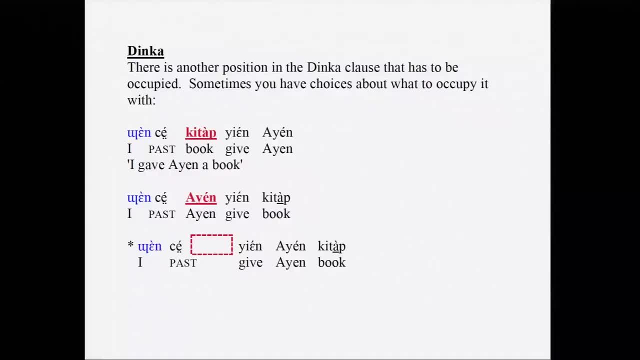 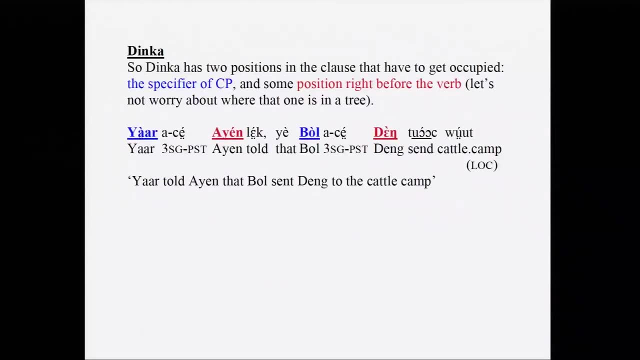 Okay, so far This is all set up. So Dinka has two positions in the clause that absolutely have to be filled. There's the specifier of CP, right, So it's a V2 language. the blue position, The position at the beginning of every clause, has to get filled by some phrase. 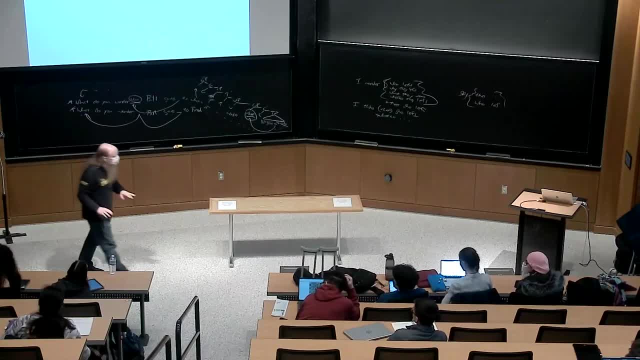 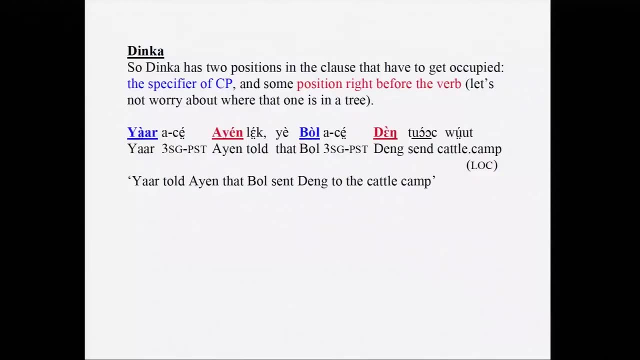 and dink is V2.. So it can be filled by a variety of different phrases. And then there is another position that's right before the verb that also absolutely has to get filled. So if you say in Dinka, you are told I in that ball sent down to the cattle camp. 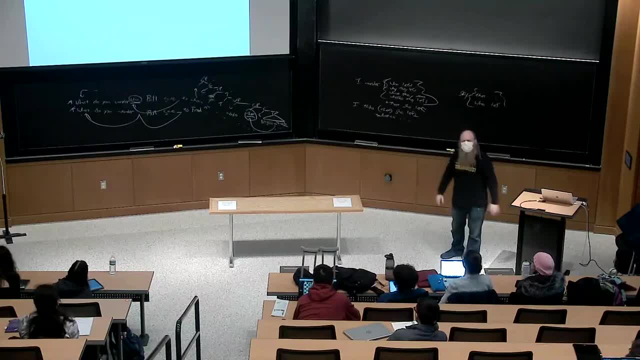 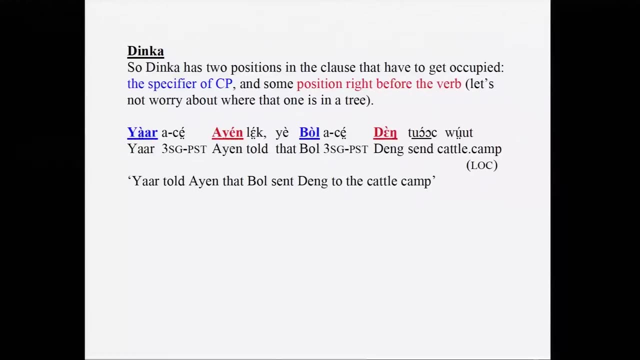 cattle camp is where the cattle are. young people go to the cattle camp. our consultant told us that the cattle camp is where young people get to know each other. So men and women mostly don't mix, But at the cattle camp then they do. So yeah, and I in trying to remember yard and I in our women's names and ball and 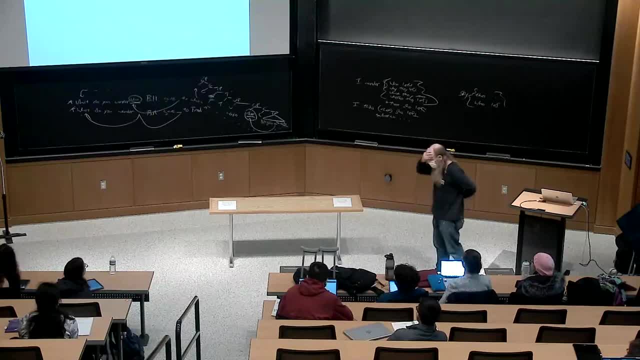 dang, or men's names ball. I think ball means person who is born after a set of twins. It's apparently a really common name: twins. I guess you're really common among the Dinka I in is a name for a color like a. yeah, anyway, 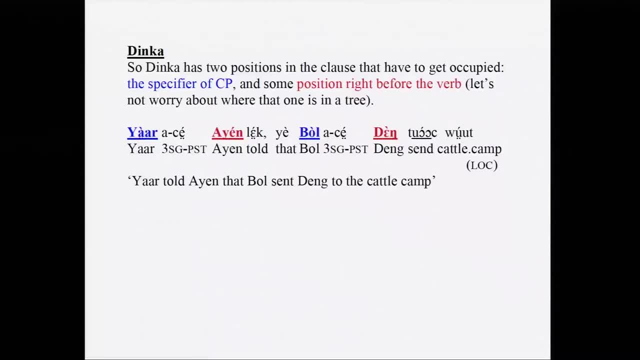 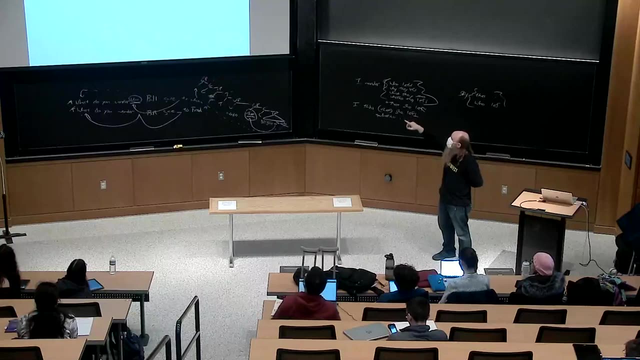 Okay. So here's a sentence: the main clause and the embedded clause both have their subjects in the first position. So you've got yard before the auxiliary in the main clause and you've got balls before the auxiliary in the embedded clause. Yeah, and in the main clause you've got I in the person who's being told going. 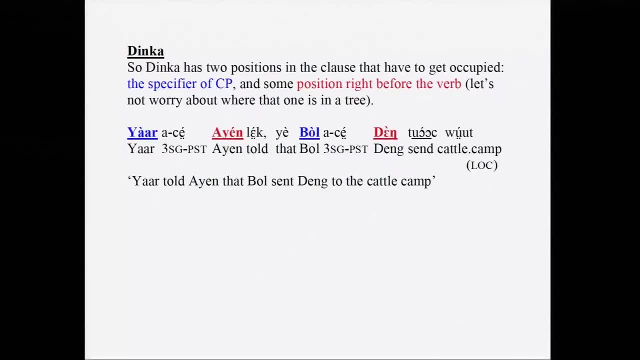 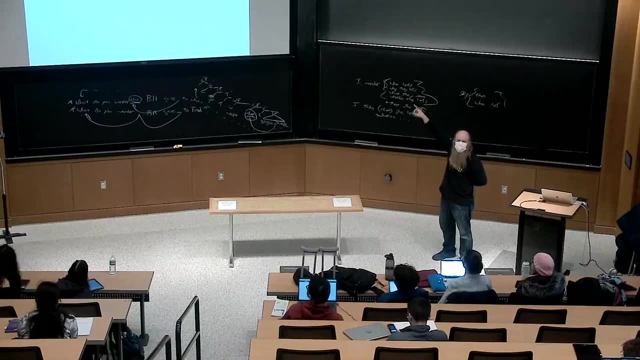 before the verb told right, filling that red position. and in the embedded clause You've got dang: the person who's being sent. Preceding the verb following filling that red position. Okay, so far. So now you know a little bit of Dinka. 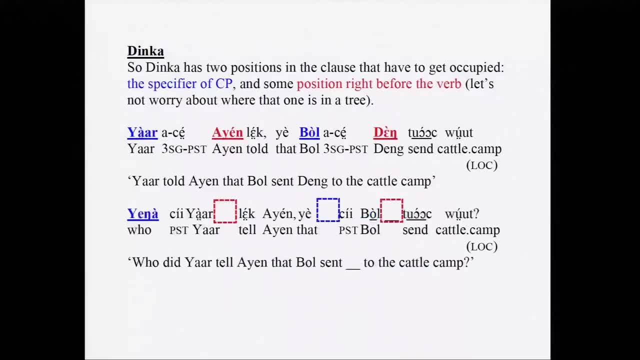 Now Here's the thing: If you wh extract, So suppose you want to ask who did yard tell I in that bowl sent to the cattle camp? So here we've changed dang into a wh word and we're going to move dang into the main clause, right? 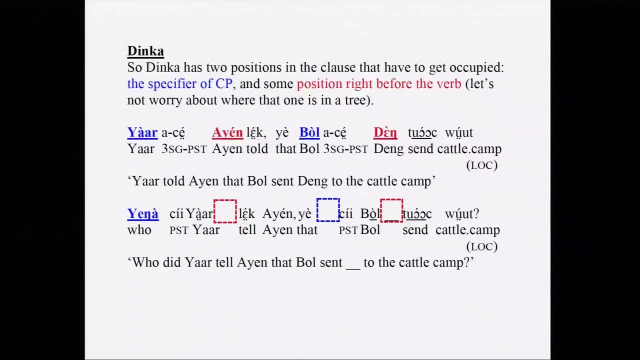 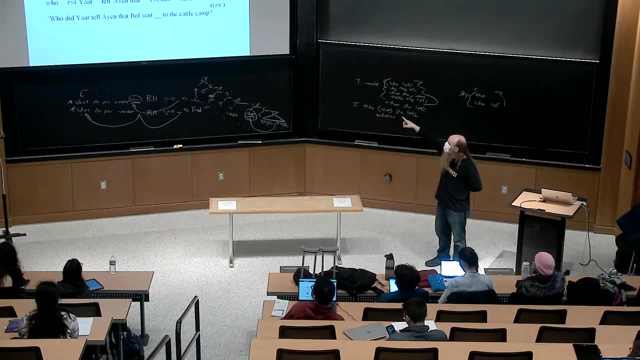 So the object of send is going to be a wh word and it's going to go in the main clause. the whole thing is going to be a question. Here's the observation: If you do that, all of those positions that normally absolutely have to be filled have to be empty. 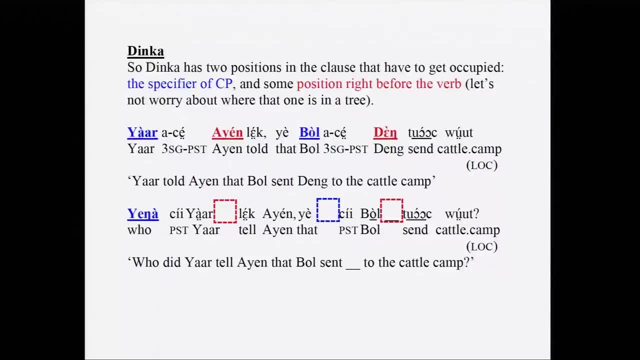 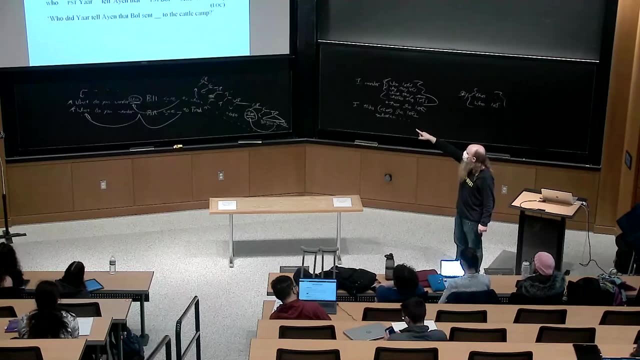 So who started off as the object of send? And so that rightmost red position, the one that dang used to be in, is empty. That's not so surprising, That's where who came from. But what's interesting is that the blue position right 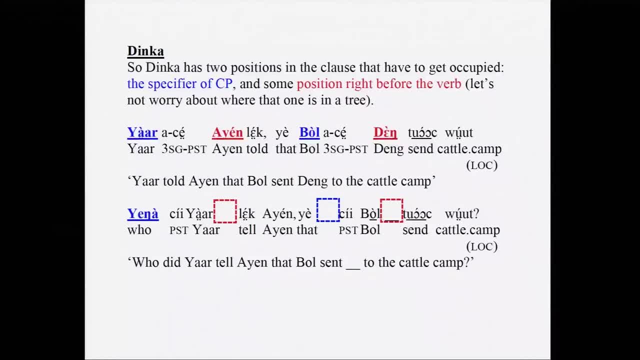 above that, the one before the auxiliary of the embedded clause, the one that was filled by bool in the first example, can't be filled by bool. Bool has to not be there anymore. And similarly the red position before tell, the first red position in the second example. 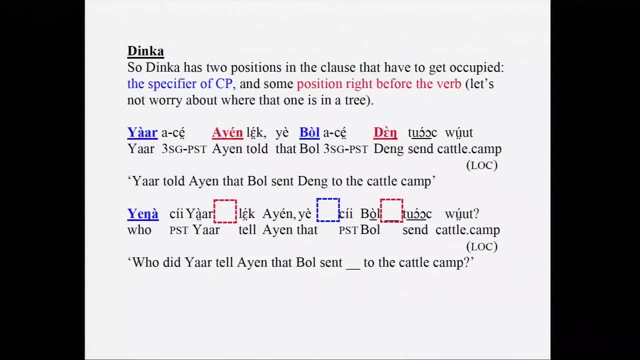 there, the one that's an empty box has to be empty. Normally it would be filled by in. That's what's being filled by in the first example, But if you wh move across it it has to be empty. So these positions that ordinarily absolutely 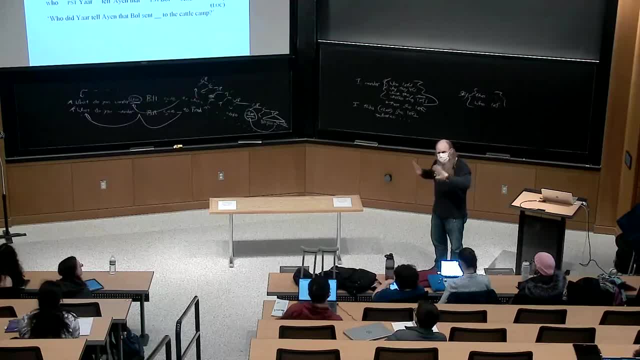 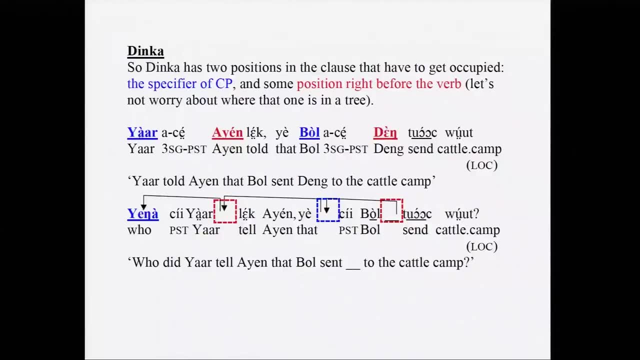 absolutely have to be filled, cannot leave them empty Suddenly. they have to be empty if you're moving a wh phrase across them. Well, we can understand why. if we're willing to believe in successive cyclic movement. So you just have to be willing to believe. 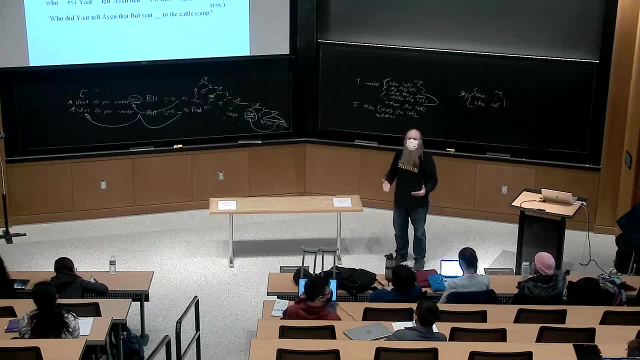 The wh movement is obliged to move, not in one mighty leap but in a series of little hops. It has to land And all of these open positions, And that's why they can't be filled the way they normally would be if you're doing long wh movement across them. 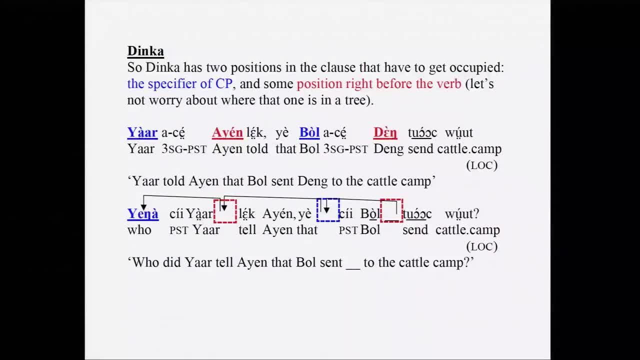 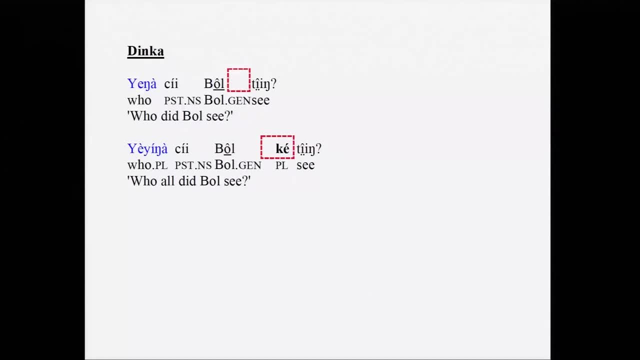 So there's an explanation for why these positions are emptied out. I'll show you one other cool thing about dinka, And then I think we're done with dinka. Dinka has a distinction between singular and plural versions of wh words. So there's, which is the word for who. 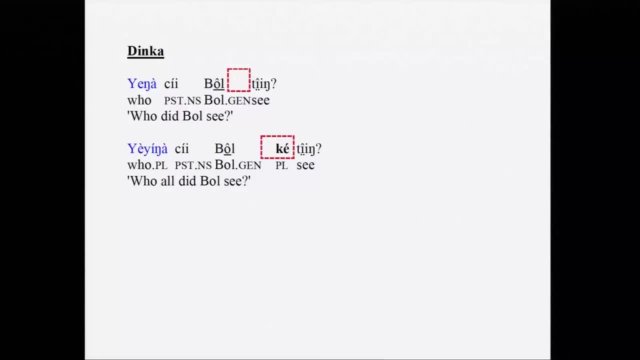 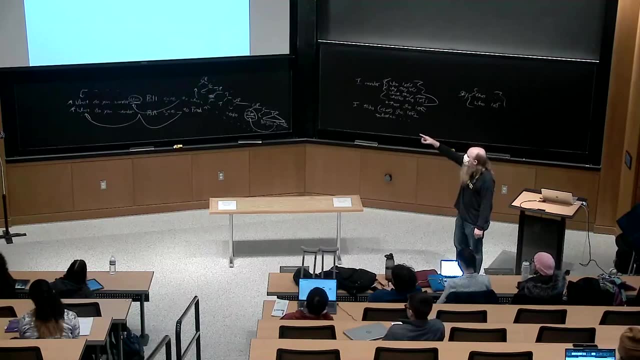 And then there's which is the word for who plural, who. all English doesn't have a word for who plural, but plenty of languages do, and dinka is one. If you ask a plural question, you put that who at the beginning. 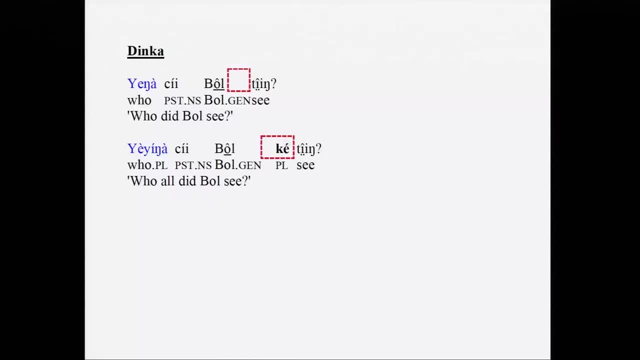 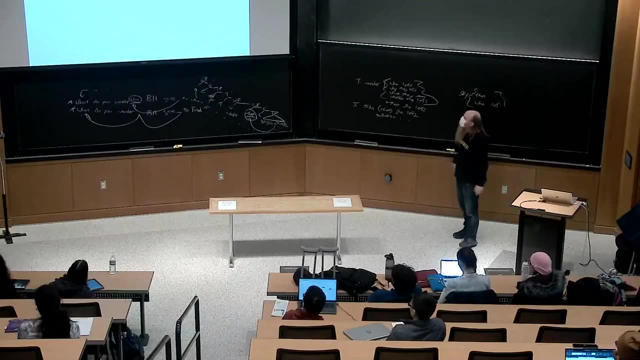 in the spec of CP of the clause that you're in, But you're required to leave behind the plural morpheme in the red positions, the positions before the verb. So who all did bol? si, Yeah, you've got this. who plural in first position. 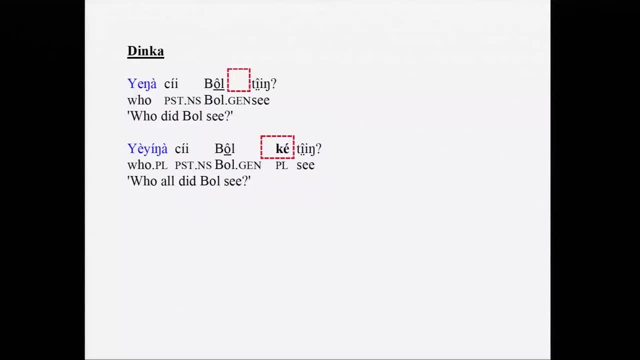 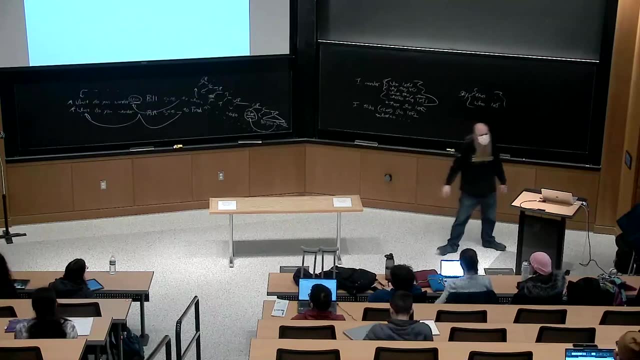 But you've also got this ke that goes in the red position, The position that's before the verb. If you wh extract something from the verb phrase like an object, you have to leave this plural morpheme behind. So interesting fact if you do a longer question than that. 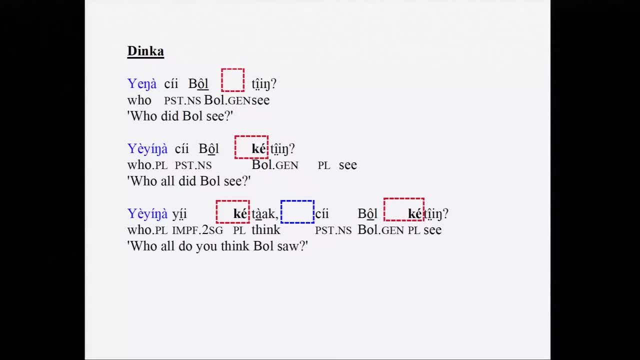 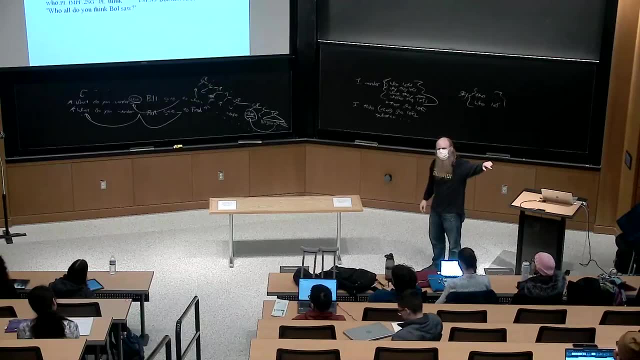 like who all? do you think that bol saw? So you've got who plural at the beginning and you've got ke in both of the red positions. along the way As you wh move up the clause, it's like you leave behind this little. this was plural thing. 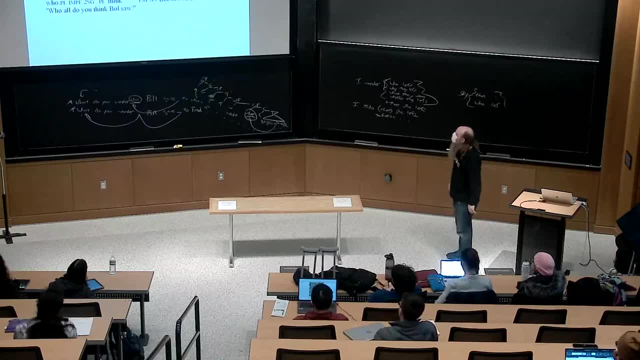 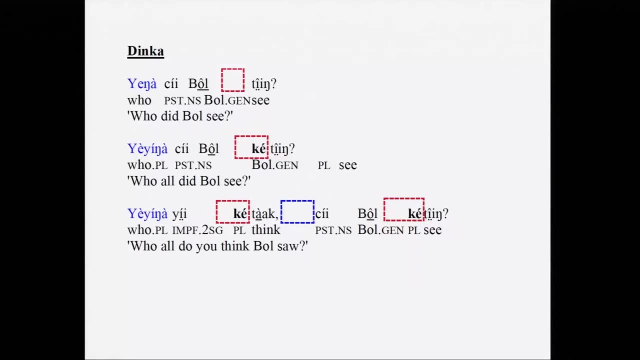 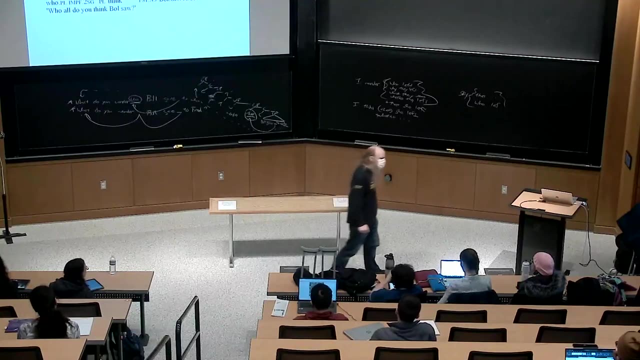 as you move along, So you get multiple ke's as you go up. Ke sort of resembles the third person plural pronoun, which is keek, So that's the word for they. So we figure it's somehow related to this. So Dinka gives us some evidence for this idea. 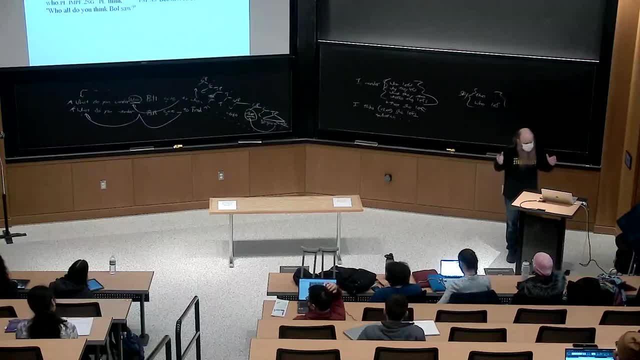 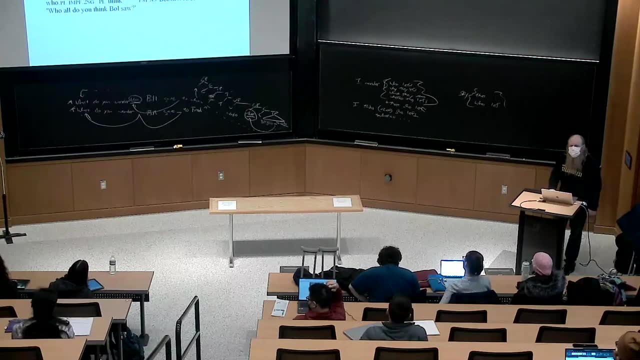 this wacky idea of Chomsky's from the 70s that wh movement has to be successive, cyclic, that it's not possible to just move in one big jump. Yeah, You have to move in a bunch of little hops. So Dinka has sort of a detector for landing in positions. 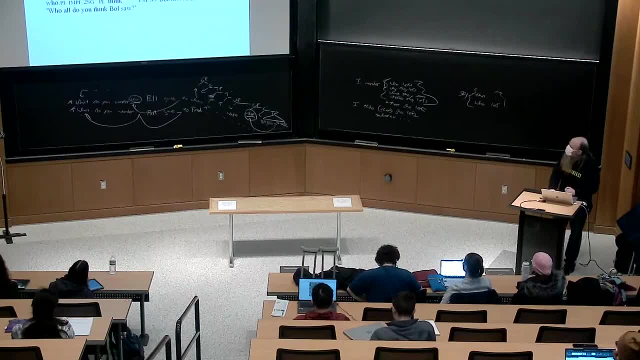 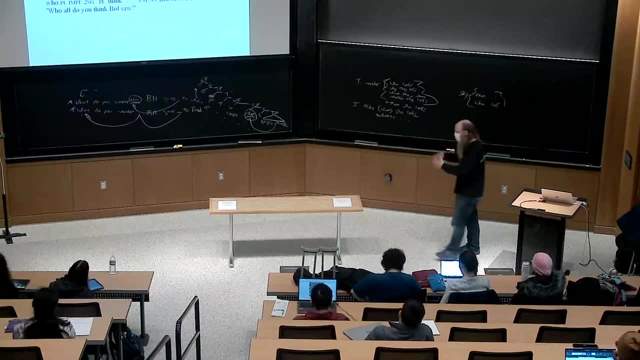 Two detectors actually. One is this ke thing and the other is just whether certain positions are filled or empty. So these positions that normally have to be filled have to empty themselves out if you're going to wh move through them by hypothesis, because the wh word is landing. 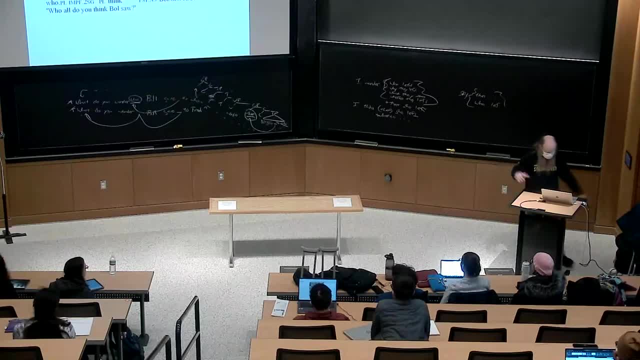 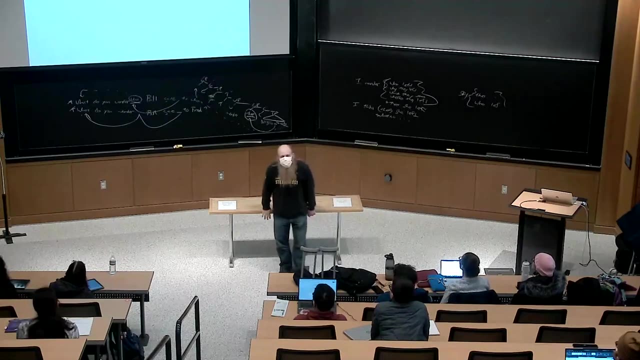 and moving on the way up. OK, One piece of evidence. There are zillions of pieces of evidence for this. This is one of my favorites. Yeah, OK, Now we are done with syntax. Let us have a moment of silence for syntax. 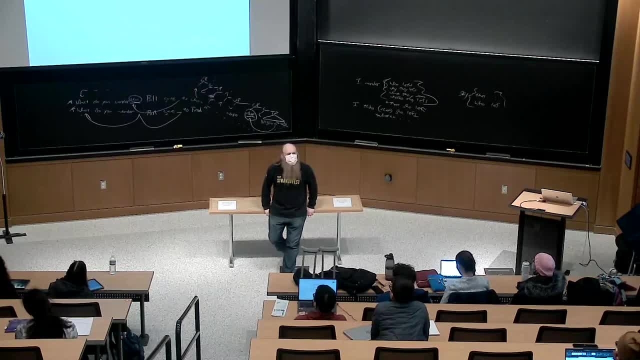 Does anybody have any questions about syntax? before we leave syntax behind and begin talking about something else? So if you are looking at the syllabus, there was going to be a day on dialects. I will move that day to the end of semantics. 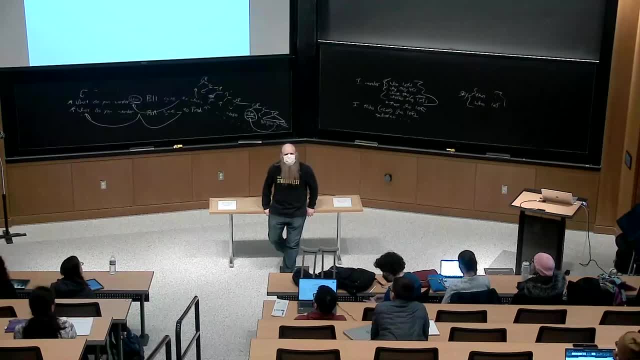 So we're now more or less caught up with the syllabus. We're going to spend some time doing semantics And then we will have kind of a grab bag of topics after we're done with semantics- various things. Any questions about syntax before we leave syntax behind. 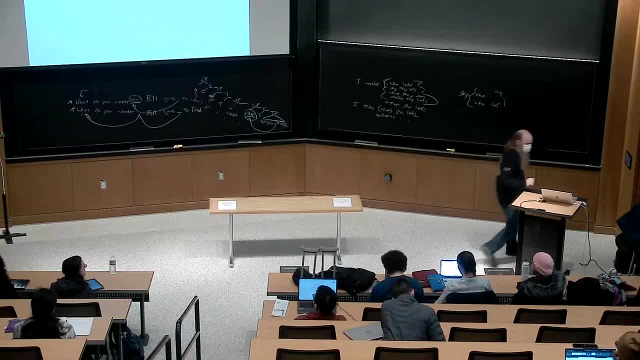 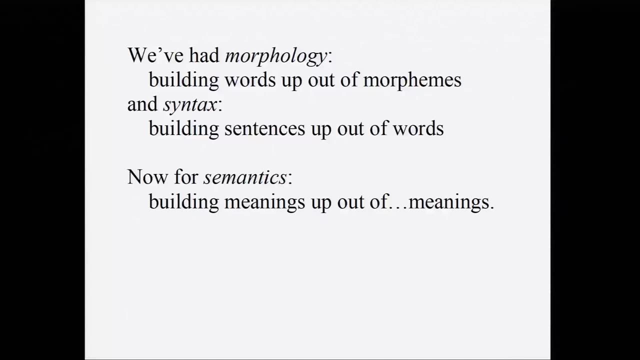 OK, All right, Let us start in on semantics then. So we've done morphology, which is the building up of words out of morphemes. We've done syntax, which is the building up of sentences out of words. We're now going to do semantics, which. 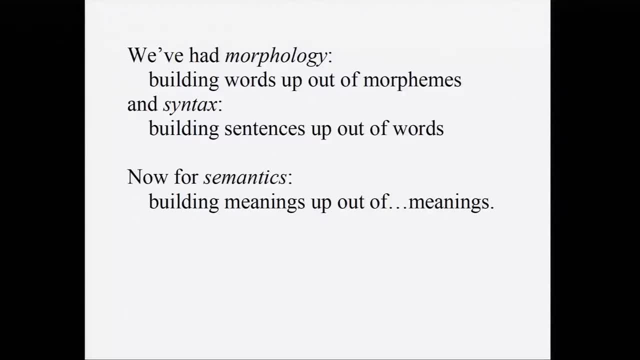 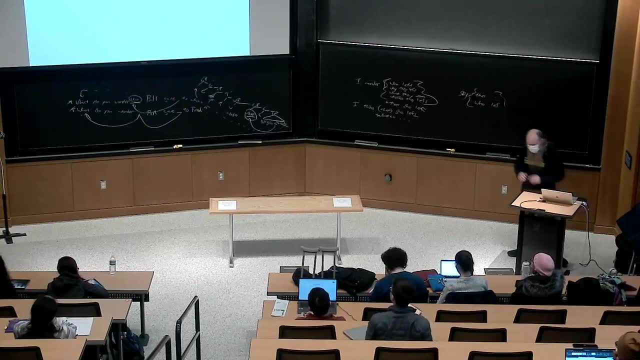 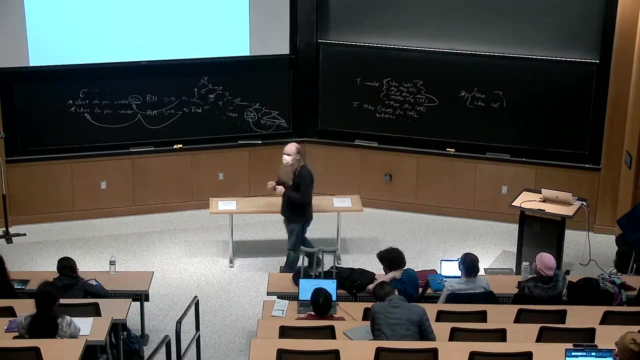 is the study of how you make meanings out of small, smaller meanings. That's sort of what semantics is all about. There's a going hypothesis, which is that something like if you completely understand the meanings of the various parts of the sentence, the various morphemes that combine: 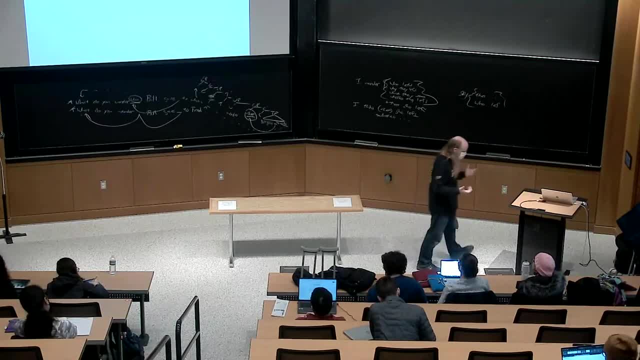 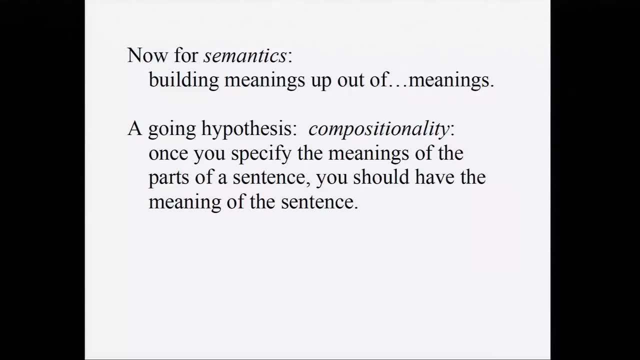 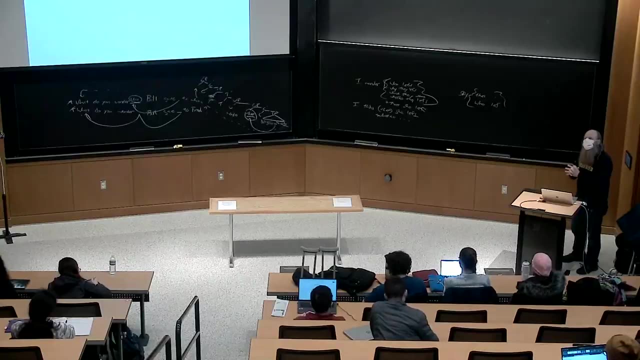 that there ought to be a simple set of rules for how to combine meanings. that would give you the meaning of the sentence. This idea is called compositionality. It's the idea that we should pay a lot of attention to specifying very completely what particular morphemes mean and that if we'll do that, 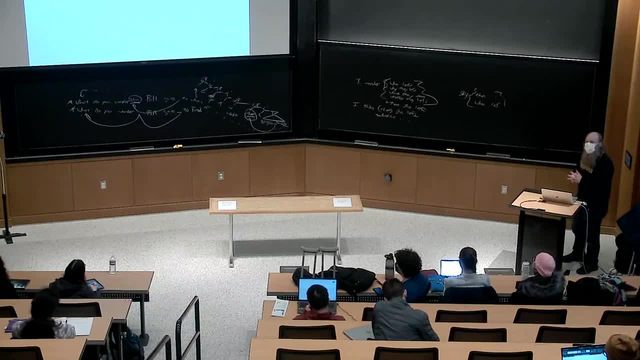 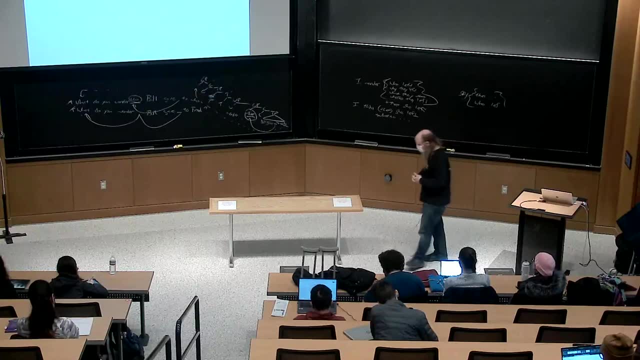 we can have simple rules to generate the meanings of sentences. So we're going to do some semantics. I'm going to introduce you to semantics, And semantics is going to be like the other topics we've talked about in this class, in that I hope to tell you enough about it to make it sound interesting. 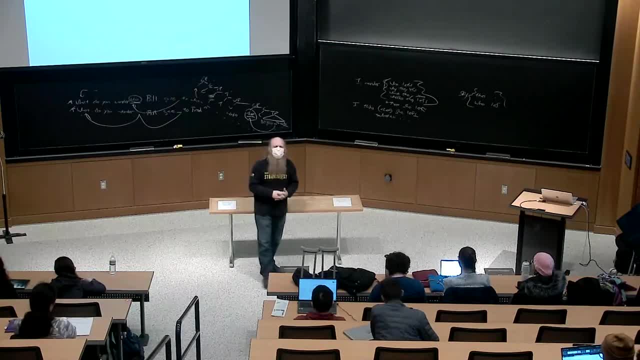 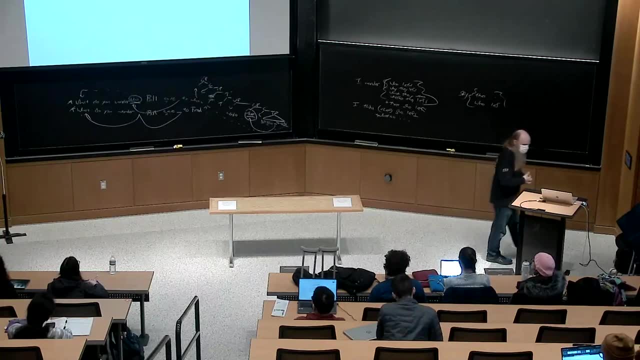 And then I will abandon you and let you study it on your own. Go, take. there is an undergrad intro semantics class that I encourage you to take if you find the stuff that we're going to talk about We're going to talk about interesting. 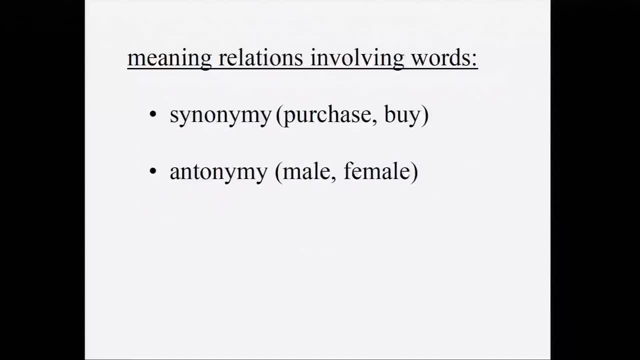 There's lots of interesting work in semantics, So let's talk about some meaning relations, some classics like meaning relations involving words. So we can say that words are synonyms if they seem to mean the same thing. So words like purchase and buy. 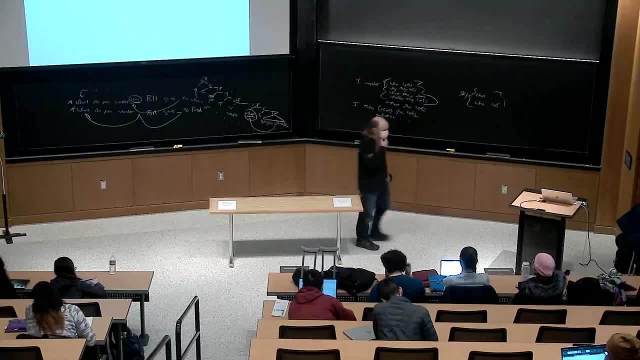 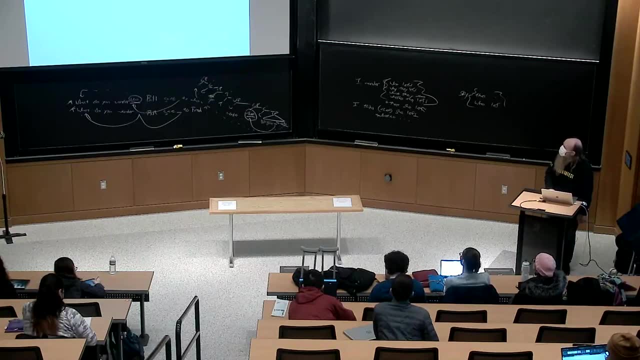 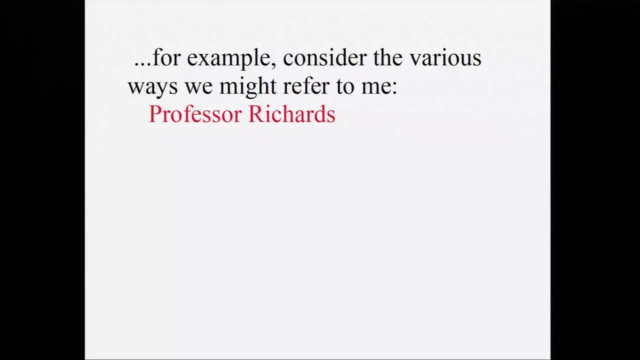 And that words are antonyms if they seem to mean opposite things. This is an antiquated example. I should fix this. so male and female. But there are fancier things to say. So let's consider the various ways someone might want to refer to me. 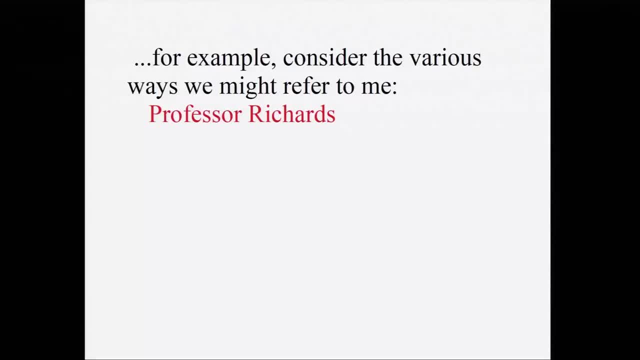 So people usually say at the beginning of the classes: doesn't matter to me what you call me. Some people call me Professor Richards or call me Professor. Some people call me Norvin, which is my first name, If you can't remember my name there. 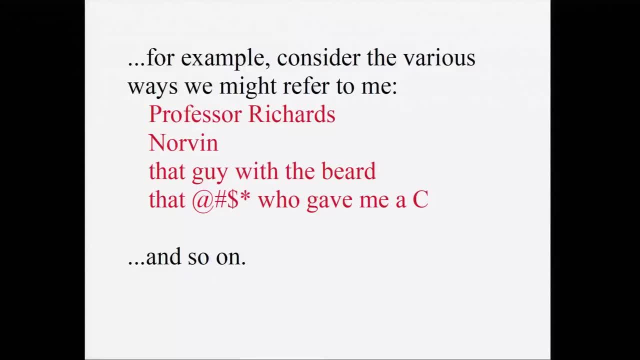 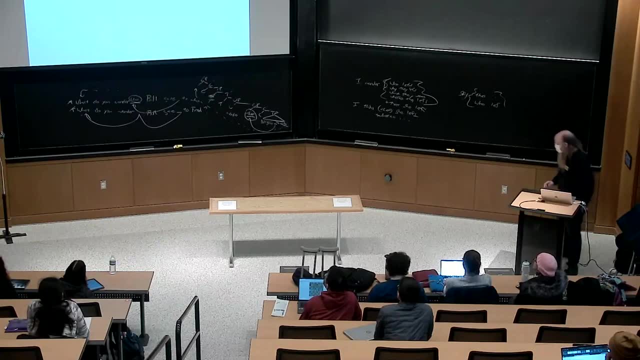 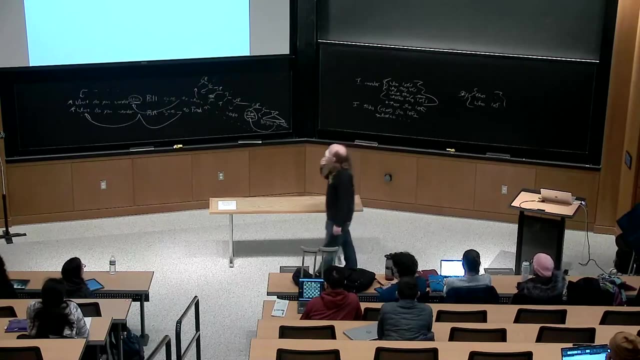 are other things you might want to call me, Variety of things that you might say about me, depending on circumstances, And to say that these are all things that you can use to refer to me is to say that it's usually true if you have a sentence. 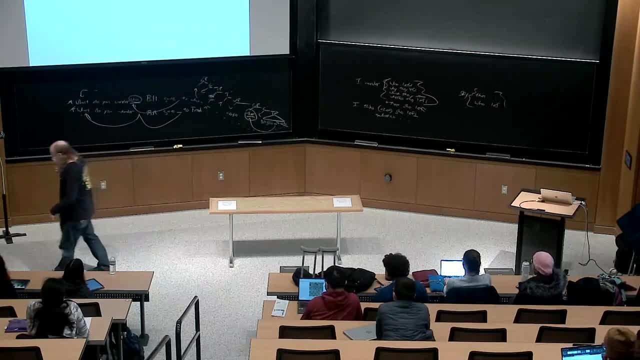 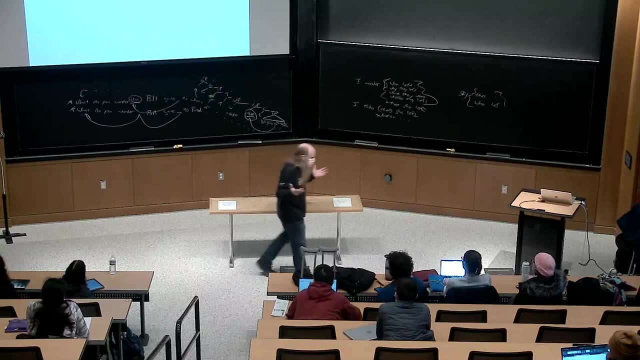 and it has one of those expressions in it. if you change just that expression to another expression, that the sentence, the meaning of the sentence, won't change. In particular, if it was true before, it'll still be true. If it was false before, it'll still be false. 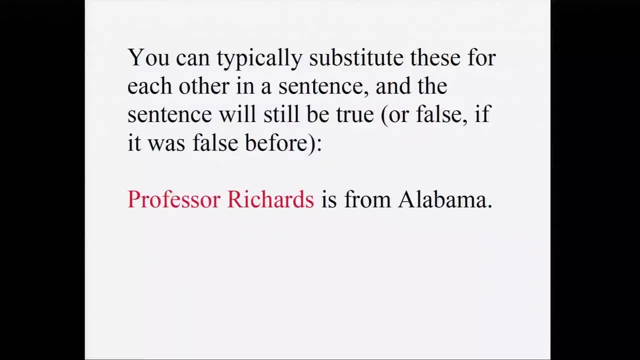 So here's a sentence: Professor Richards is from Alabama. Sentence is true, I am from Alabama And if you were to switch out the red expression for any of the other red expressions, the sentence would still be true. So to say that these all mean the same thing. 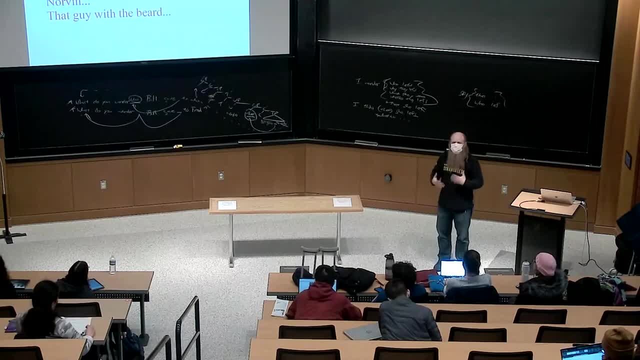 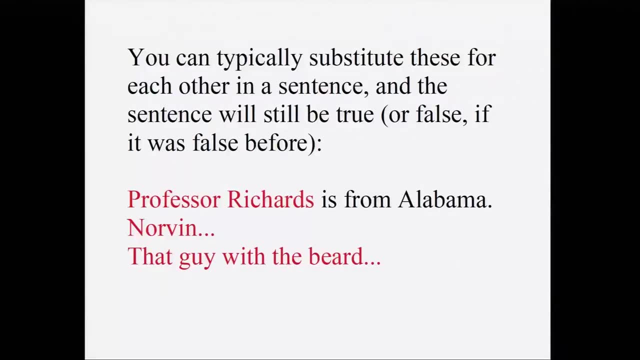 to say that Professor Richards and Norvin and that guy with the beard can all refer to the same person is to say that if the first sentence is true, then changing from one of these to another one is not going to change that. If it's false, it's not going to change that. 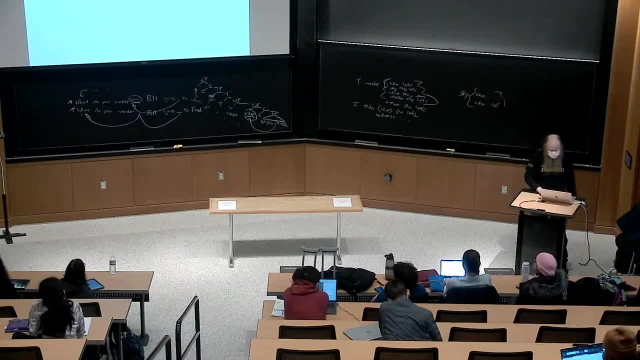 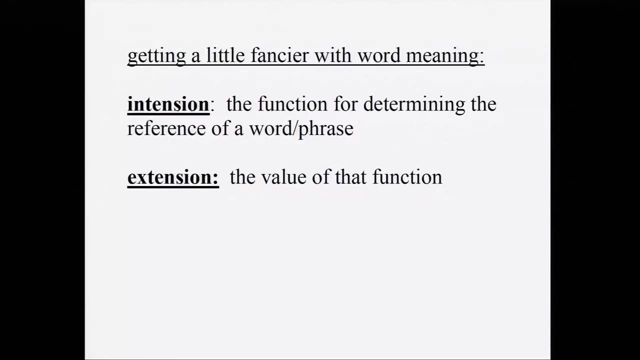 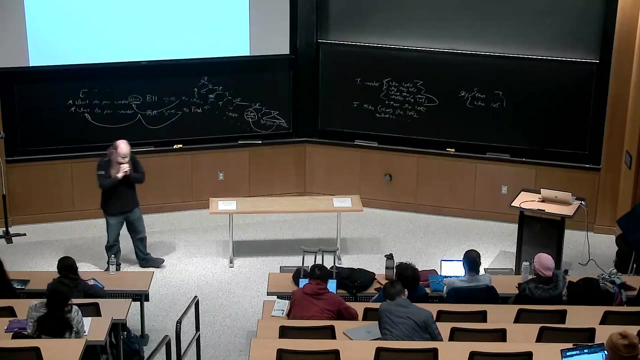 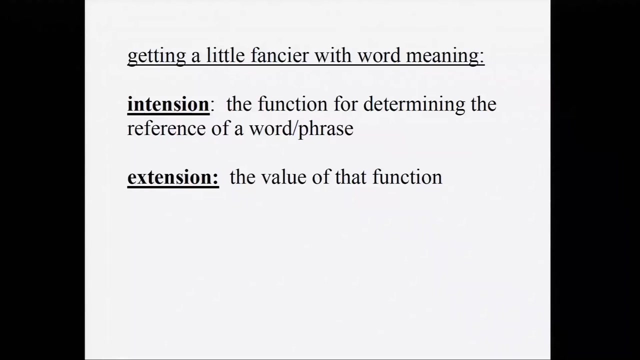 Sound right. We have to be careful, because it's possible to get a little fancier with the meanings of words and phrases. People sometimes talk about what's called the intention and the extension of the meaning of a phrase or a word, Maybe the easiest way to think about this, at least for me. 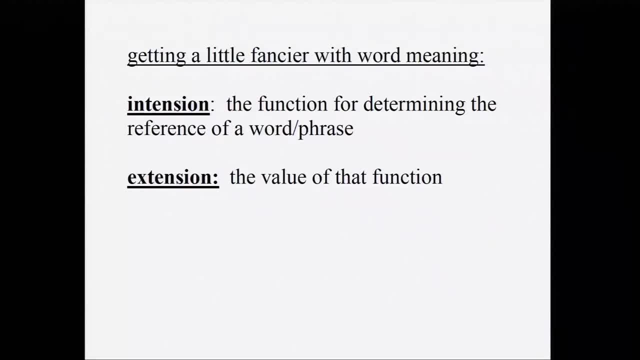 goes like this: The intention of a word. if you ask what the intention of a word is, what you're asking me for is sort of the intention. The intention is the procedure that you will use. I'm going to give you examples of this in just a second. 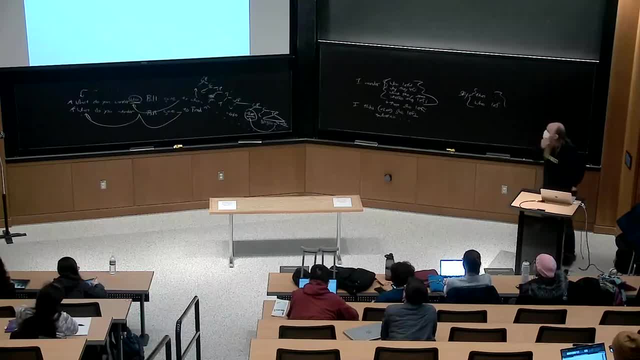 But the intention is the procedure that you will use to determine what that word or that phrase refers to, Whereas the extension of a word or a phrase is the value, the thing you will get if you apply that procedure, the value of that function. 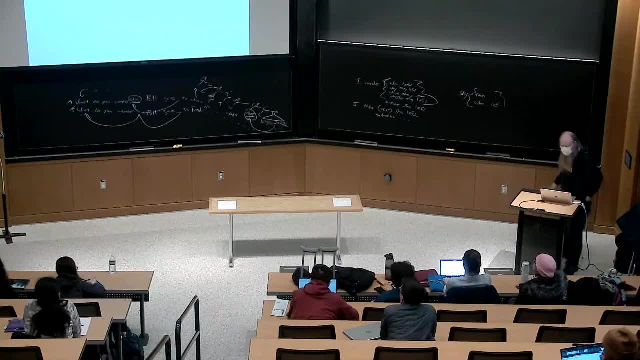 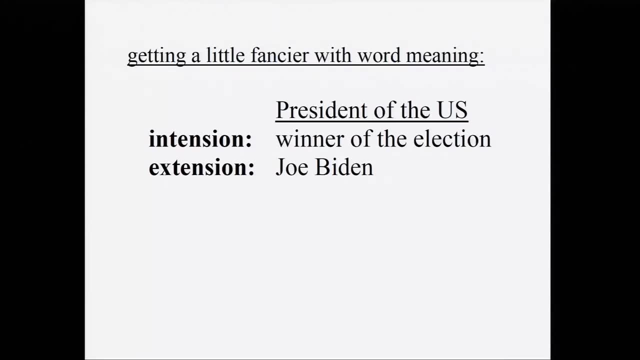 Let me show you what the heck I'm talking about. So the phrase the President of the United States has an intention and an extension. The intention of that phrase the President of the United States is sort of the procedure that you should use to find out who that phrase refers to. 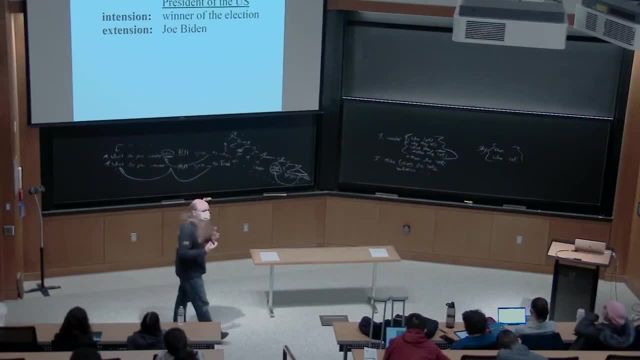 So what you should do is find out who won the election, who won the illustration of the election for President. That's the intention of that phrase. The extension of that phrase is well what you'll get if you apply that procedure, which, right now. 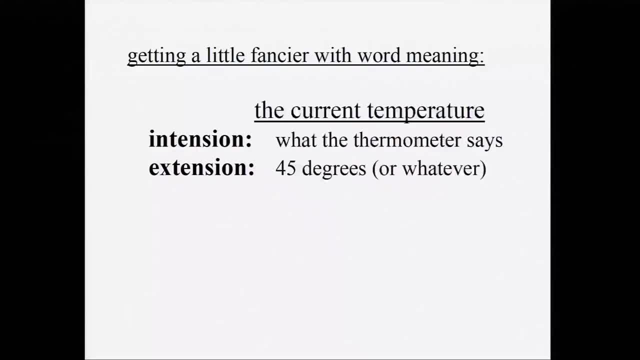 is Joe Biden, Or, similarly, the phrase: the current temperature has an intention and an extension. The intention is the procedure you'll use to find out what the current temperature is like. Go, look at the thermometer, go on to weathercom or whatever, and then it has an 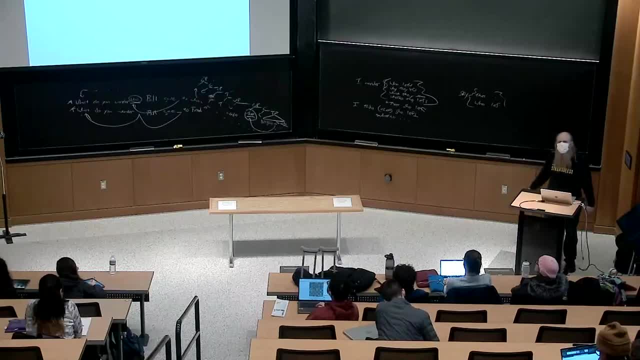 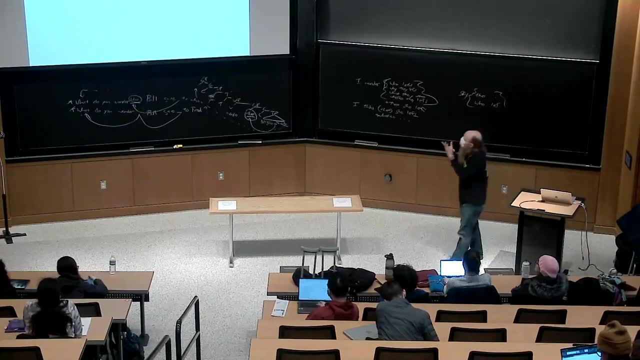 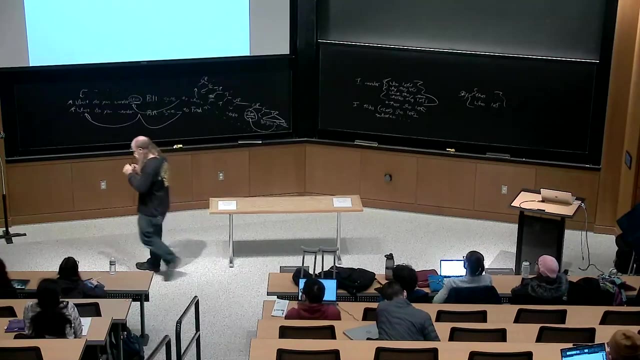 extension, which is well, whatever. it is 45 degrees, let's say So I said before, when we say that these phrases mean the same thing, to say, that is to say that you could take a sentence that's true and switch one of the phrases and 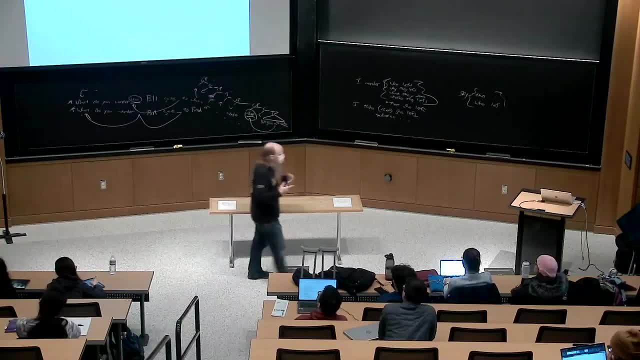 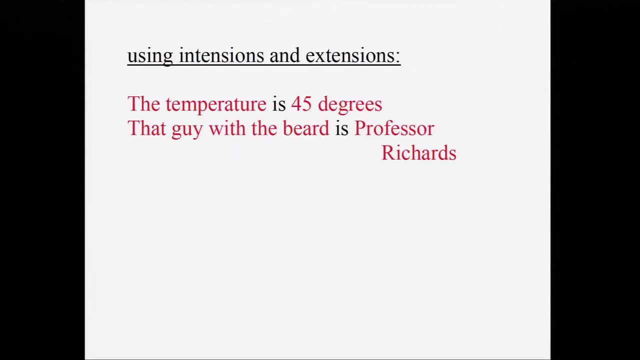 still have a sentence. that's true. We have to be careful, though, about things like intentions and extensions. So when we say the temperature is 45 degrees or that guy with the beard is professor Richards, it's true that that guy with the beard and professor Richards are mostly substitutable for each other, but 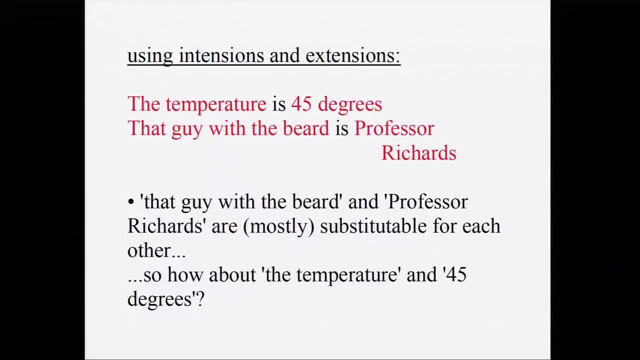 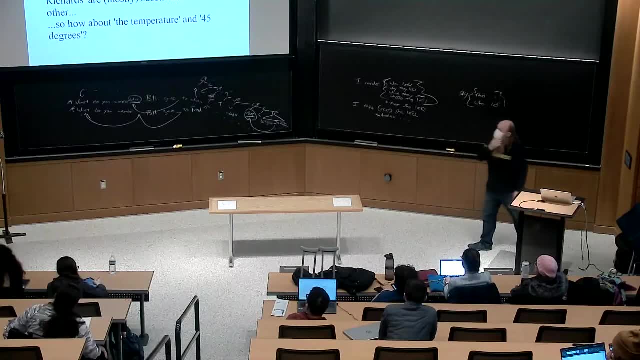 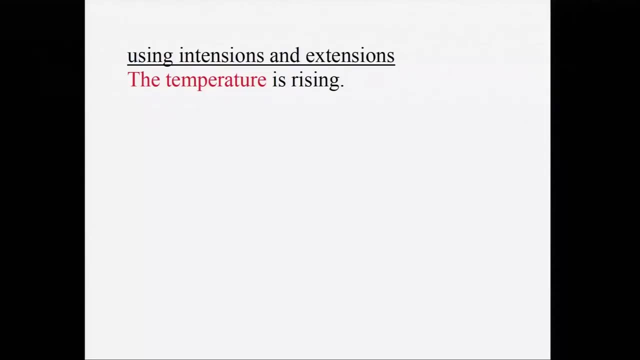 we have to be careful with phrases like the temperature and 45 degrees, etc. degrees. So the temperature has an intention and an extension, and its extension might be 45 degrees, but its intention isn't necessarily. Which means that, for example, even if it's true, the temperature is rising and it doesn't. 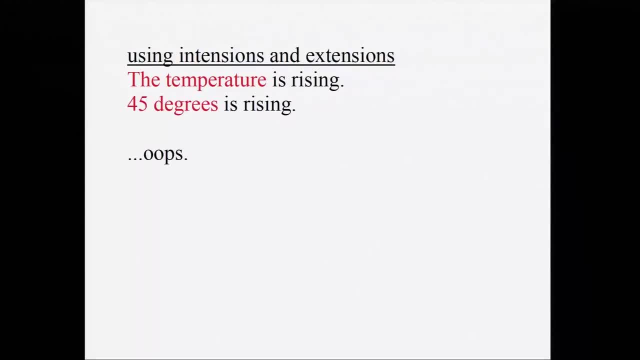 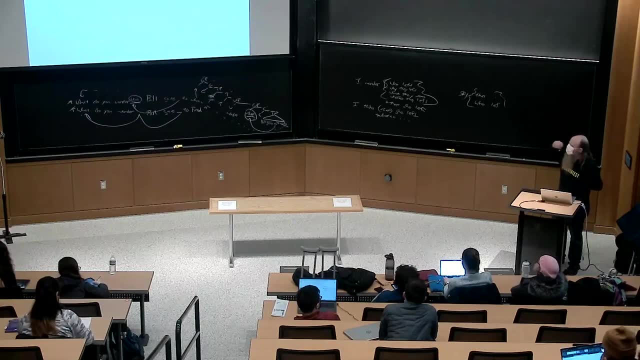 follow that 45 degrees is rising. So even if it's true that the temperature is 45 degrees and that the temperature is rising, So here's a place where it seems as though you can't substitute in one phrase for another, That's because 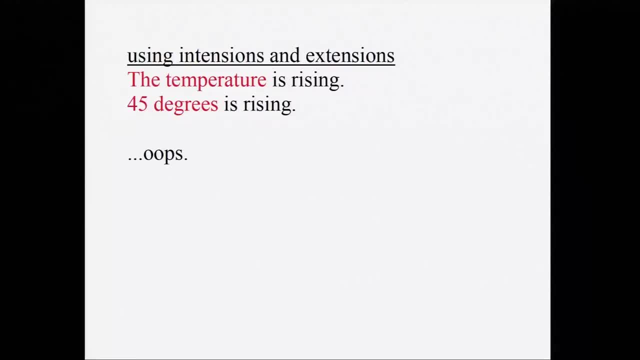 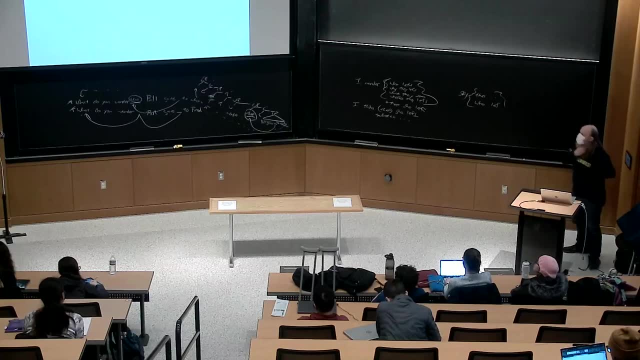 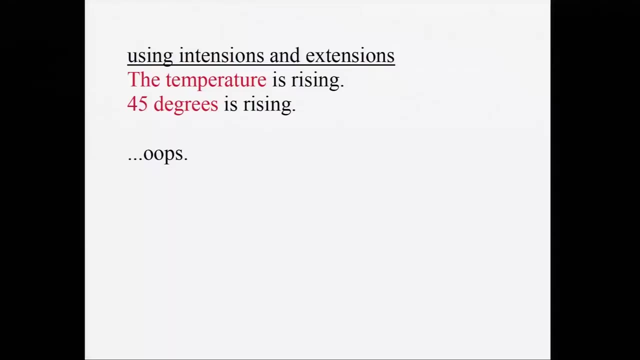 rising is interacting specifically with the intention. It's telling you something about what you will see if you look at the thermometer. It's not telling you something about the extension of the phrase the temperature. So there are places where you can confuse yourself with intentions and extensions. 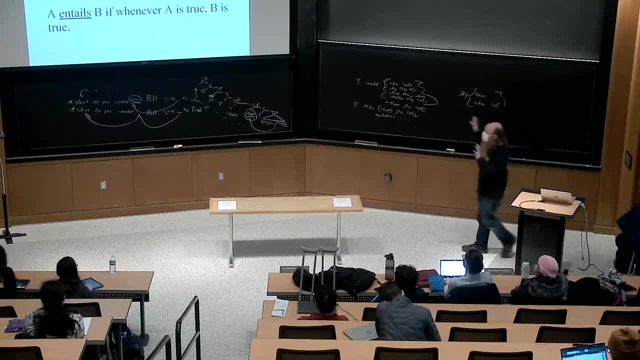 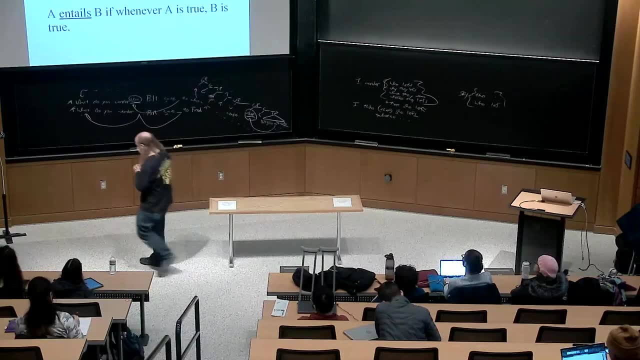 Okay, let's extend the focus a little bit and talk about sentencesSo that's, you know, the beginnings of some things we'll have to watch out for when we look at the meanings of phrases, When we start talking seriously about the meanings of. 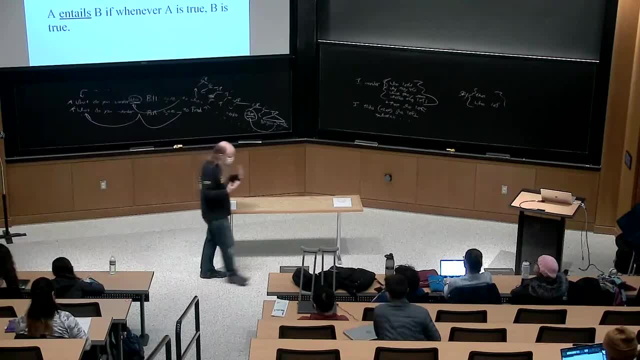 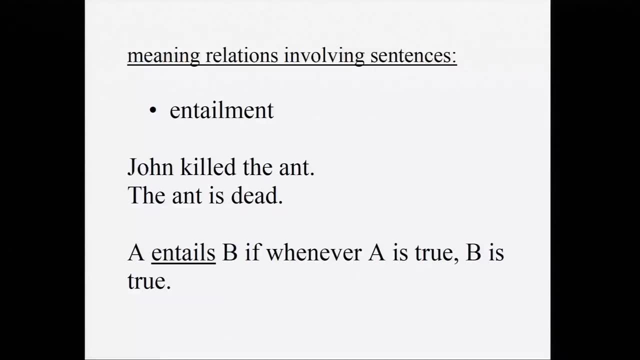 sentences. there are some relations between sentences that it's going to be useful to keep track of, So one of them is entailment. So we say that a sentence A entails a sentence B. if whenever A is true, B must be true. So if John killed, 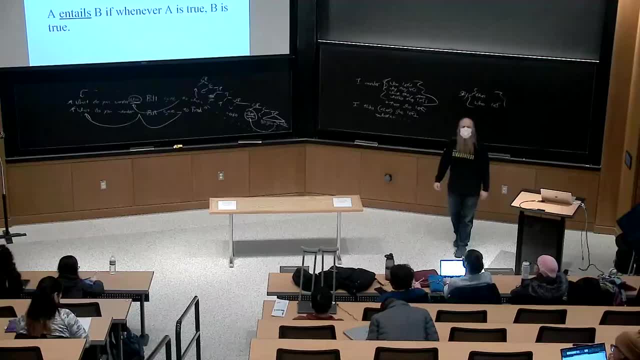 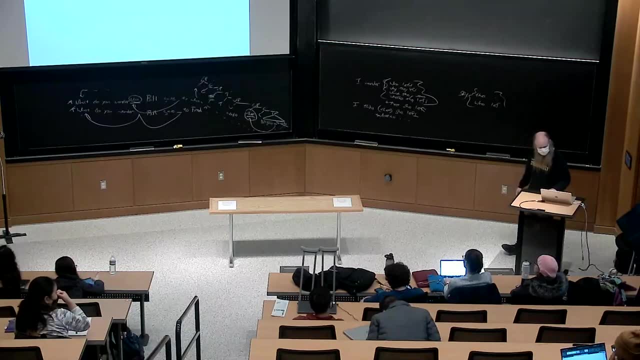 the ant, it has to be true that the ant is dead. That's what kill means Yes. So for this example, we have the intention and the extension and the intention is not fixed right. Yeah, It's just 45 degrees now. 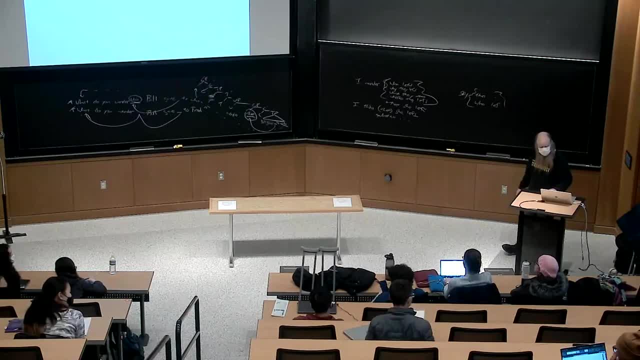 50 degrees next day. If we said the winner of the previous election, would that be always substitutable for the right? So, oh, the winner. so let's see now The phrase. let's go back to Joe Biden. 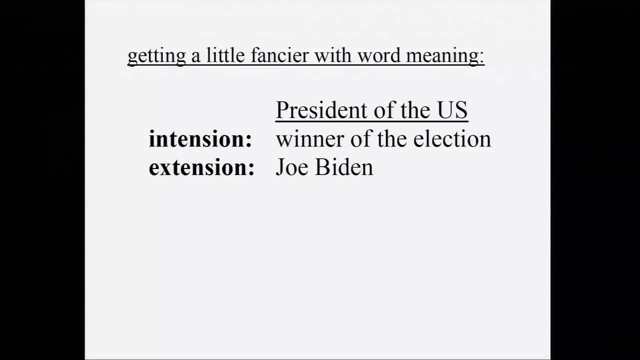 Here he is. It's not always going to be true that the winner of the previous election is substitutable for Joe Biden, because I can say things like: in 1945, the President of the United States declared war on Japan, right And that. 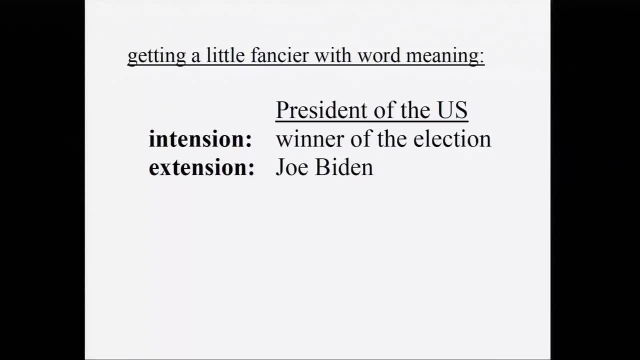 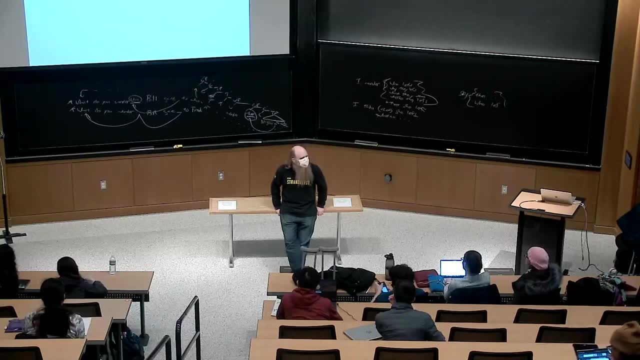 phrase that's probably at the wrong year. That phrase, even if that sentence is true, I don't get to substitute that in for Joe Biden. That's a case where it refers to a different person, the person who won the election previous to that. 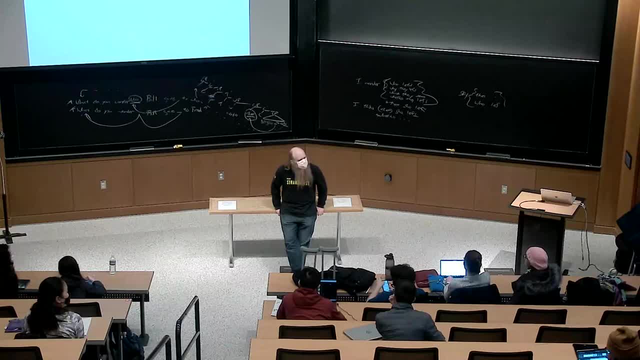 Am I getting at your? I feel like we could get here now. Probably, Probably, This is day one of semantics, but yes, yeah, you're right. This is mainly meant to make you wary about expressions like the meaning of a phrase. 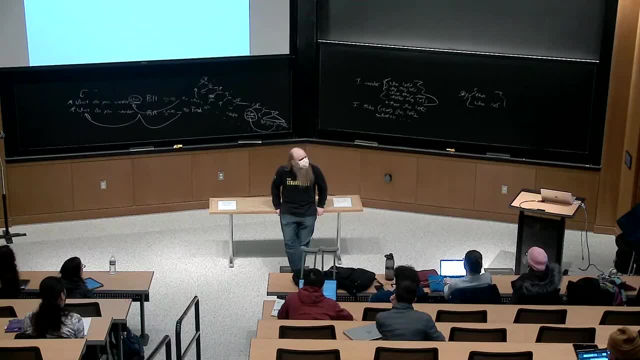 The meaning of a phrase has more than one dimension. You have to be careful about what kinds of predicates it's interacting with. I mean similarly, if I say something like the President of the United States has always been male, That's true. It's also true of 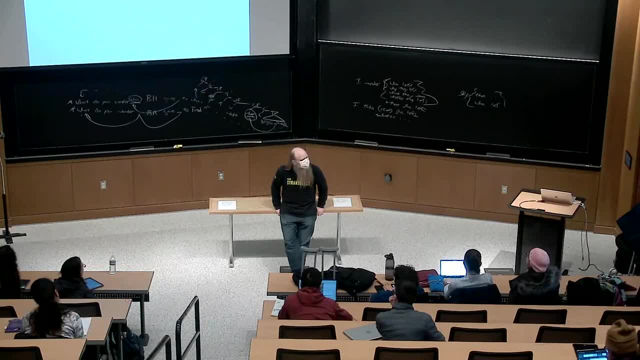 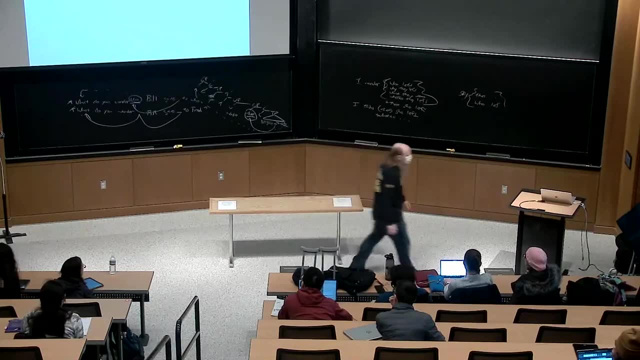 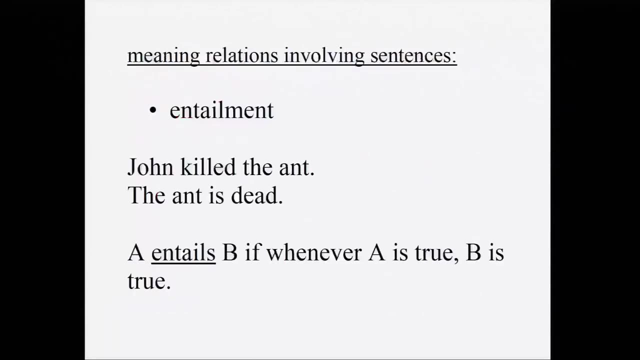 Joe Biden, as far as I know. but those aren't the same claim. All right, yeah, Yep, Okay, Okay, Okay, Okay. Rising ants, Dead ants, Okay, Yes, so entailment. One sentence entails another sentence. 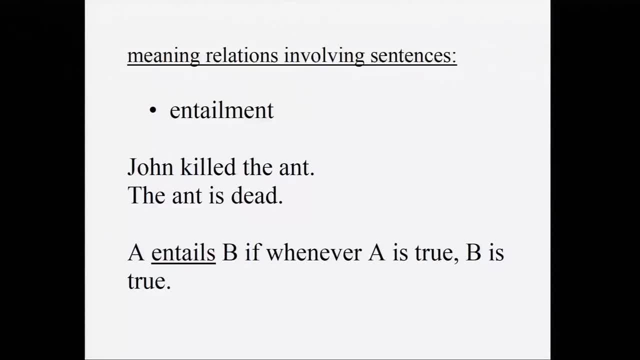 if, whenever the first sentence is true, the second sentence has to be true. That's what entailment means. Similarly, to say Norvin is Don's nephew is to say that Don is Norvin's uncle. The first of those sentences entails the second. 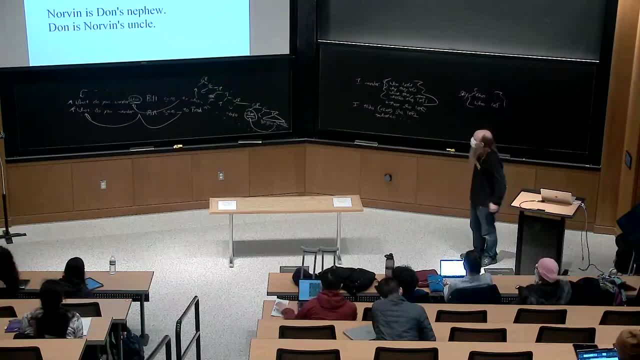 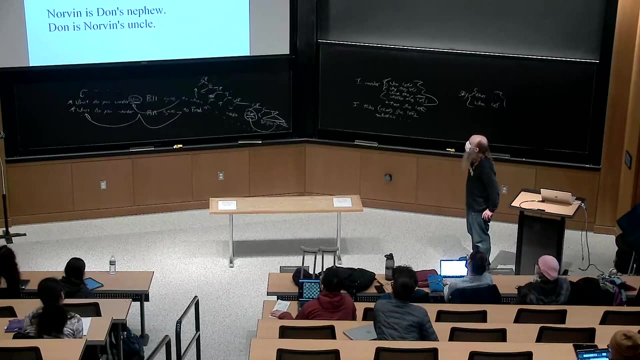 No, it doesn't. Actually, this is a lie. Neither of these sentences entails the other, unless you know that Norvin and Don are both male. If you know that Norvin and Don are both male, then they entail each other, Otherwise. 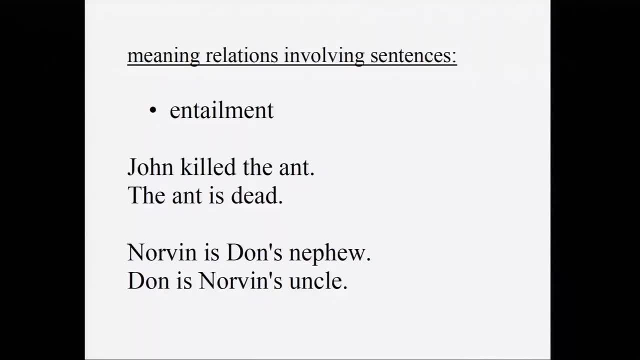 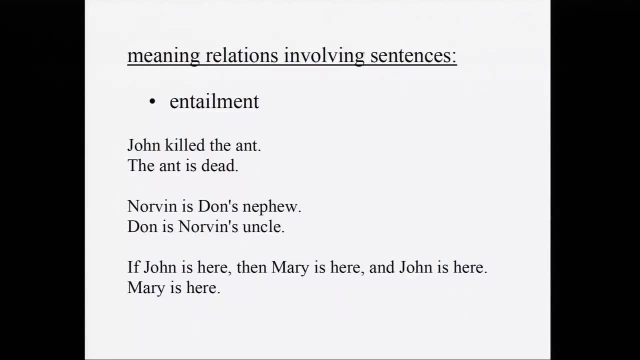 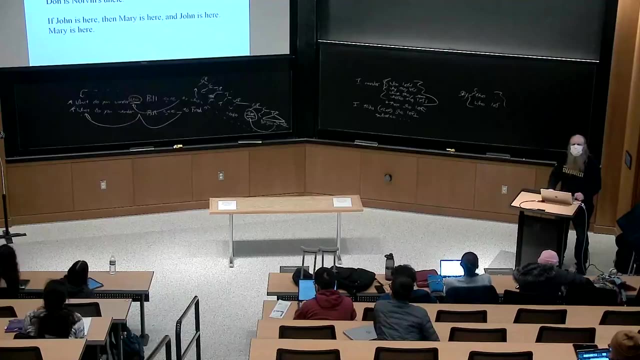 not, I guess. Yeah, Hmm, I should fix that, Or here I think this one does work. If John is here, then Mary is here and John is here. That first sentence, that long sentence, entails that Mary is here. 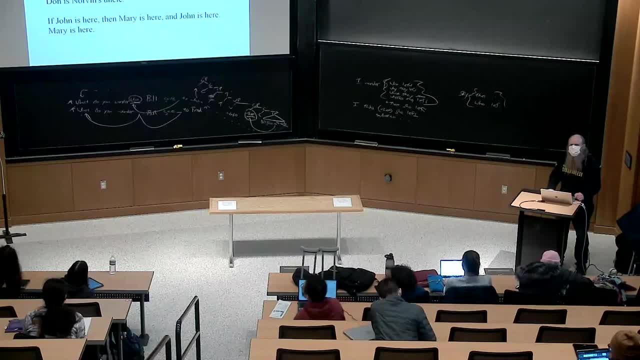 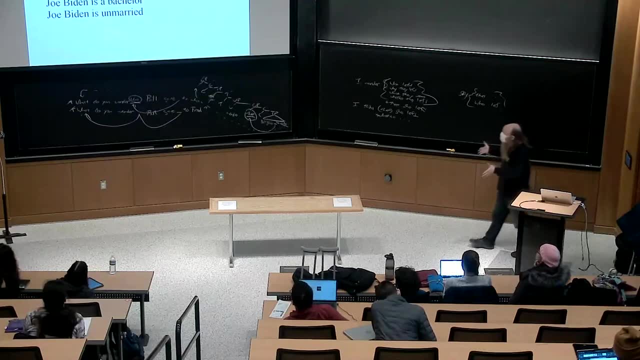 So if that first sentence is true, the second sentence is true. Okay, so these are entailment relations. Entailment relations are not about whether the sentences actually are true. So to say that sentence A entails sentence B is just to say, if you imagine, 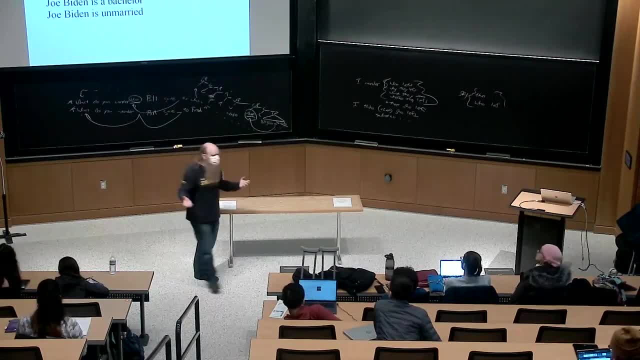 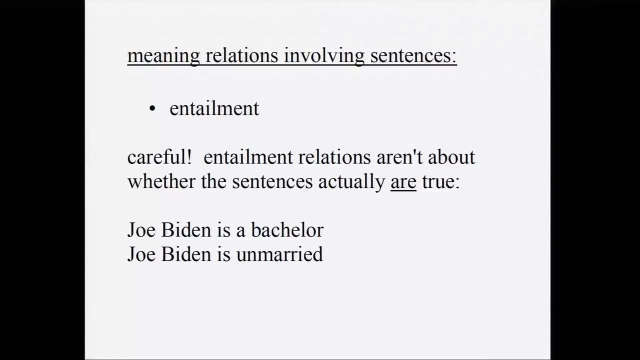 that A is true, then B is also true. So Joe Biden is a bachelor entails that Joe Biden is unmarried? Yeah, They're both false, but if the first sentence were true, the second sentence would be true. Does the second sentence entail? 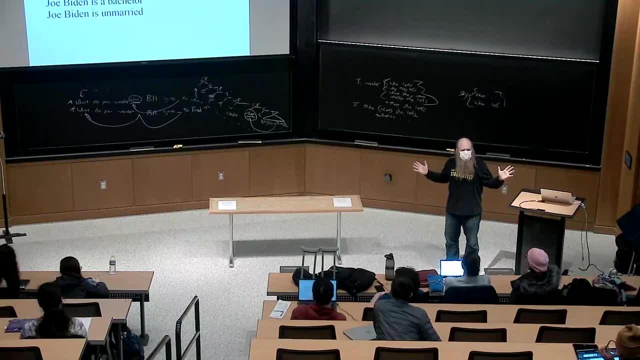 the first, What is a bachelor? An unmarried man? If Joe Biden is a man and he's unmarried, He may be a bachelor, but Joe Biden could be a woman for all we know. Right, yeah, that's an example. 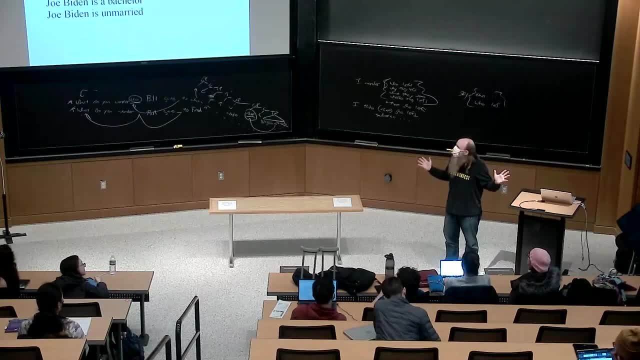 And actually I think I misspoke when I said that a bachelor was an unmarried man. If his wife had died he would be unmarried, I guess, But not a bachelor. I think a bachelor is someone who has never married- Also false. 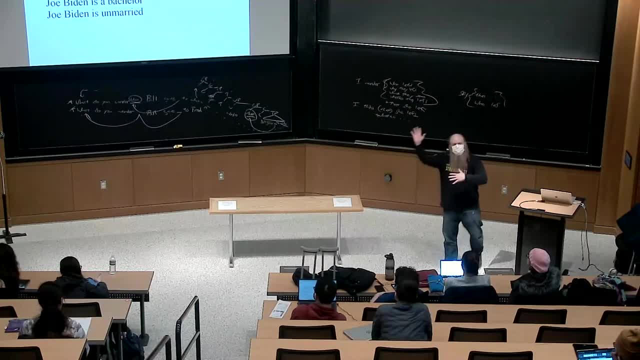 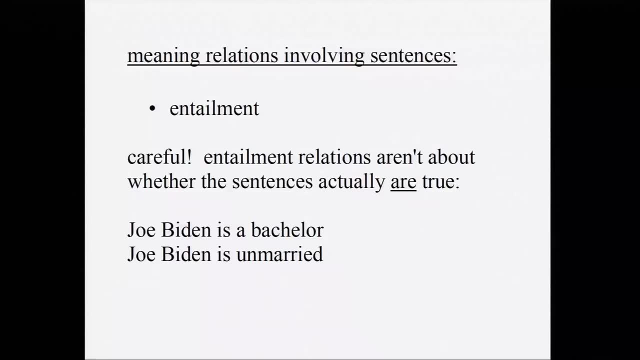 He's actually married. Okay. so entailment relations are not necessarily symmetrical. It's possible for A to entail B and for B to not entail A. And entailment relations are about what life would be like if the first sentence were true. It's not about whether it is. 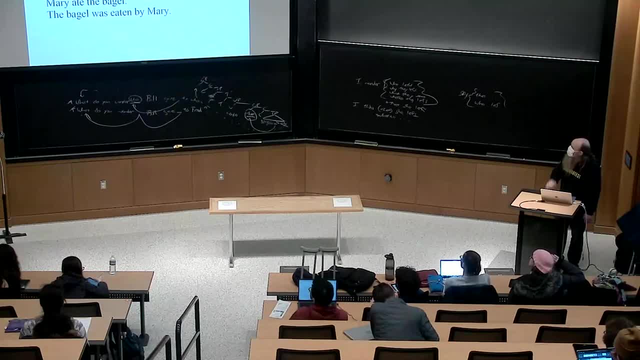 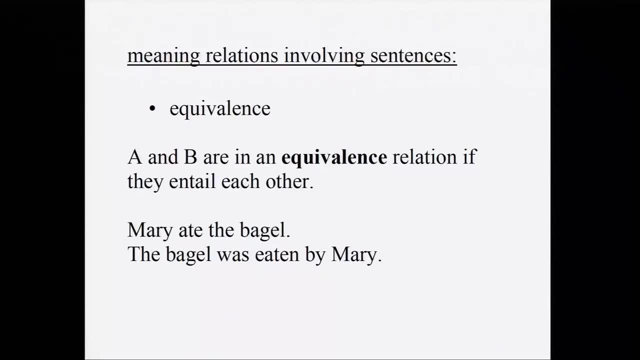 true, And we say that A and B are in an equivalence relation if they entail each other, Also say that they're synonymous. So, Mary, ate the bagel, and the bagel was eaten by Mary. The first sentence entails the second and the second entails the first. 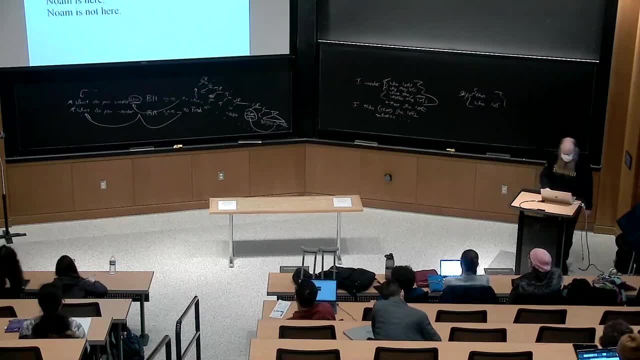 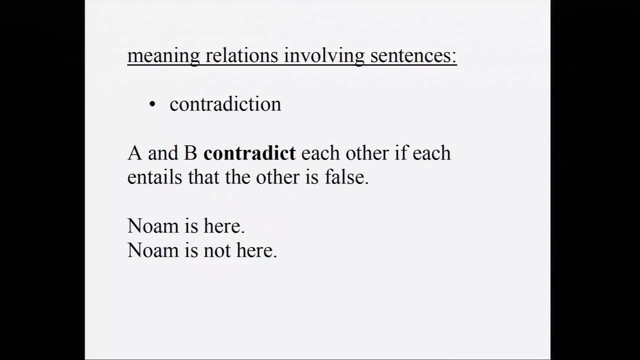 These are equivalent sentences And we say that they contradict each other if each entails that the other is false. So as long as gnome always refers to the same person, if gnome is here, that entails that it is not true that gnome is not here. 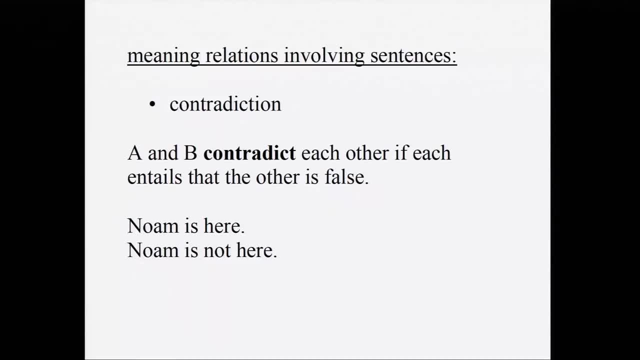 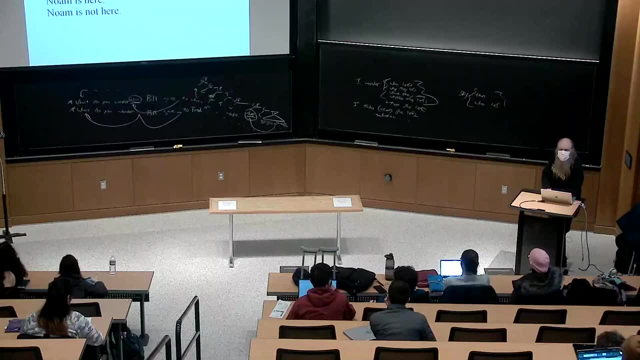 And if gnome is not here, that entails that it is not true that gnome is here. I'm waiting for somebody to work hard on the meaning of here. Yeah, which I guess we could Suppose. he's halfway into the room, or something. 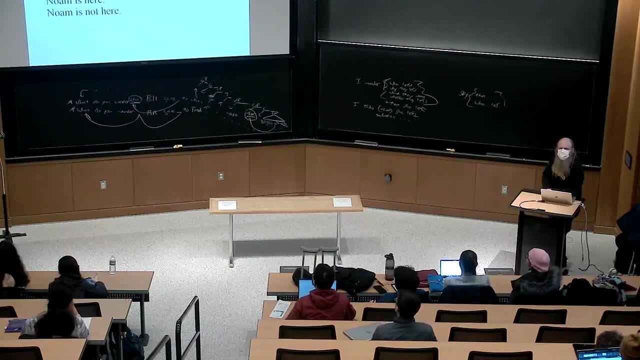 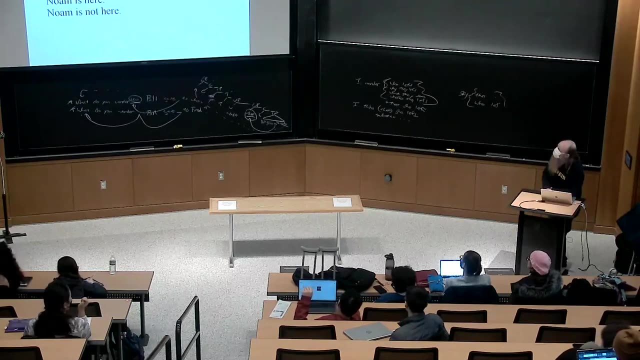 Forget about that stuff for a second. Let's pretend that people are either here or they're not here. Okay, so we say that A and B contradict each other if they each entail the falsehood of the other. Yeah, Can I assume that it's possible for A? 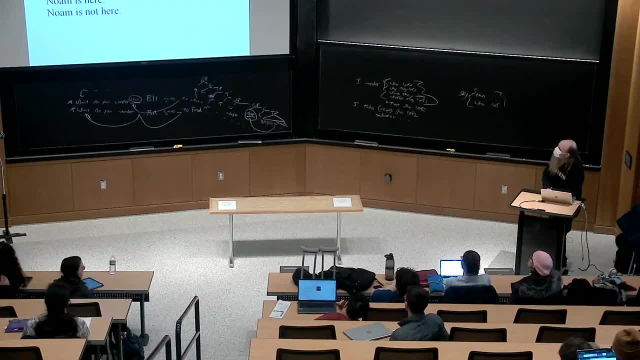 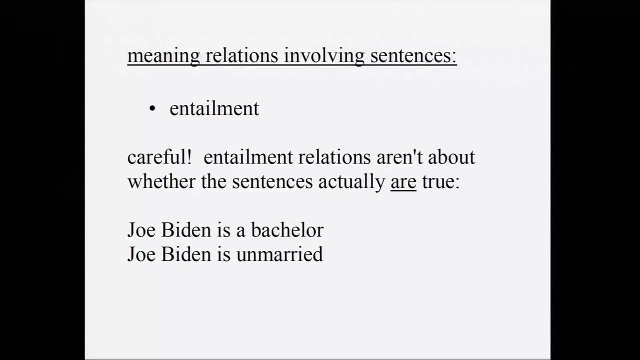 Is it possible for A to contradict B, but B not. So for A to entail that B is false, but for B to not entail that A is false. Yeah, So, If you, If you. I got back to this slide because I feel as though. 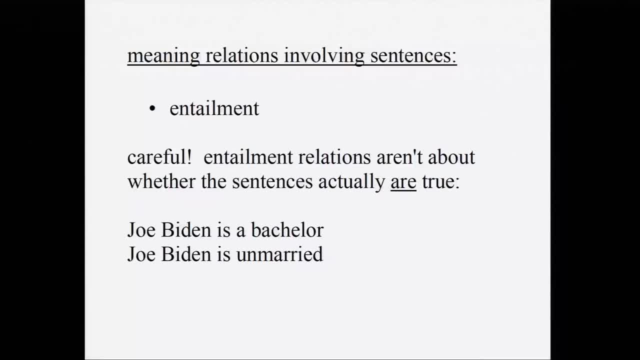 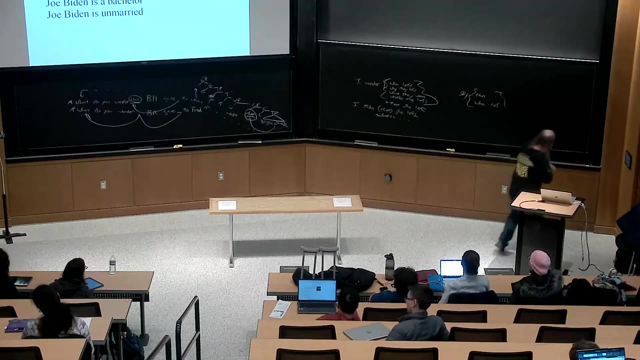 if we arrange things correctly, Yeah, yeah. So if Joe Biden is a bachelor, Nope, What's a better example? So So we're looking for a case of a subset relation where all Is it rectangle and square. Is it rectangle and square? Yeah, that's better, isn't it? 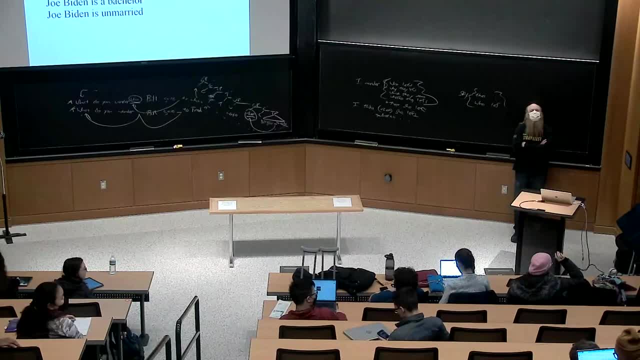 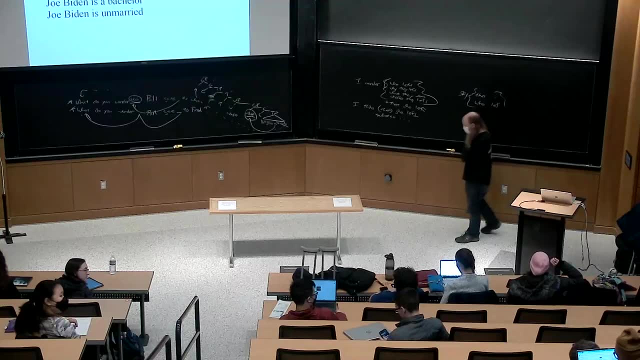 Yeah, go ahead. Give us the rectangle and square example. If you say that something is not a rectangle, that doesn't necessarily mean that it isn't a square. If you say that it isn't a square, that means it's definitely not a rectangle. Yeah, okay. 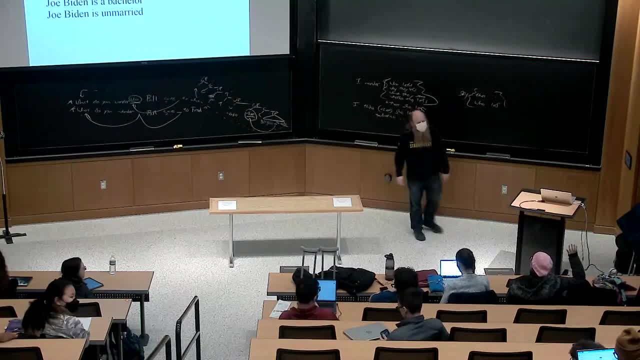 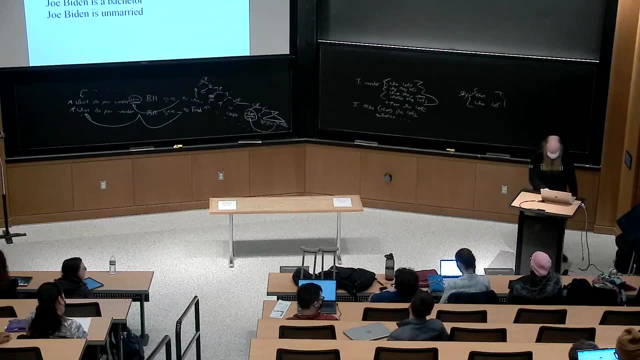 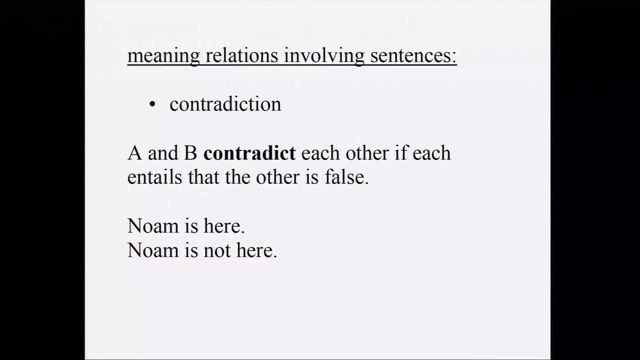 Other way around. Oh, okay, Other way around, Good, Yes, I think that the logic rules are like: if you have something like, then Q, then it follows that not Q implies not P, but you have no idea whether Q implies P or not. 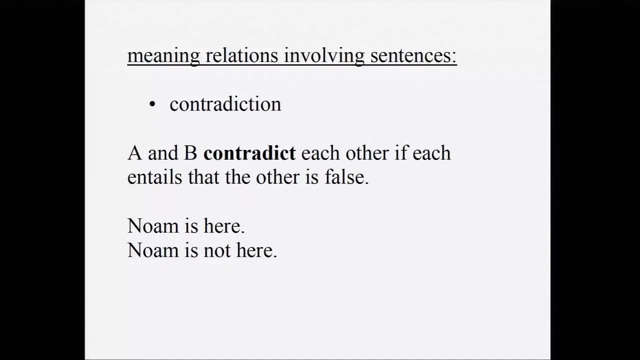 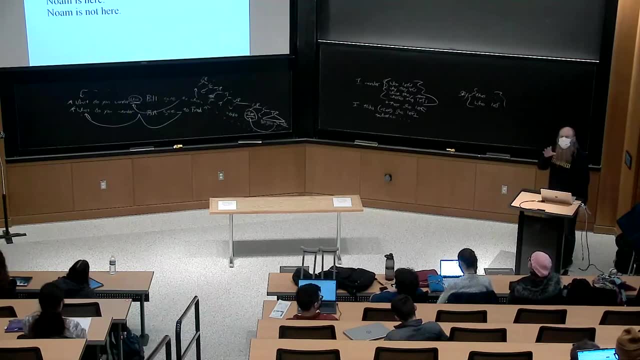 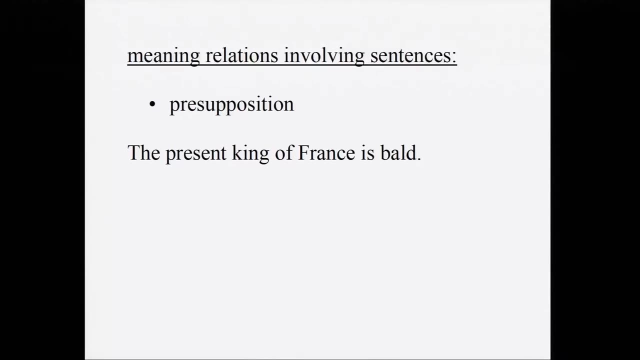 Yes, yes, yes, yes, That's true. So that is what people say about if P is Q. Yeah, you're right. Yep, Yes, Okay, good, I'm gonna move away from entailment and start talking about presupposition. 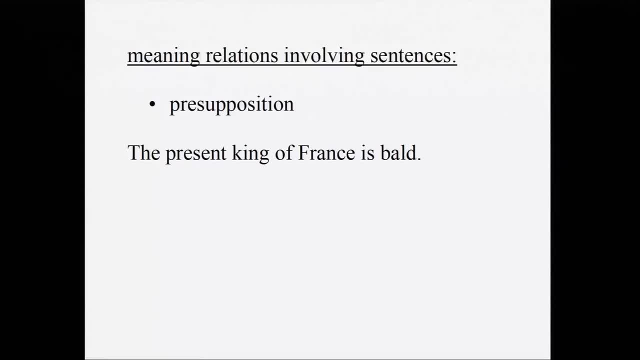 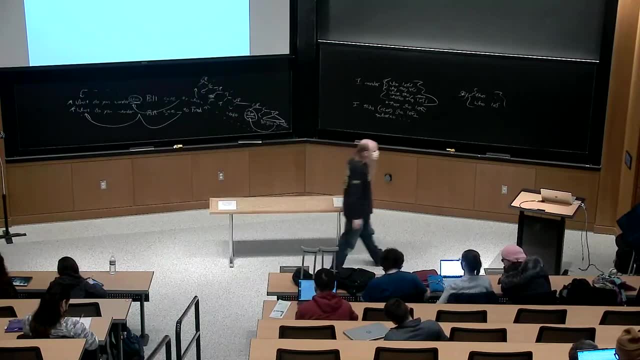 Presupposition is another kind of relation between sentences. Again, it doesn't matter whether the sentences are true or not. You're being invited to imagine what life would be like if they were true. So a sentence like the present king of France is bald. 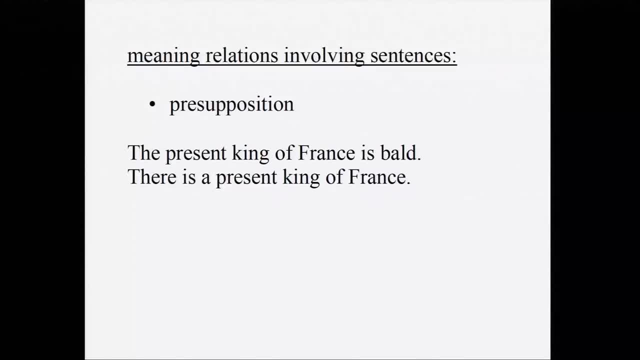 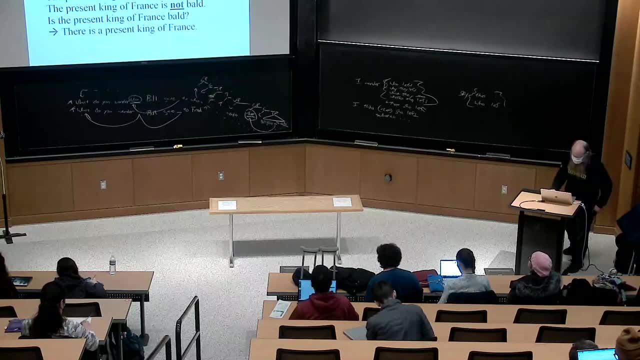 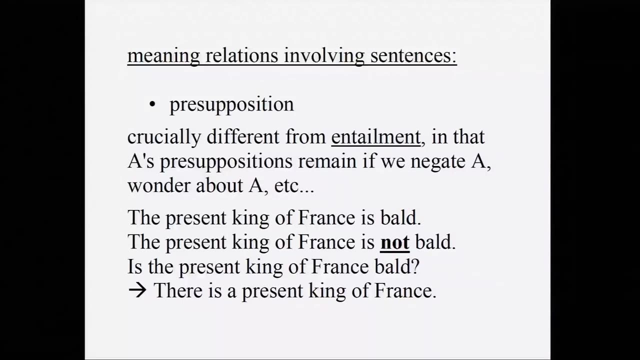 presupposes that there is a present king of France. This is different from entailment in ways that I think I illustrate on the next slides. Yes, Crucially different from entailment. If I say the present king of France is bald, or if I say the present king of France. 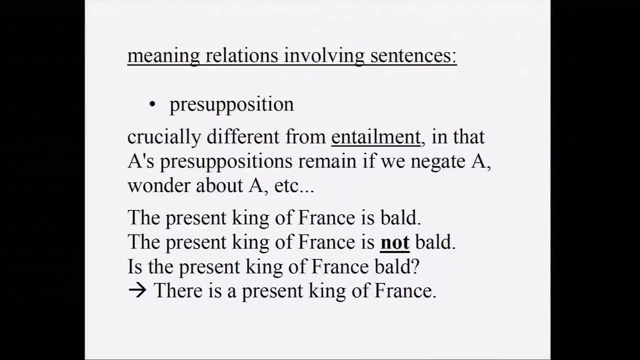 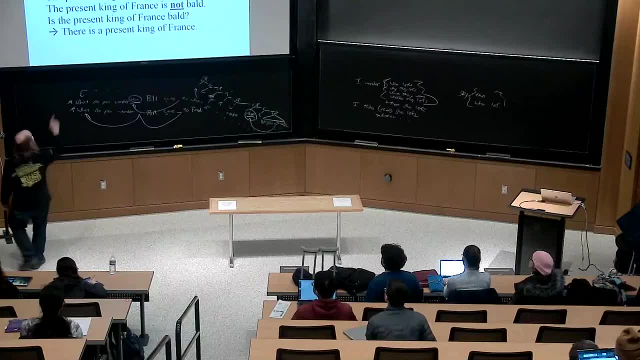 is not bald. or if I say, if I ask you, is the president of France bald? All of those have this relation of presupposition to there is a president king of France, that is, we can stick to the first two. If I say the president king of France is bald, 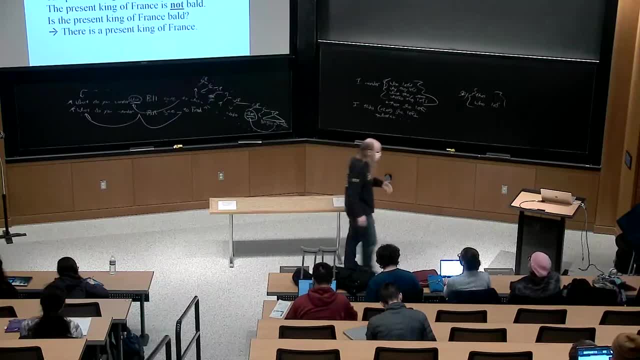 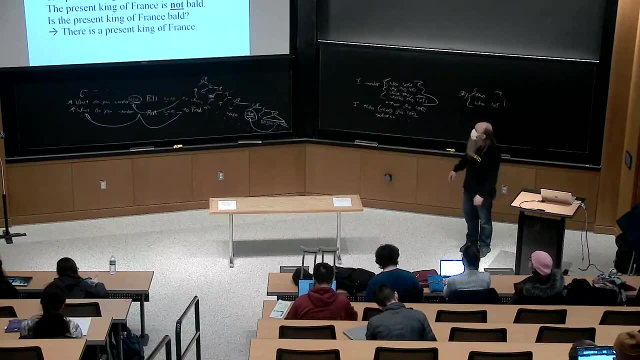 or if I say the president king of France is not bald. for either of those to be true, there has to be a president king of France. That's different from entailment. So for entailment, when we did things like John killed an ant. 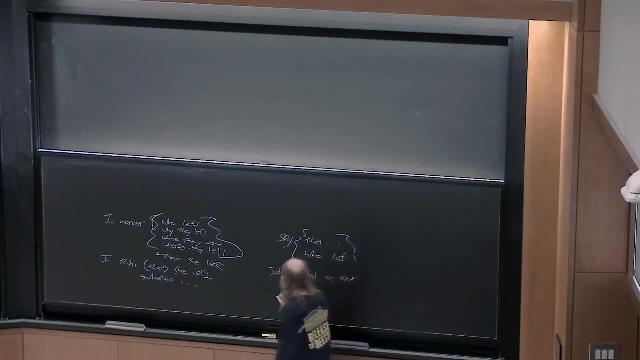 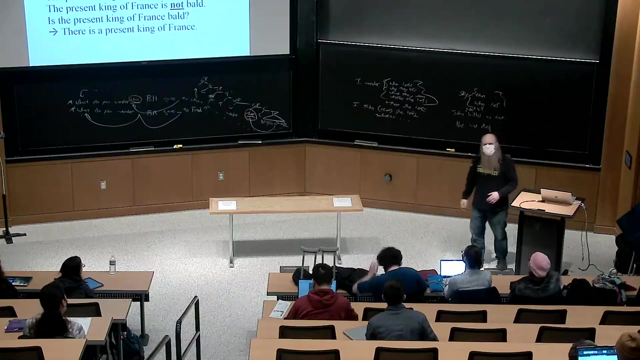 and the ant died. that's an entailment relation. If I say John didn't kill an ant, well, if John didn't kill an ant, then the ant didn't die, at least not necessarily The ant might be alive. So to say that John killed an ant entails that the ant died. And if I negate 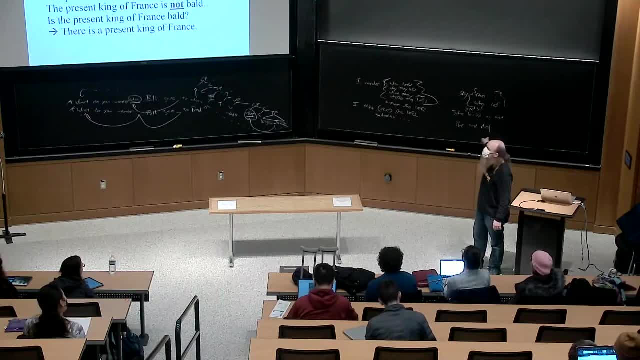 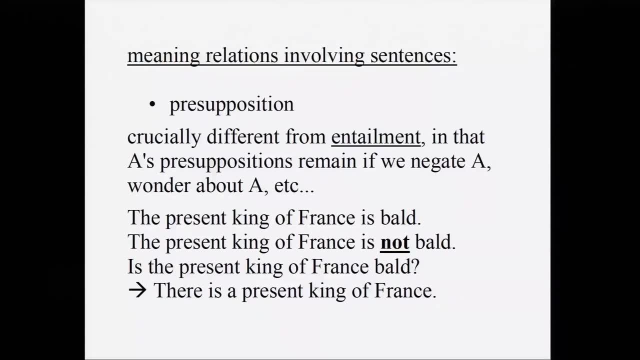 the first sentence, I no longer entail what I used to entail. But if you negate a sentence, that presupposes something. so if you add- not if you go from the present King of France is bald to the present King of France is not bald, you still have the presuppositions that you used to. 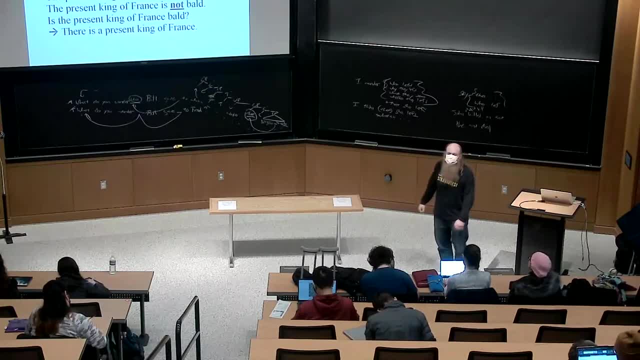 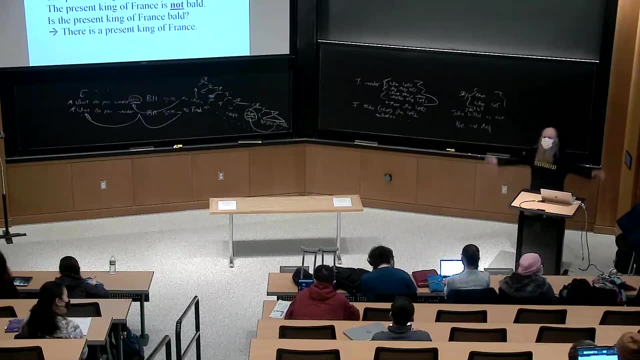 have You still presuppose, so it has to be true- that there is a present King of France. Yes, Yes, Which is true, by the way, if anybody's learning about the world from this class. Oh, so if there is no present King of France, ah, if there is no present King of France, 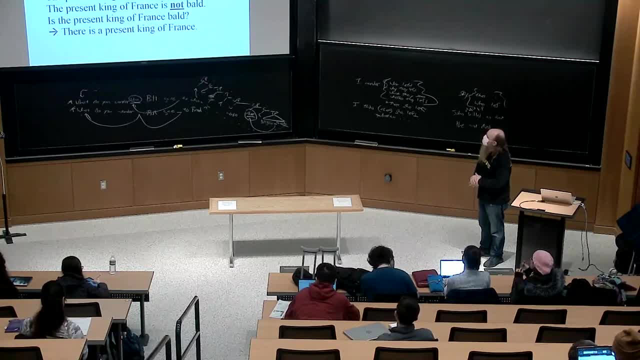 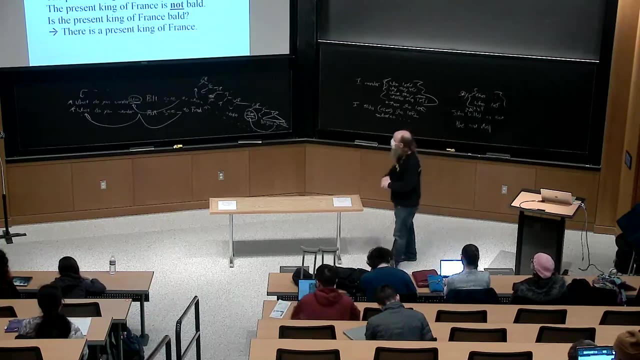 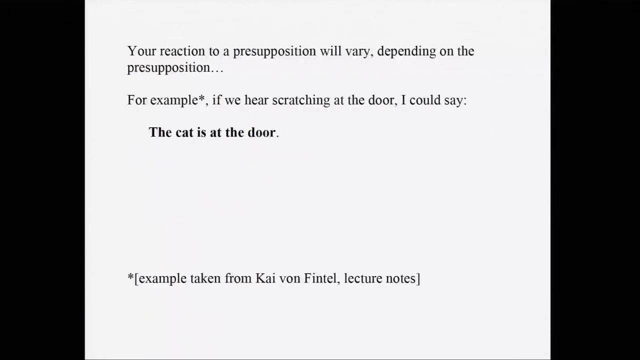 yeah, good point. Their truth value becomes difficult. This is sometimes called presupposition failure. So if I say a sentence that presupposes something false, we're actually going to talk about this, I think, on the next slide. Uh, your cognitive state becomes difficult, Um so um. this is a classic uh of it's used in: 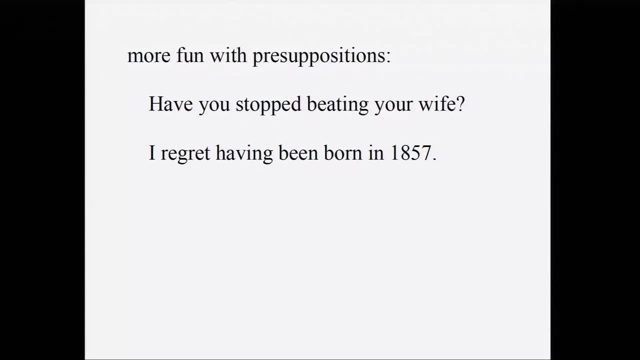 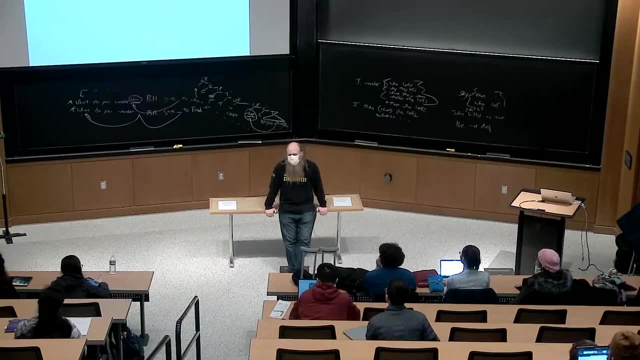 politics and also in comedy. uh, unfortunate example from the Marx Brothers. uh, Marx Brothers ask: at some point, have you stopped beating your wife? Um, uh, the point of the question is that there's no good answer. um, if you say yes or no, you're accepting the presupposition. 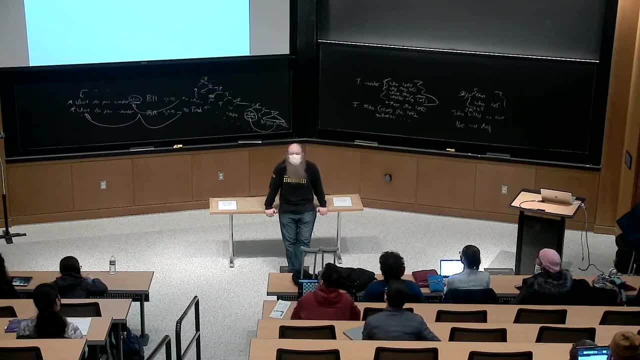 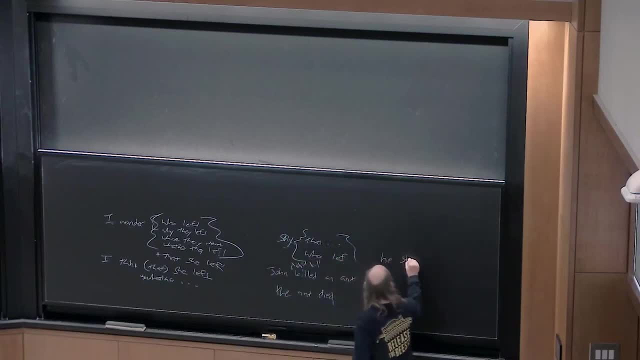 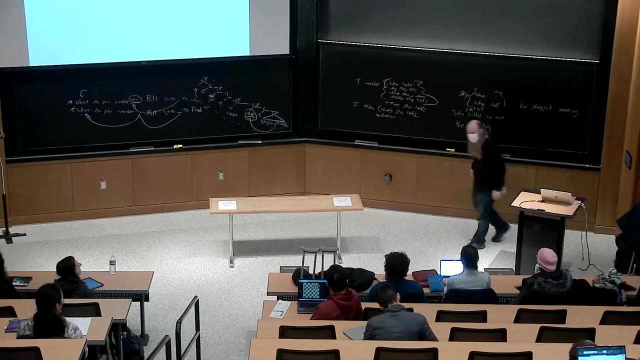 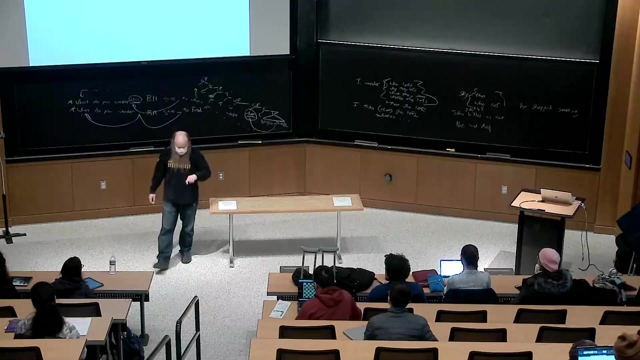 that you used to have To beat your wife. That's what this question does, right? Um? the corresponding statement has the same presupposition. So, uh, he stopped smoking. presupposes that he used to smoke, right? Um? and uh, that means that, um, if I presuppose something which is false, so if you, 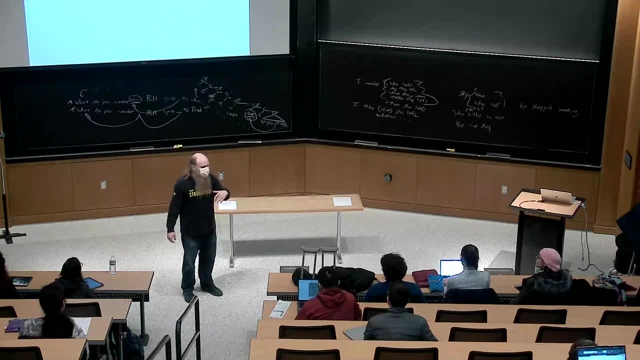 ask me: have you stopped smoking? Um, you're presupposing that I used to smoke, And if that's false, it's not a no. It's not enough for me to either say yes or no. I inherit your presupposition. Um, I have. 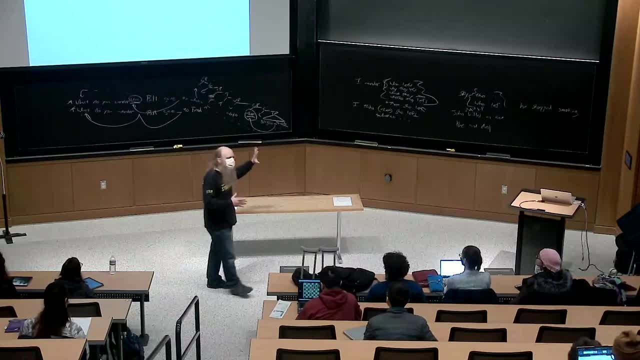 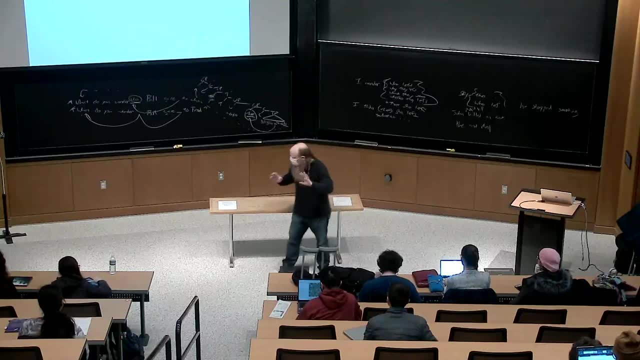 to say something. I have to say something like: wait, I never smoked in the first place, right, Or you know, your presupposition is false, Something like that. There's a? um, a literature in the literature on Zen, Buddhism, which I'm not an expert on, um, there's a. 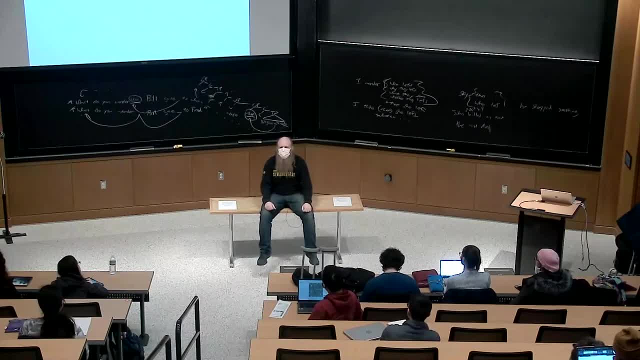 kind of exchange between teachers and students. that happens a lot, where a teacher will ask a student the question: uh, the teacher will. the student will ask something like you know, uh, does the dog have the Buddha nature? Uh, or something like that, And the teacher, by way of 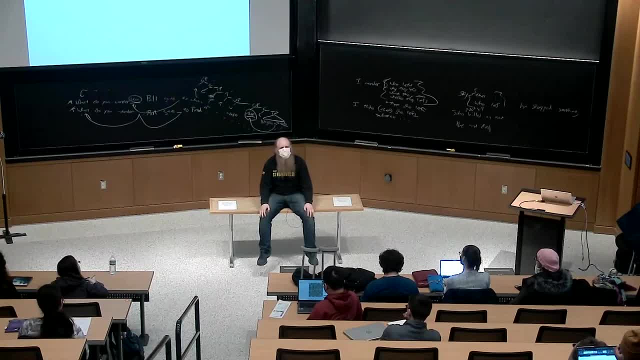 answer will haul off and slap the student, or pour cold water on the student or shout moo And the student is enlightened. This is a kind of story you see a lot in the Zen Buddhism literature. Uh, I don't know a whole lot about Zen Buddhism, but I've always wondered whether 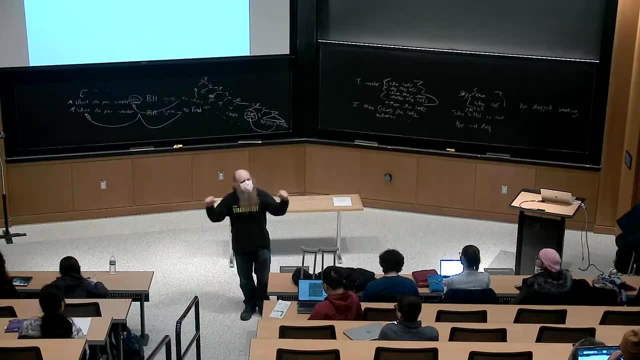 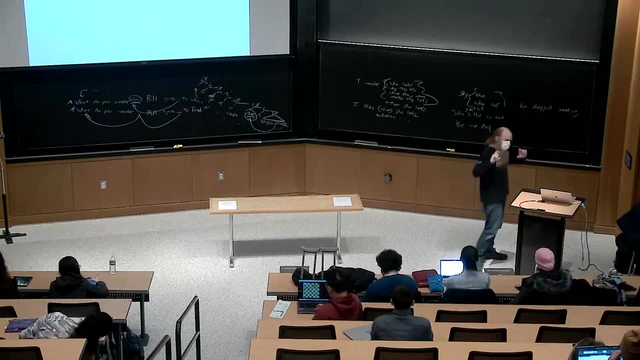 moo means you are making a false presupposition, Because it's an interesting fact about languages that we we have words that are you know, they're, they're, they're, they're, they're, they're- words like yes or no, that that say things like the statement that underlies your question is: 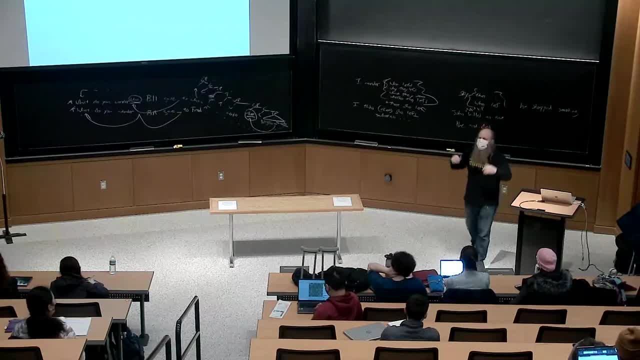 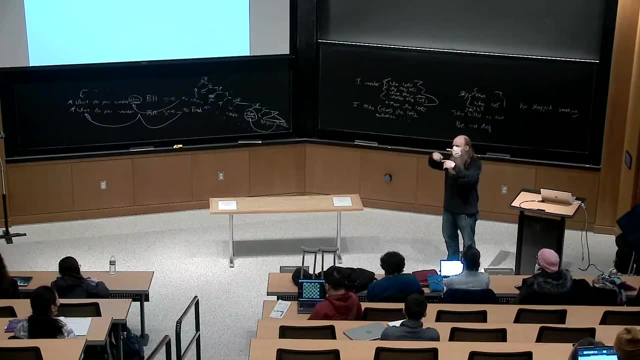 true or false. If I ask you, is it raining? You're asking me to evaluate the truth or falsehood of it is raining And I'm supposed to say either yes, it's true that it is raining, or no, it's false. 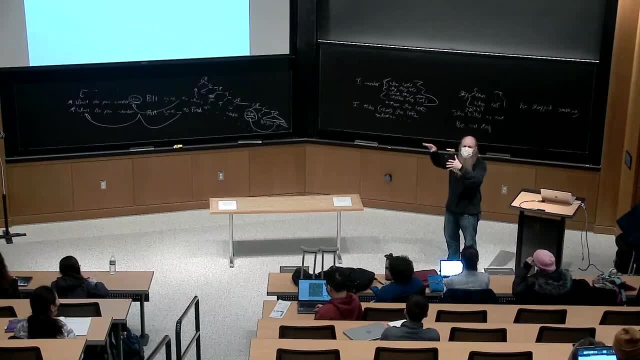 that it's raining. Yeah, You ask me: have you stopped smoking? Uh, the statement that you're asking me to evaluate is: you have stopped smoking. And I have yes and no as my sort of standard options, but I don't have an option to say yes or no, And I don't have an option to say no. 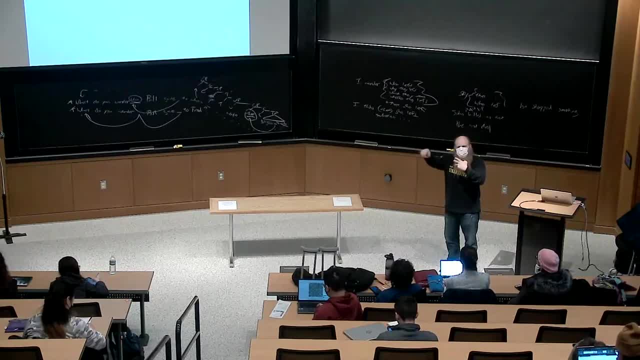 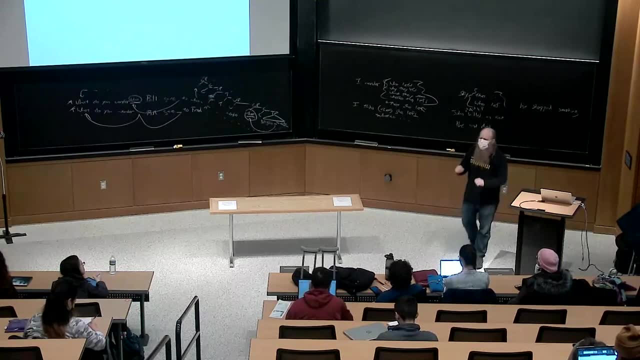 I have an option that says there is a false presupposition, Yeah, And, and most languages don't Like. it's not common for languages to have something to say that means you have made a false presupposition, Uh and so, yeah, it's interesting that languages work this. 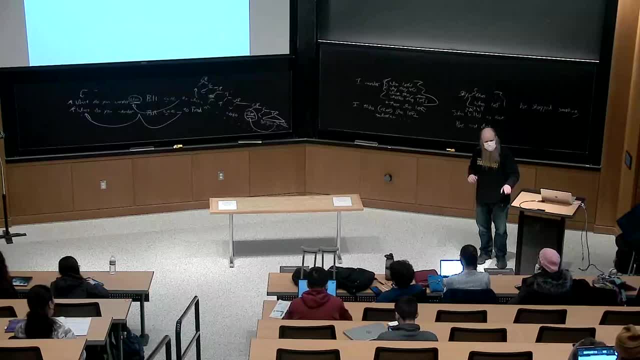 way. That's interesting because I think in in like math, like in in like formal logic, if the um it's like, you know, if this, then that, then if this is just false, then 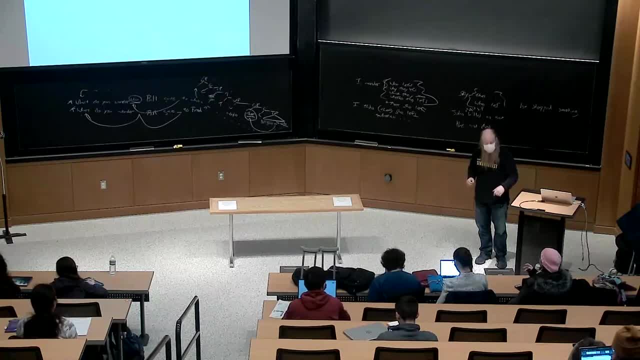 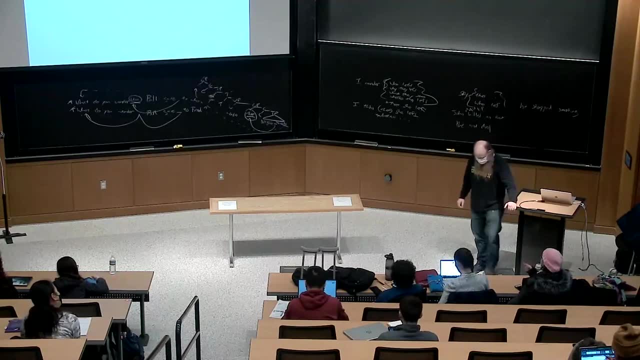 it's the whole thing is true, just by default. Um, and the thing I'm wondering is, like: does this mean that when you ask a question, you are actually asking like: have you stopped beating your wife? You're asking like, like: are all the presuppositions in this true? 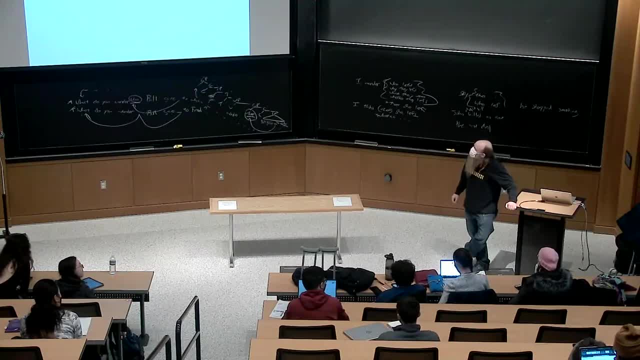 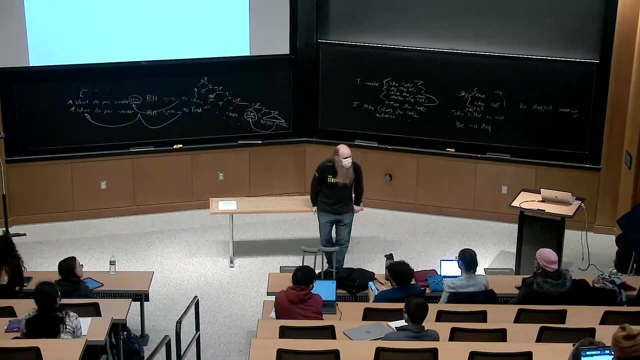 And is this also true? So that's just it, though I'm not asking you whether the presuppositions are true. That's why, uh, if I ask you this question, uh, change it to have you stopped smoking. Uh, uh, if I ask you, have you stopped smoking? Um, you can't say no and have that mean. 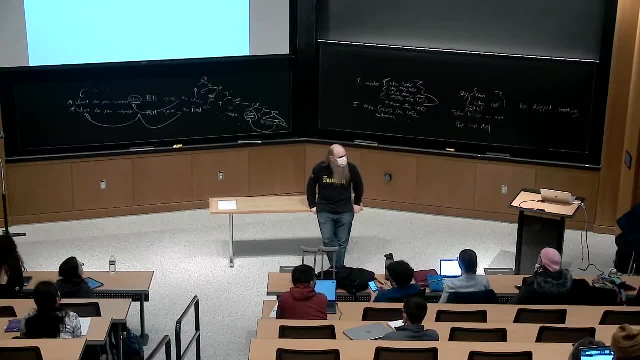 uh, and have me interpret that as meaning uh, you never smoked in the first place, right? Um, you're absolutely right that, if you were, uh, this is the kind of thing that, like robots and aliens, get wrong standardly in science fiction stories, right? 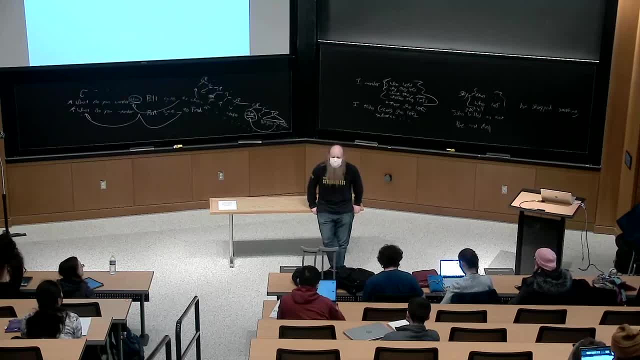 That, uh, you know false presuppositions lead to sort of ungrammaticality or something like that, something weird going on. Did I get it? the answer to your question? So presupposition failure, this case where I say something that has a false presupposition. 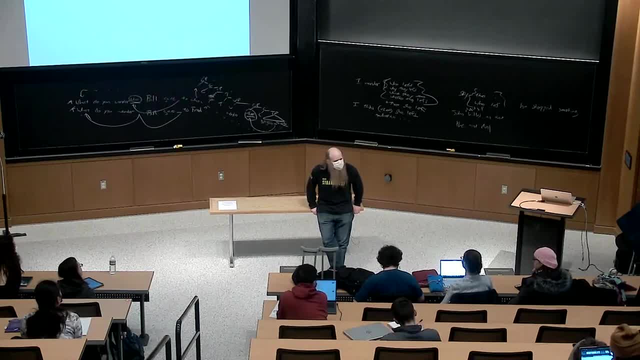 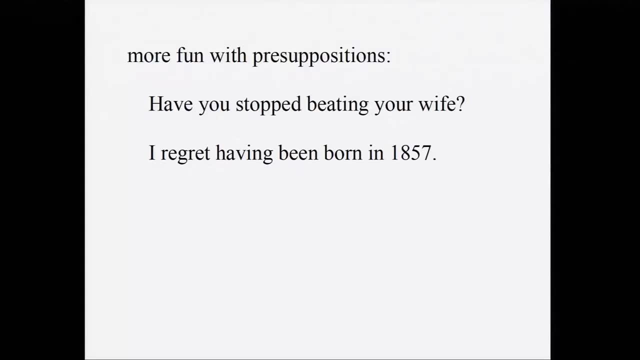 uh, it doesn't make the sentence false. It makes the sentence weird. Um, uh, yeah, that's the expression that we, or the feeling that we have. Um, I skipped some slides to get to this one, so let me go back a bit. 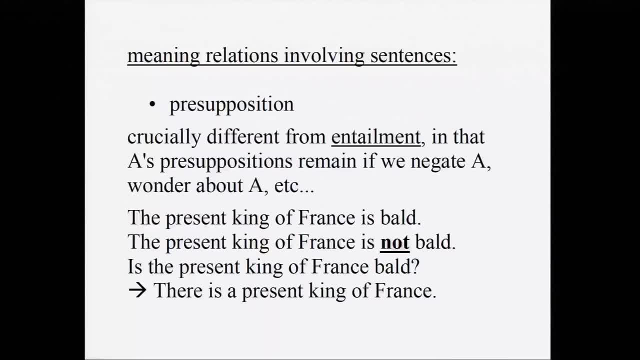 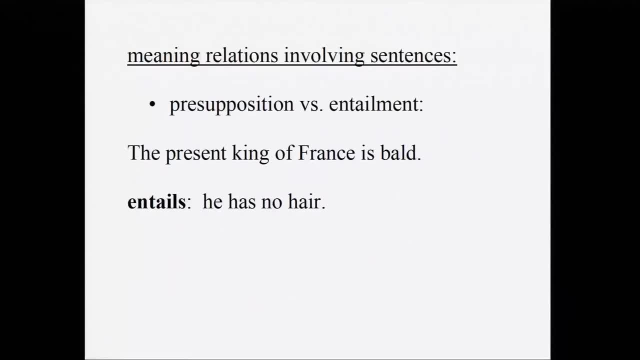 Um, okay, yeah, So, uh, present king of France is bald. uh, presupposes that there is a present king of France, It entails that the present king of France has no hair, right? Uh, because that's what it means. Um, and so you know, if I say the present king of France is not bald, 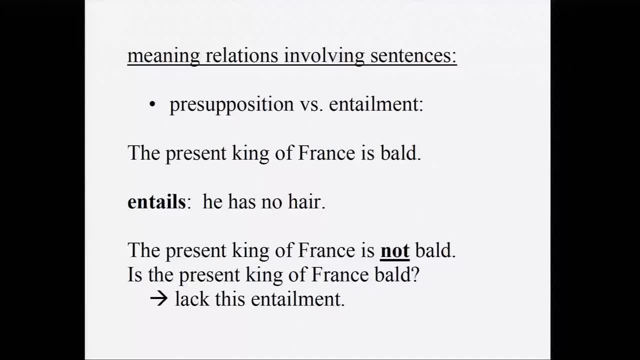 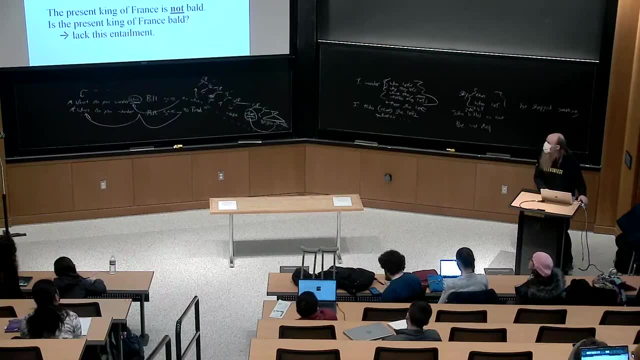 um, uh, that no longer entails that he has no hair. So that's the difference between entailments and presuppositions. Entailments, uh, don't survive. negation: If you add not, then you lose the entailments that you used to have, but you still have the presuppositions. 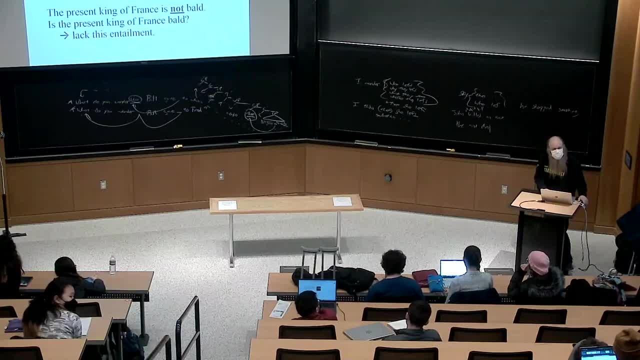 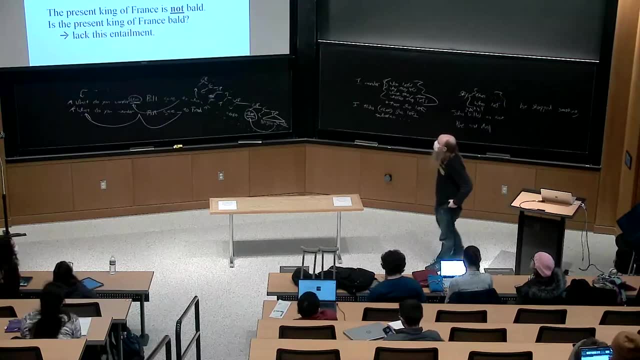 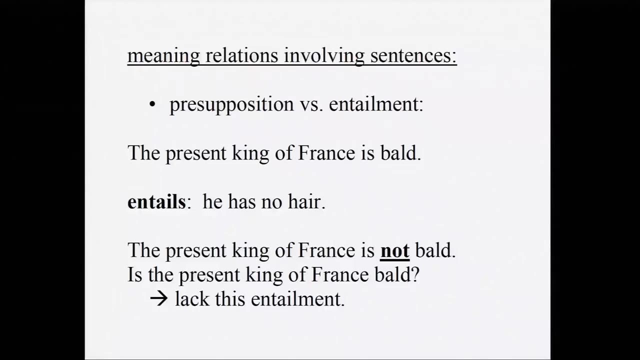 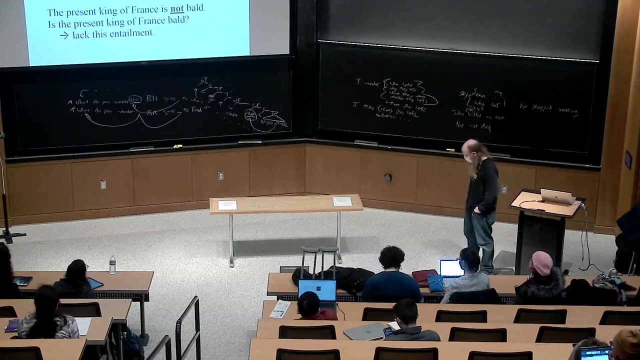 that you used to have. Yeah, Could you just then say that entails the opposite. Say it again. Could you then just say that entails the opposite, Like it entails that he has hair. Oh, in this particular case, Uh, yes, I think we're going to find examples where A entails B, but not. A does not entail. 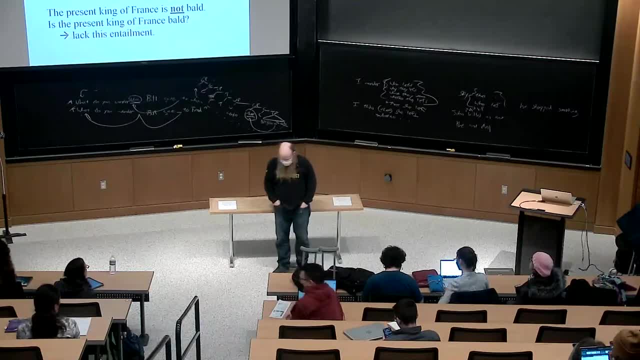 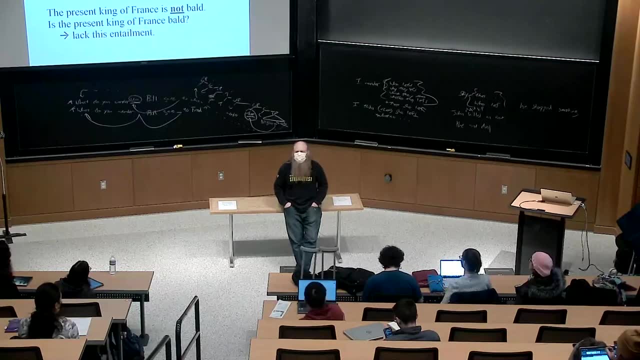 not B. So yeah, if something is a rectangle, then it. no, if something is a square, then it is a rectangle. Did I get that right? Um, but if something is not a square, that doesn't mean that it's not a rectangle, right? 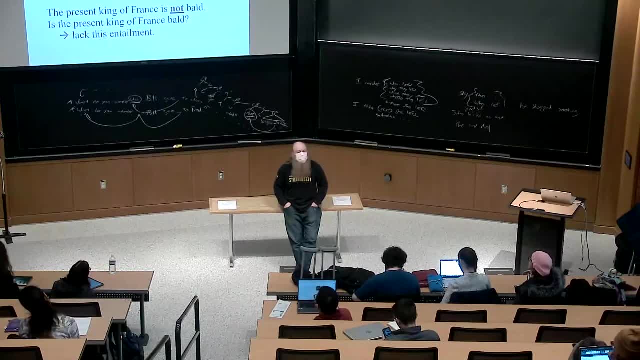 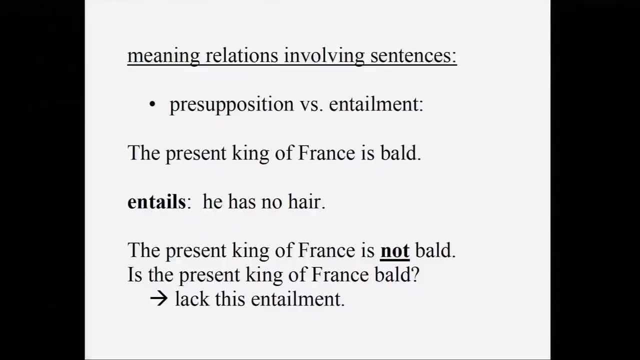 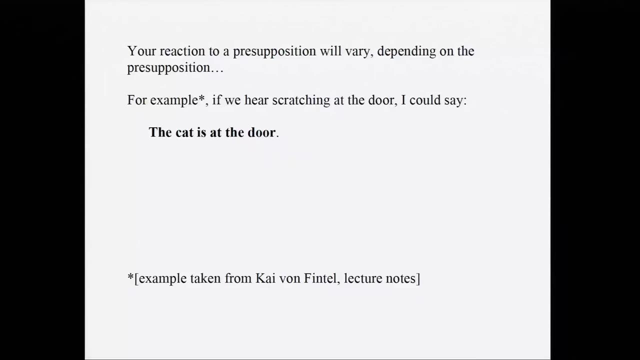 So, yes, uh, that's a case where A entails B, but not A doesn't entail not B. Yeah, Uh, yeah, Yeah, Good Phew. Um, okay, All right, Um, and then presuppositions: yeah, presuppositions. 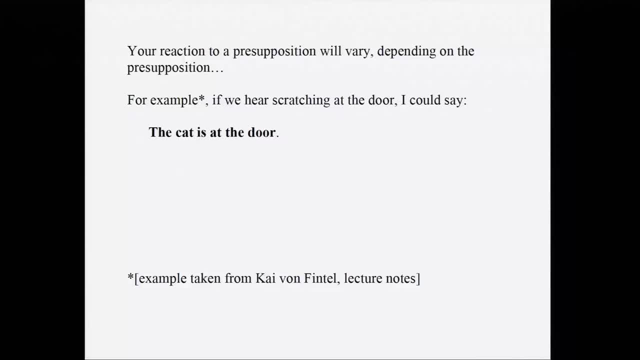 are funny. So, uh, if you know, depending on the presupposition, so if we hear scratching at the door, I could say the cat is at the door, uh, out of the blue, That there's a presupposition there which is that there is a cat. It's kind of like. 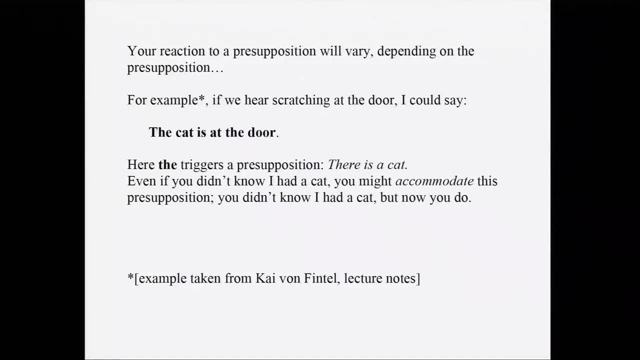 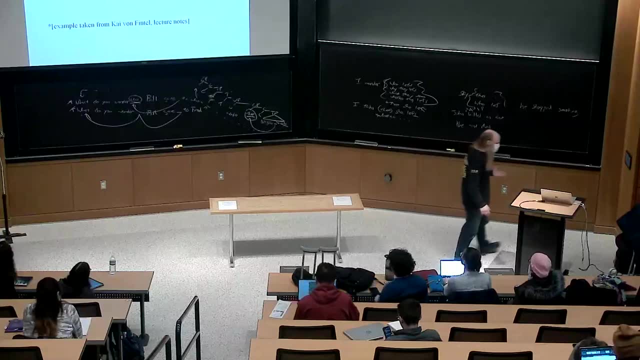 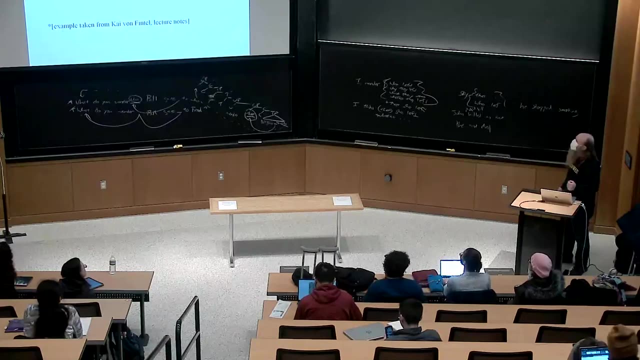 the present king of France is bald, presupposes that there is a king of France. Um, there's a process, what's called accommodating presuppositions, and this is why presuppositions are so handy in comedy and in politics. You make, you say things that presuppose things. uh, and then. 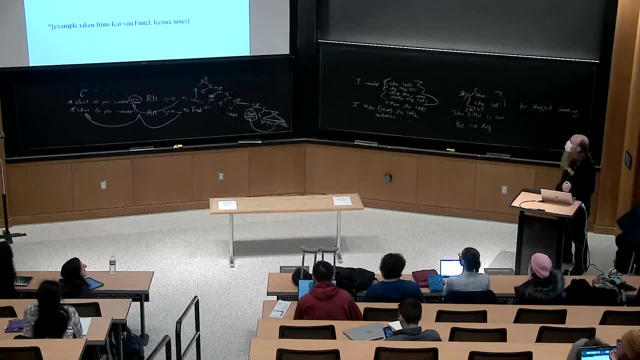 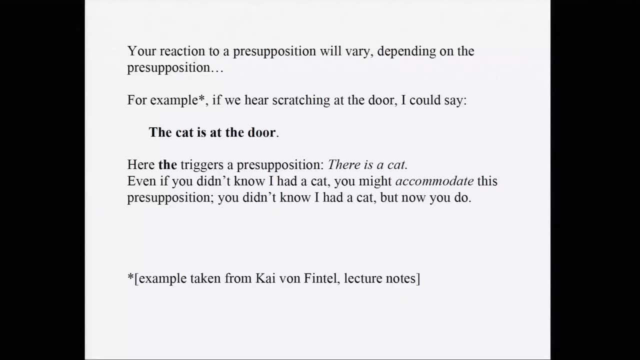 people accommodate your presuppositions, sometimes without realizing it. So if I, out of the blue, say the cat is at the door, uh, you didn't know that. Uh, so uh, if I, out of the blue, know before that I had a cat, I hadn't mentioned a cat before. but uh, my sentence presupposes: 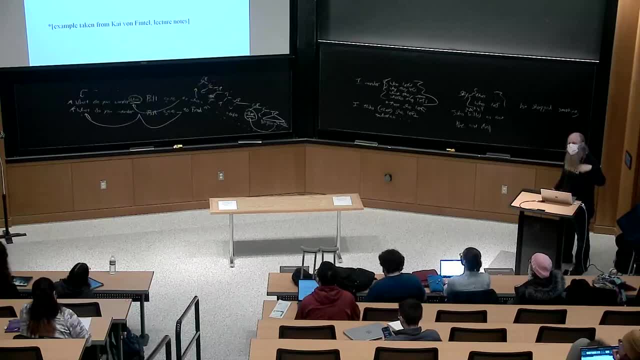 that there is a cat, and so you learn from my sentence that there is a cat and you, you uh, add that to your, to your knowledge base. Um, if I were to instead say the giraffe is at the door, um, you'd probably be less peaceful about it, right? Um, uh, so if, if, 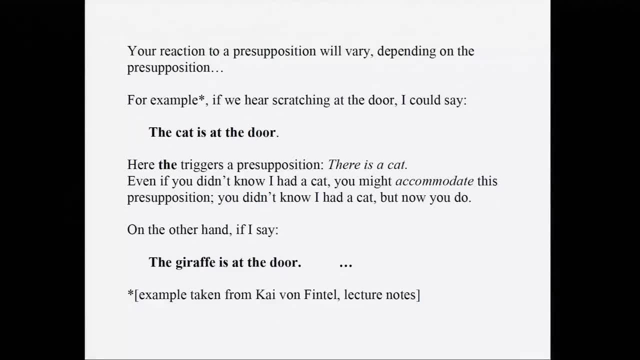 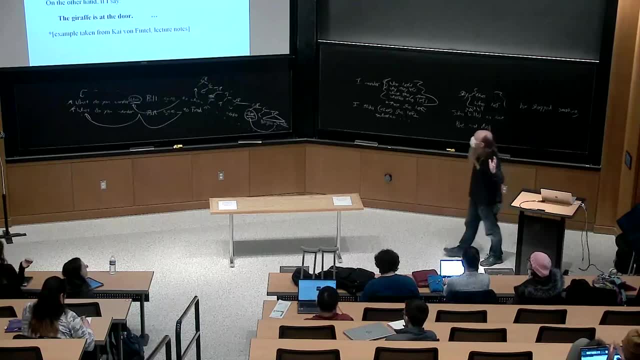 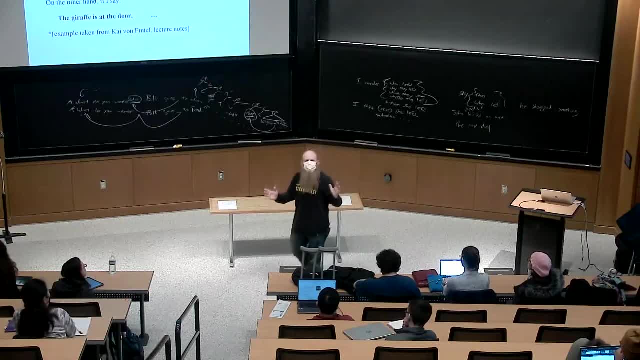 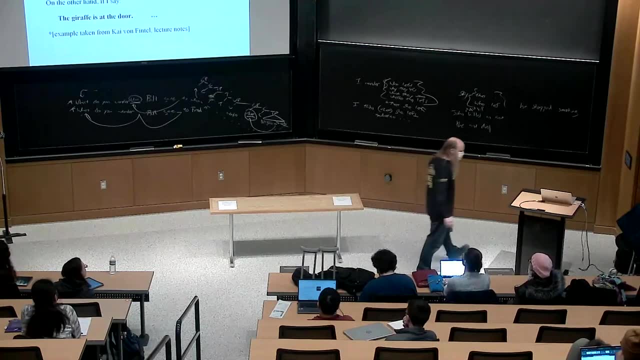 think to yourself, ah, he must have a cat, right? Uh, you know, write down in your mental notebook: he must have a cat. Maybe that's happening on some very fast level, but you're sort of not conscious of it. Uh, on the other hand, if I say the giraffe is at the door, 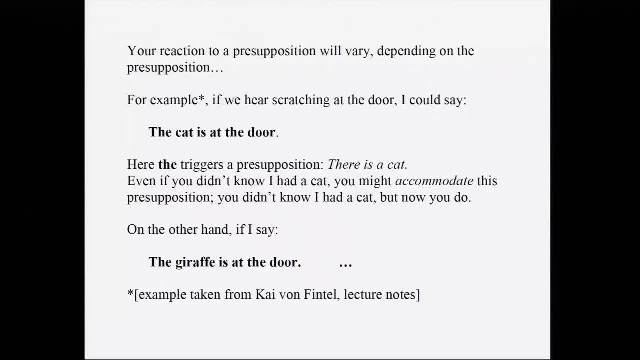 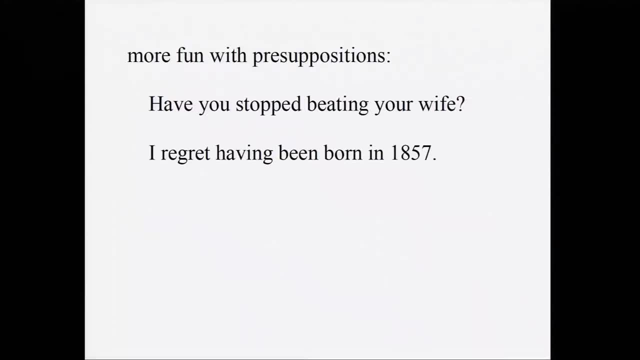 then you, you have the sensation of having learned something significant. Um, yeah, Okay, Right. And similarly, I regret having been born in 1857. If I say that and somebody objects and I say, okay, I don't regret having been born in 1857, uh, either of. 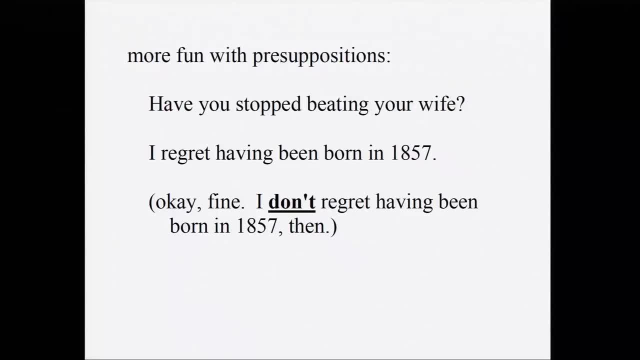 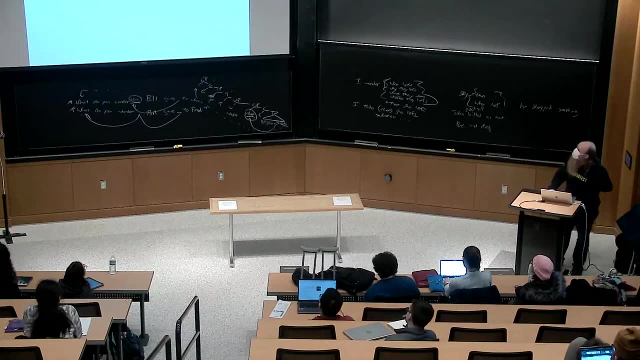 these presupposes that I was born in 1857. Yeah, And uh, uh. in order for somebody to object, they have to say: no wait, surely you were not born in 1857.. Um, so that's entailments, and. 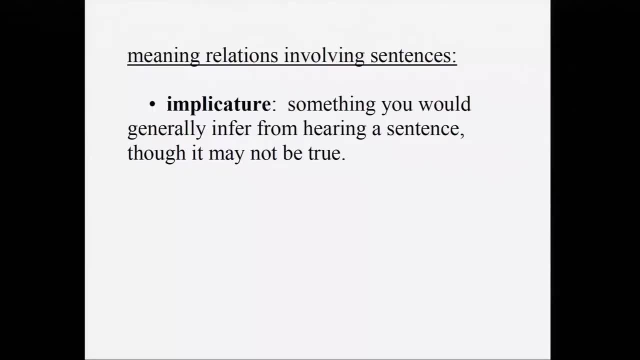 presuppositions. There are also implicatures, which I think we have time for. Implicatures are things that you might tend to infer from hearing a sentence, but that might not be true at all. So, for example, uh, if I ask you a question like can you open the window? 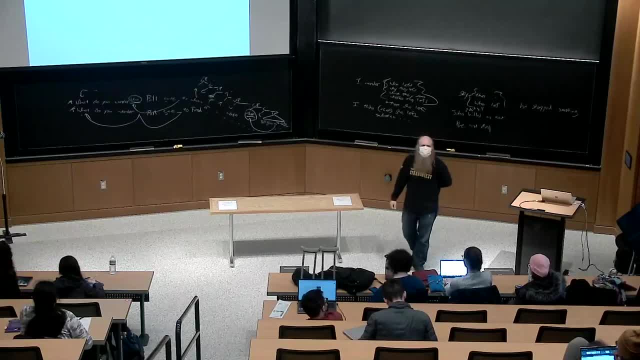 There's an implicature that I would like you to open the window. It's not entailed or presupposed. Yeah, But you, when you hear me say that you're likely to conclude that I wish that you would open the window. Or if I ask you, where's the salt? Yeah, Um. 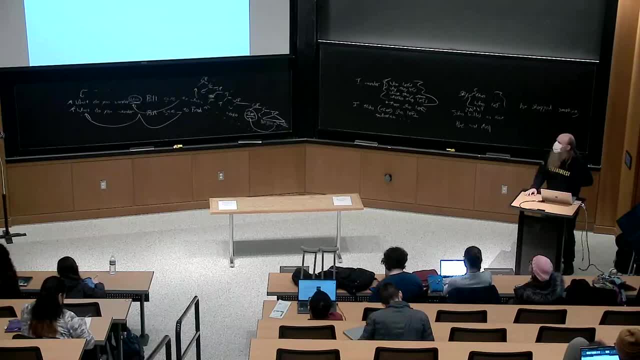 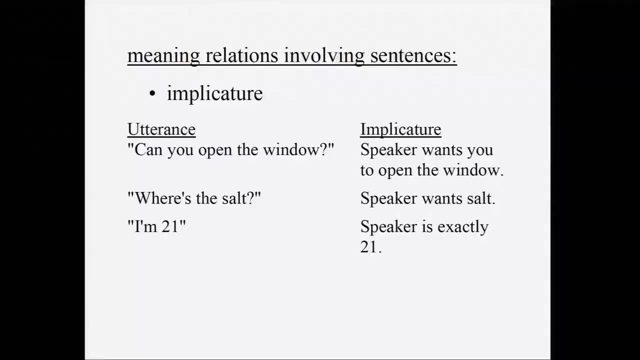 there is a minimally cooperative answer to that in which you point. you know, um, but what I really want you to do is give me some salt, right? Or if I say I am 21,, there is an implicature that I am 21,, that I in fact exactly 21,. 21 is my age, Uh, or if I say: 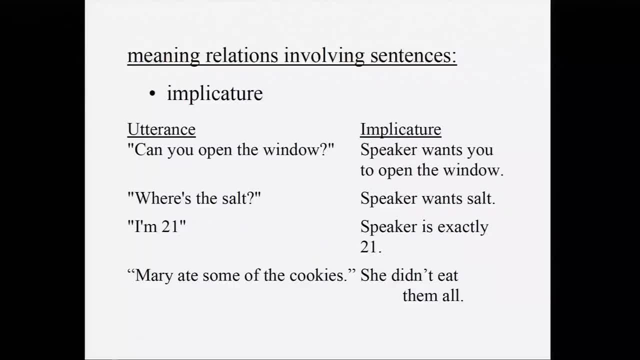 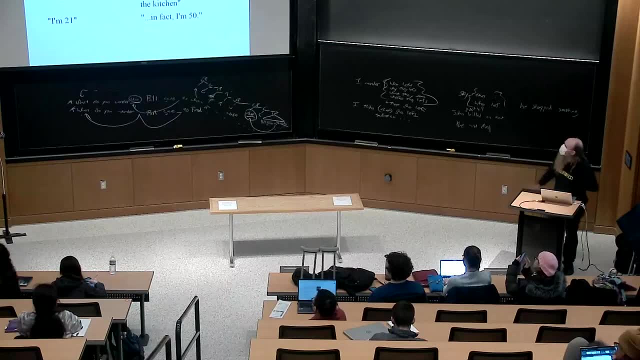 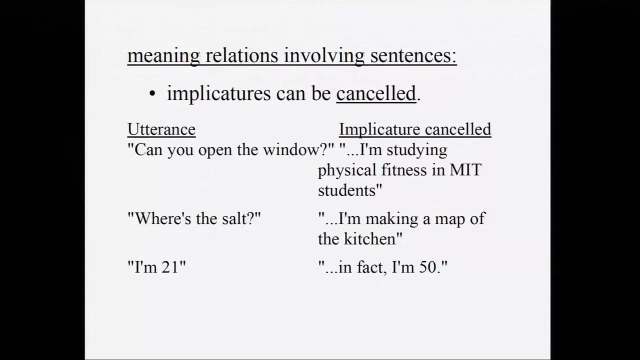 Mary ate some of the cookies, there's an implicature that there are some cookies left, But all of these things could be false under the right circumstances. So, uh, if I ask you, can you open the window? Probably what I in most circumstances. what I want you to do is open the window. 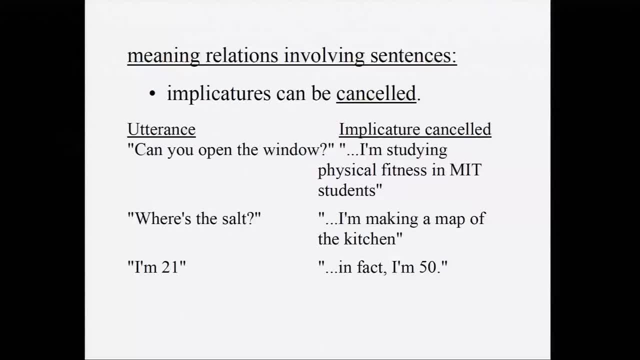 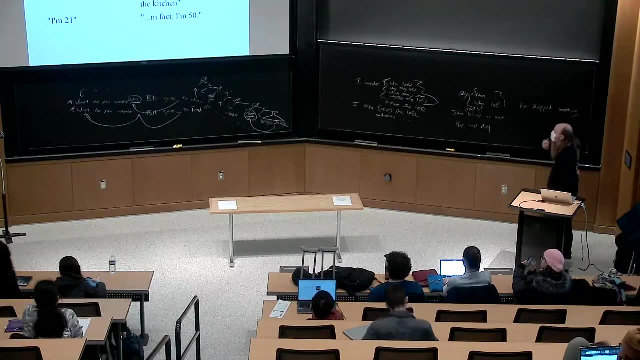 But maybe what I'm doing is, you know, making a study of physical fitness in MIT students, and I want to know whether you're capable of opening the window, Or you know where's the salt- Maybe you. in most circumstances, what I want you to do is hand me the salt, but maybe 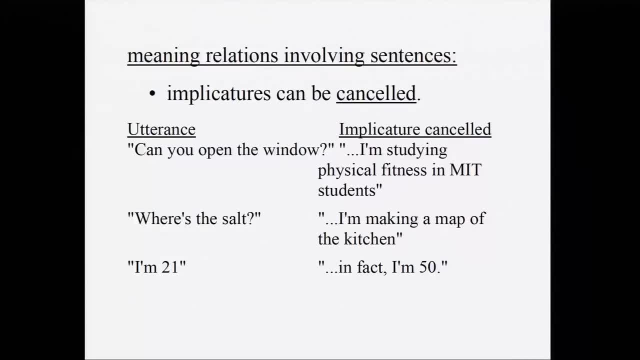 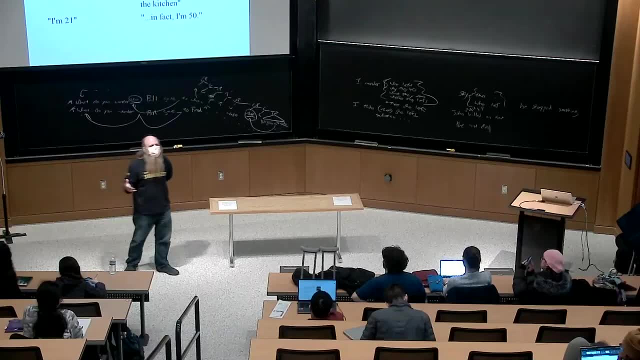 I'm making a map of the kitchen. Or there are circumstances in which I could say- I personally could say I'm 21,- namely when I'm trying to go into a bar or something and, uh, they tell you you can't come in here unless you're 21.. 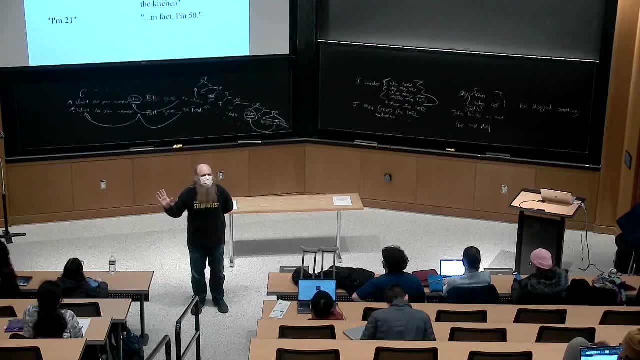 I could say I'm 21.. In fact I'm 50. Yeah, Um, but uh, you know what I mean is I? I satisfy the requirement? Yeah, Do people agree with that? Yeah, There's another kind of example like this: 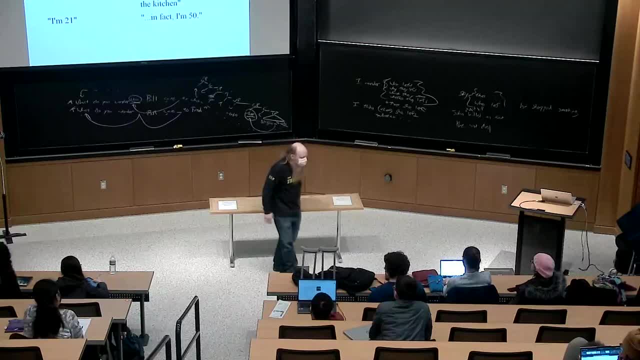 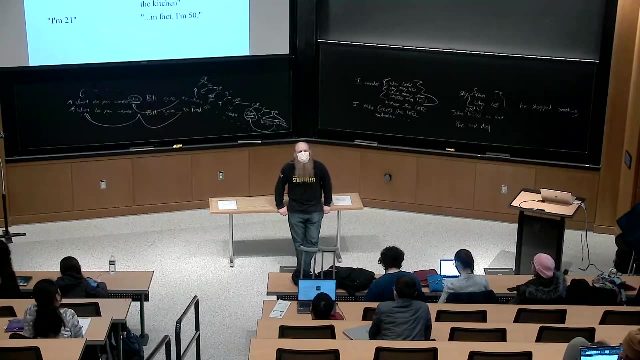 that people give Um. imagine that the government is going to have um a tax break for people with uh, two children, two or more, Yeah, And uh, so, uh, the. I claim this tax benefit on my, on my taxes, and someone from the government comes by. 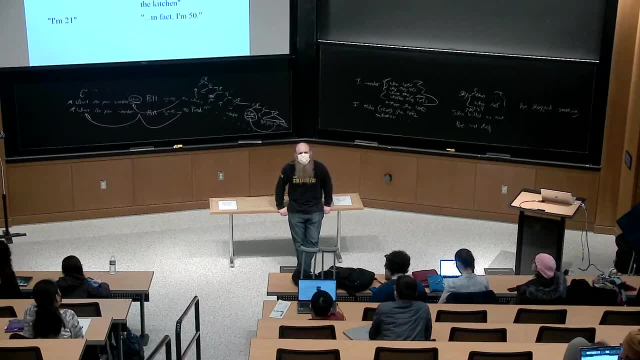 and says: you claimed this benefit. uh, you're claiming to have two children. I say I do have two children. In fact I have six. Yeah, This is um something that people seem to think about numbers: that numbers imply you know exactly the number, but they don't entail exactly the. 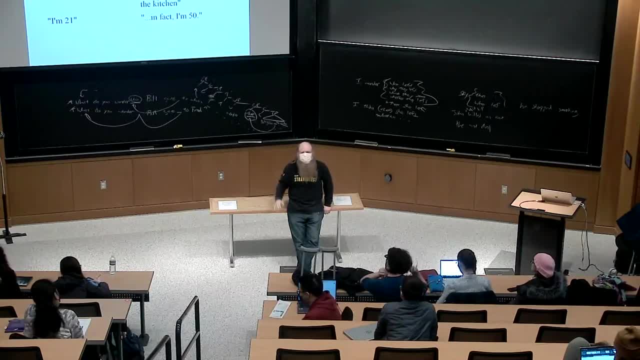 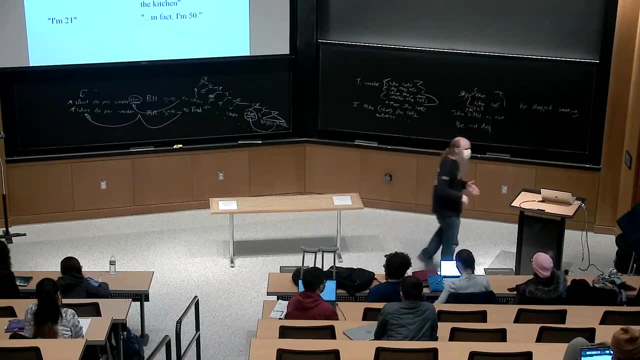 number. They just imply it very strongly, Yeah, And under the right circumstances, uh, you can convince yourself that what they really mean, what they actually entail, is that number or more. Um, these kinds of circumstances lead people to think that. 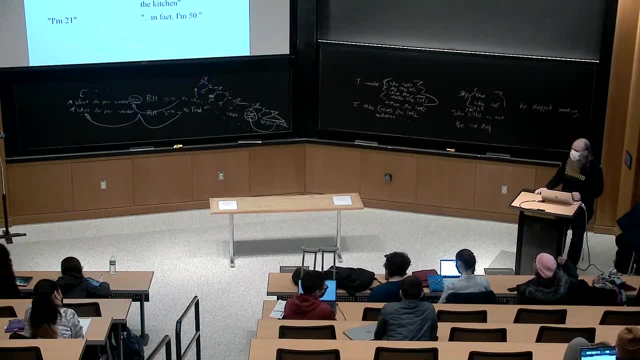 Yeah. I wonder if it's like in in languages where instead of saying things like I am 21,, you say I have 21 years- whether it'd be more likely that you accept like, oh yeah, like if you're 50, you have 50, then you probably have 25.. Uh-huh, Like, like, maybe. 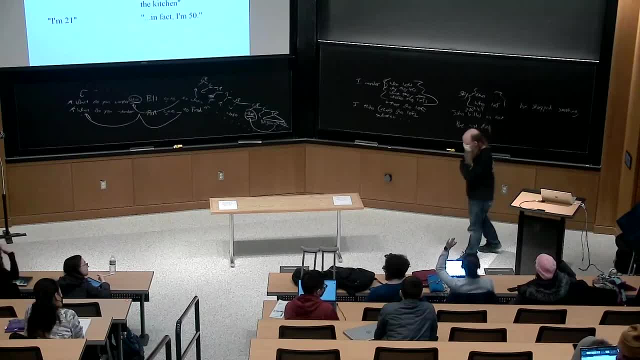 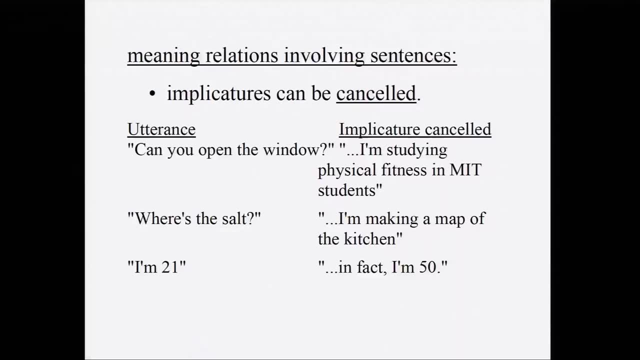 because you think of it as like an identity thing. It'd be interesting to, it'd be interesting to study that. So so, people, when I said that I could say to the guy at the bar, I'm 21.. Yeah, I'm sorry, I'm stepping on what you're, what you're saying, You're absolutely. 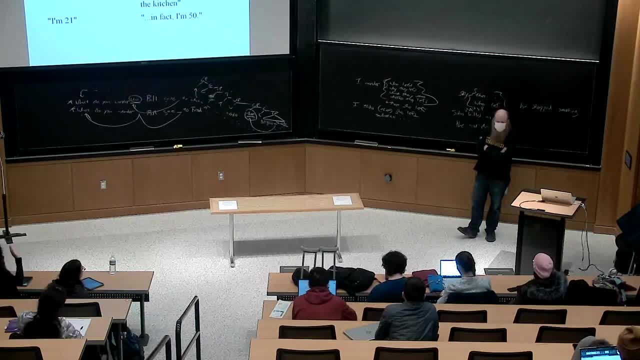 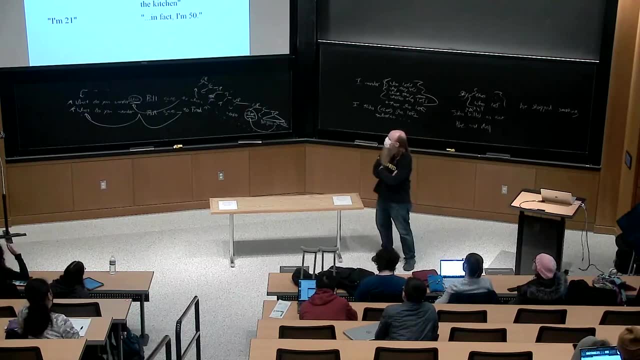 right. There are languages out there, like Spanish, which to say I'm 21,. you say I have 21 years or something like that. Yeah, Um, uh. were people just being polite when I said to the that I could say to the guy at the bar: I'm 21.. Um, did people? people want to object? That would be a. 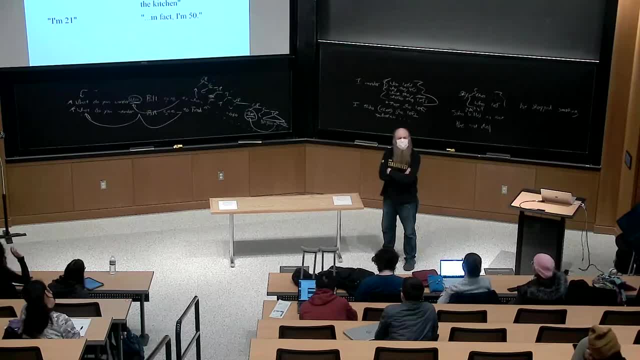 weird thing for me to say. Some people think that would be a weird thing for me to say: What's it? what should I say? I'm 50. Yeah, I was just thinking to say like I'm over 21.. 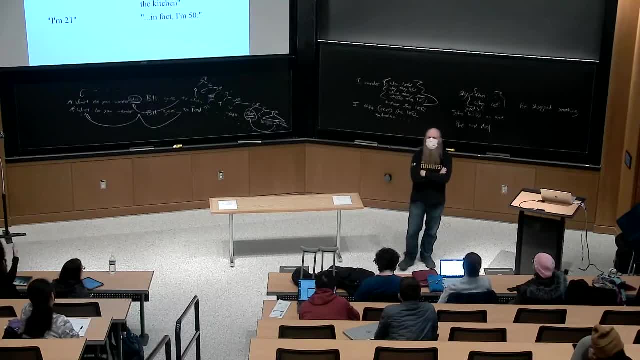 Oh, I'm over 21.. Well, suppose the guy has just said to me: you have to be 21 to get inside. First of all, notice, he can say that, right, He can say you have to be 21 to get inside. He doesn't. 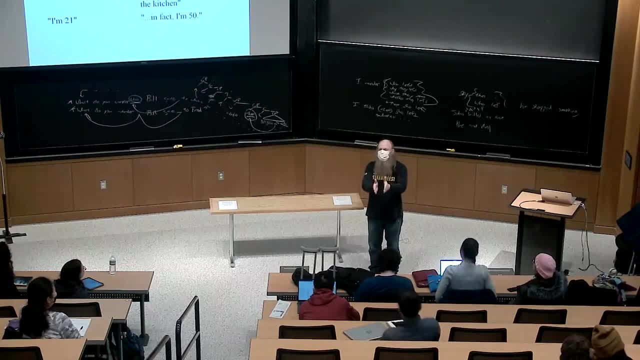 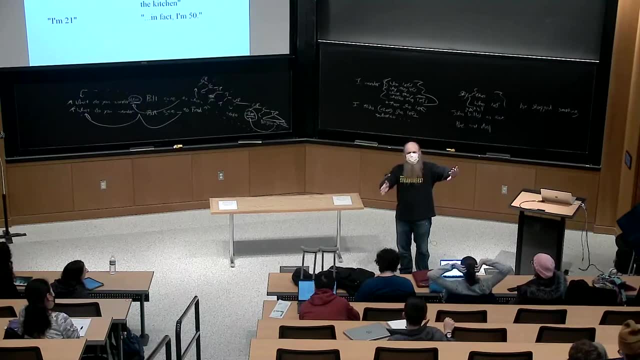 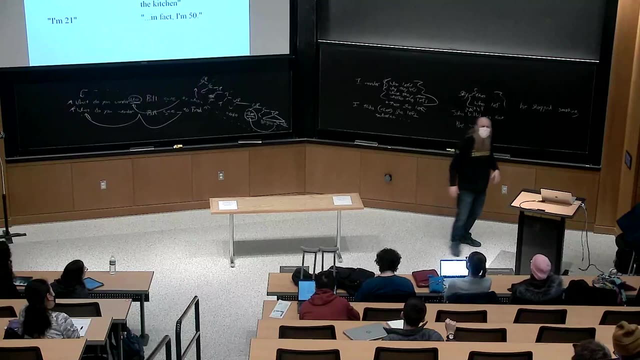 mean we don't allow 22 year olds, right? Um, he means you have to be 21 or higher, you know? And um, what I'm saying is I satisfy your requirement, But I, you know, I, I take your point. All of you go to bars and try this out. No, Oh darn, I've. 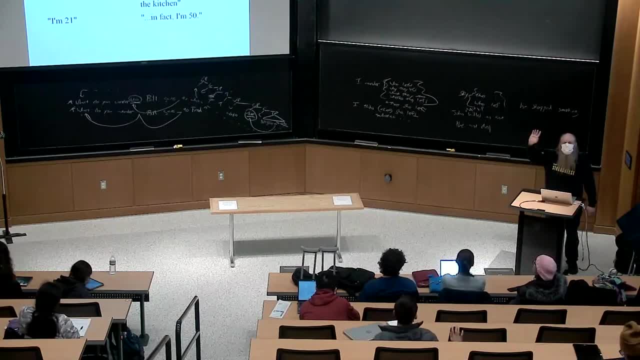 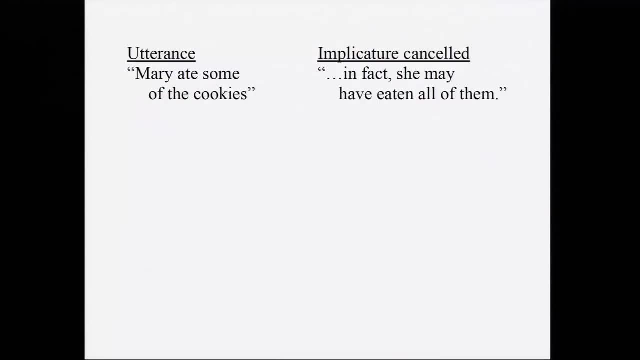 been recorded saying that This is bad. Yeah, Yeah, Okay, Um, oh yeah, And Mary ate some of the cookies. uh, implies that she didn't eat all of them, but maybe she did. Um, okay, So uh. 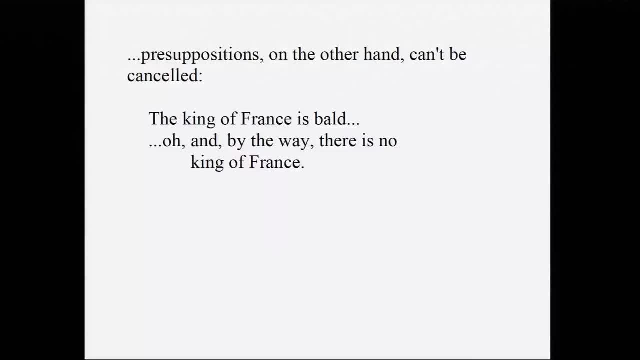 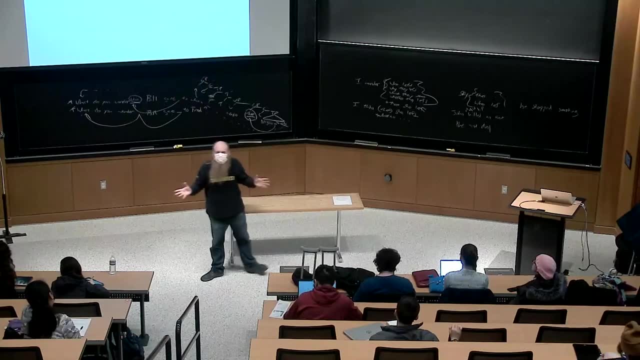 presuppositions are different from this. So, um, I can say things like I'm 21. In fact, I'm 50. or Mary ate some of the cookies. In fact, to be perfectly frank, she ate them all. Um, just so you know. you know, and that's perhaps a slightly. 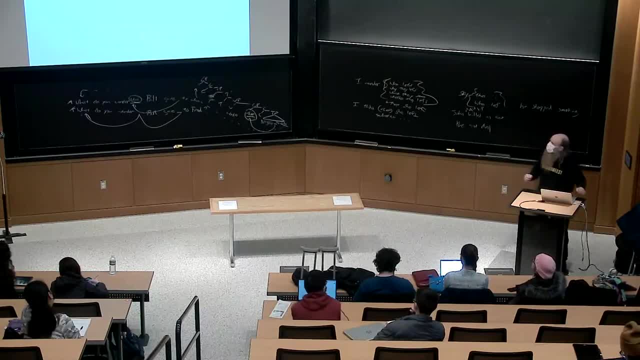 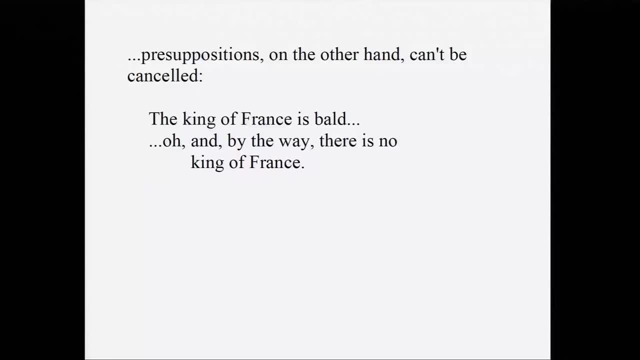 odd way of telling you that, but I can tell you that there's nothing too surprising about it. On the other hand, if I say the King of France is bald- oh, and by the way, there is no King of France- then I am very weird And I know I haven't spent a lifetime researching ways to be very 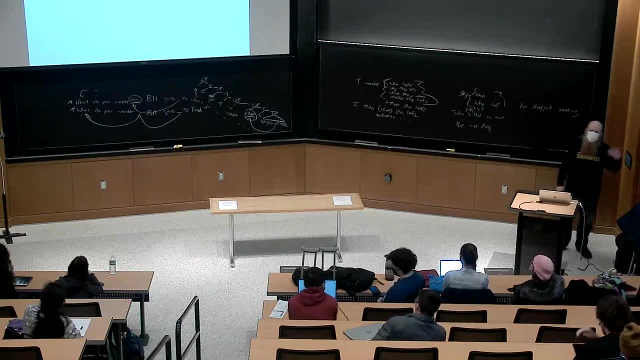 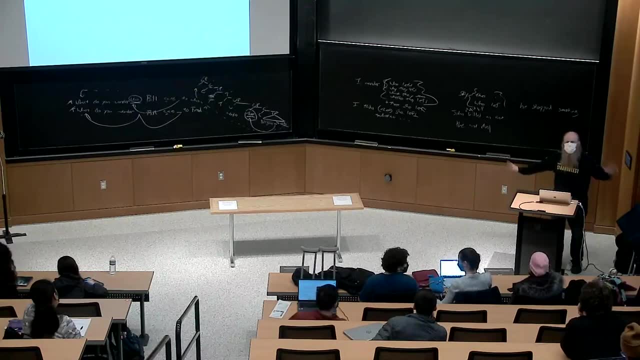 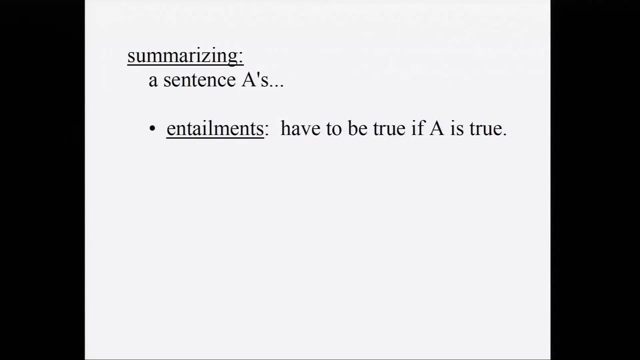 weird. This is one of the best ones, Yeah. So, uh, saying something that presupposes saying a, that presupposes B, and then saying oh and B is false, Uh, that's just like a very peculiar thing to do. So to summarize, uh, we've talked about three kinds of relations between 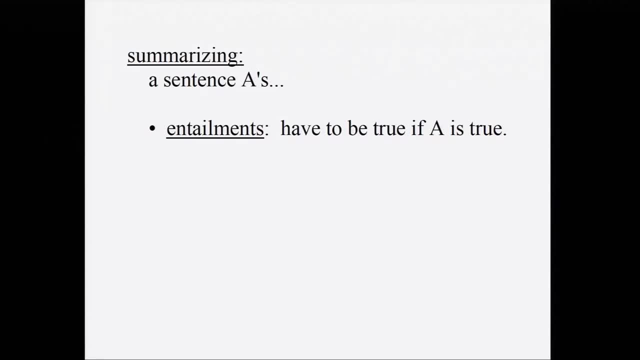 sentences. So a sentence can have entailments. So the entailments of a sentence, a, have to be true. if a is true, Um presuppositions have to be true for a to be either true or false. Yeah, So uh. 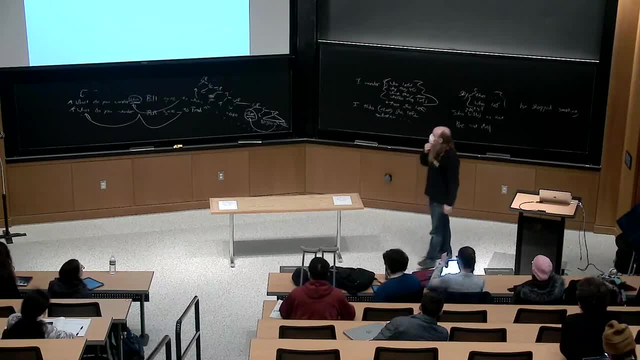 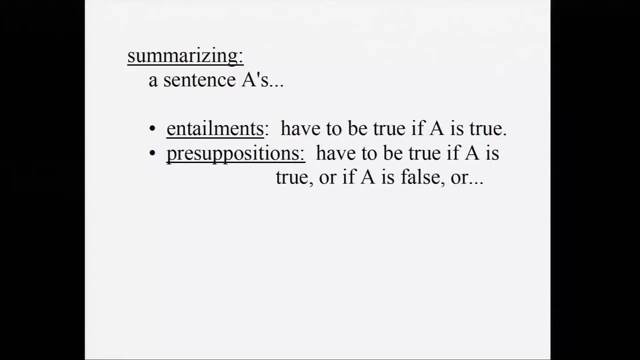 King of France is bald. Uh, presupposes that there is a King of France, So there has to be a King of France for it to be either true or false that the King of France is bald, Yeah, And then implicatures are things that. 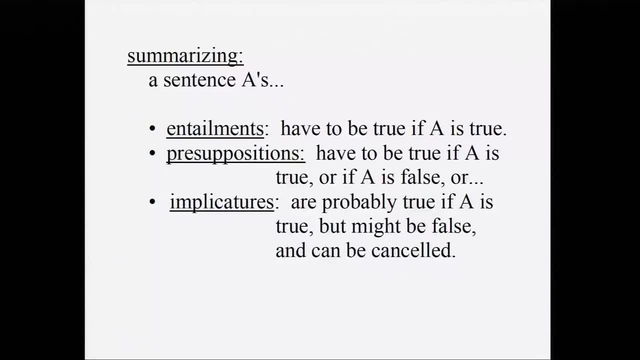 could be true. Uh, you might be inclined to think that they're true. if a is true, but they might be false. And if I, if I say a and then say, oh, and by the way, this implicature is false, uh, you're. 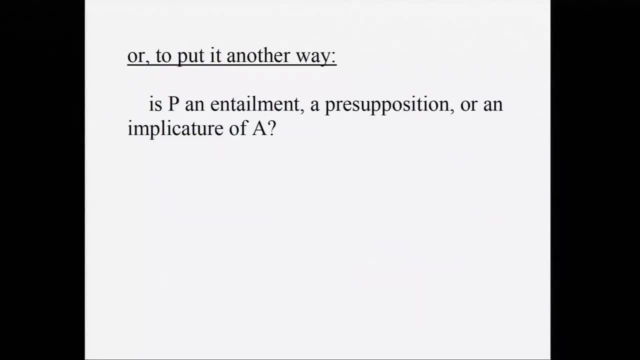 not distraught Um. or to put it another way, if you're asking about one sentence, P, is P an entailment or a presupposition or an implicature of a? the thing to ask yourself is: uh, does P have to be true for a to be either true or false? If so, then it's a presupposition, Um does P have.